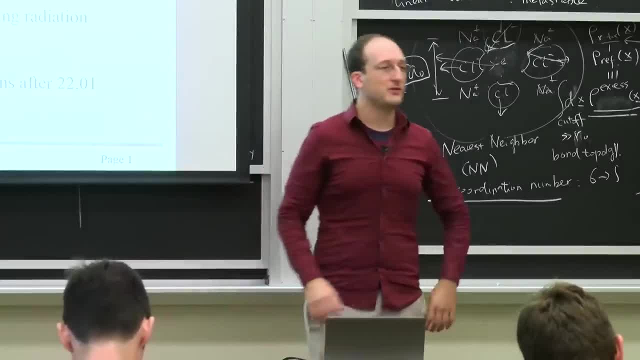 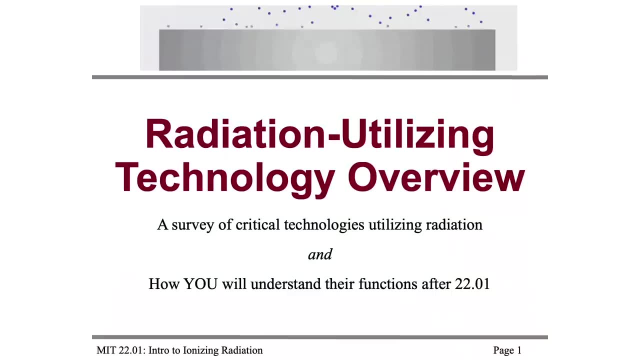 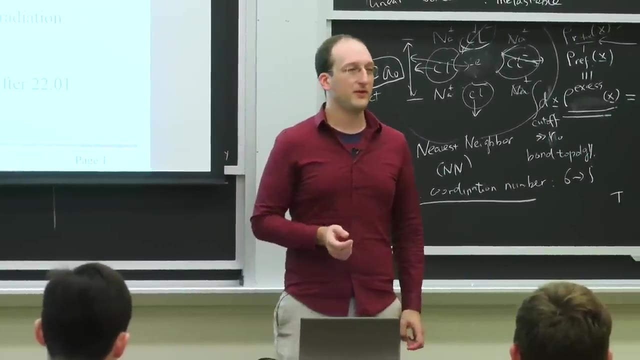 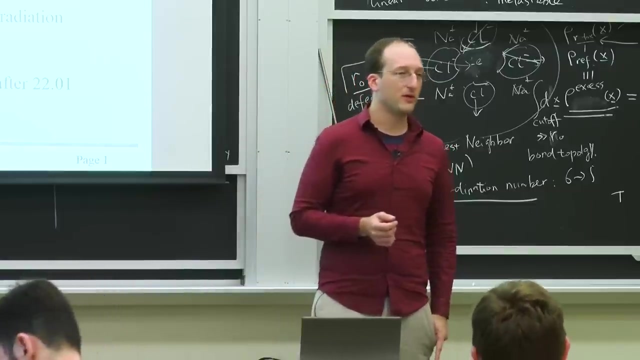 I wanted to give you guys a survey of radiation utilizing technology and tell you a little bit about the way this department has changed the way it teaches. It used to be in our department, and probably everywhere else around the country, that first we teach you the theory of how things go down and understand them and then we can teach you the context in which they're placed. This resulted in a rather boring curriculum, in my opinion, having been one of the ones that went through this actual curriculum. So for those who don't know, I was an 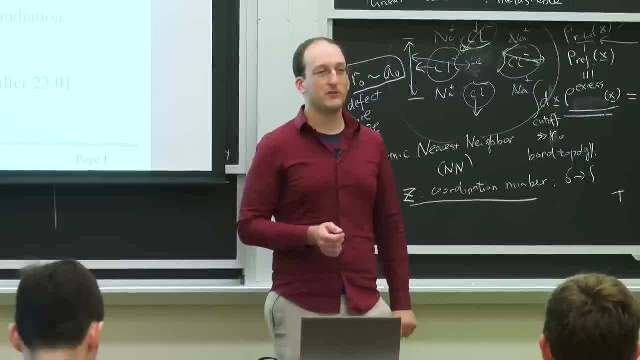 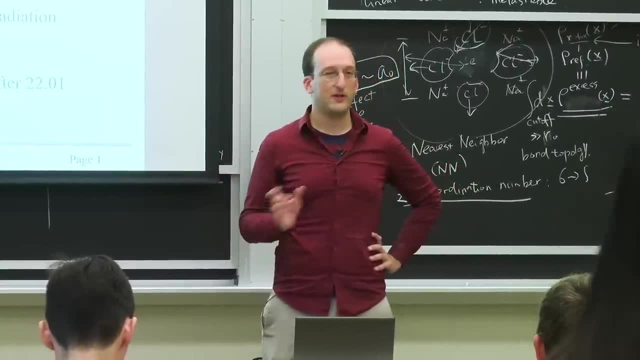 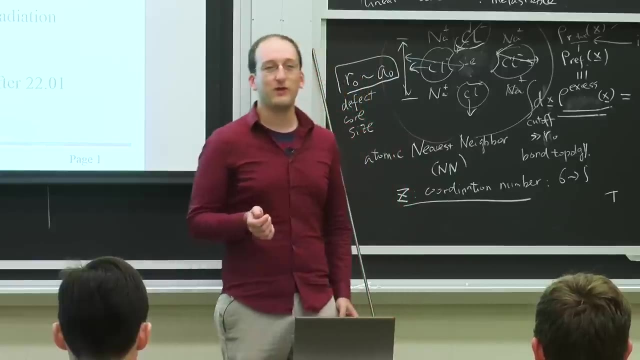 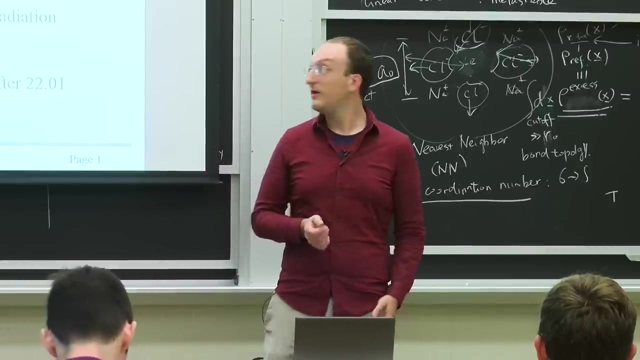 undergrad in this department, And while I learned a lot of great things from folks, I also kept some mental notes on what I would do differently, And now it's the chance to do this. So instead we've adopted a context-first, theory-second approach, which means we tell you where we're going to show you why should you pay attention to the rest of the semester. Then we fill out the rest of the theory, fill in the gaps and then revisit the context to show you what you've learned and how you can understand it. That's why today is going to be a rather light class, so don't take any notes, Just listen, enjoy, ask questions. 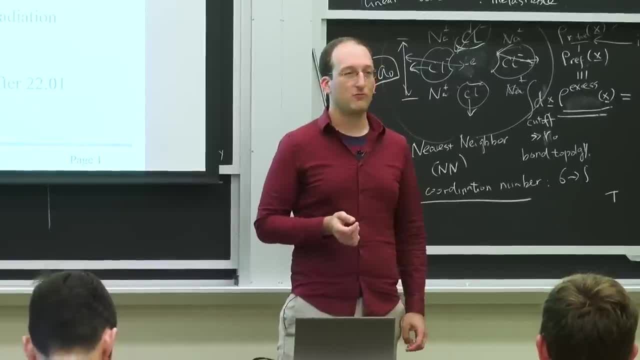 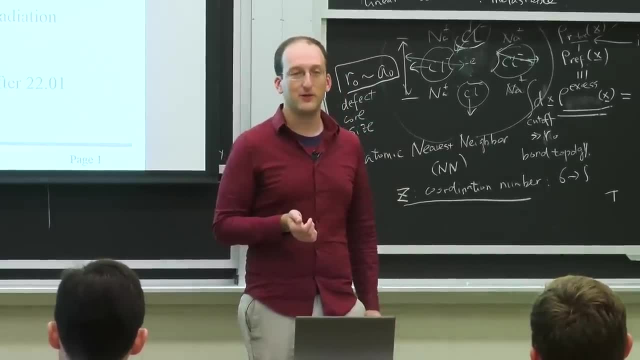 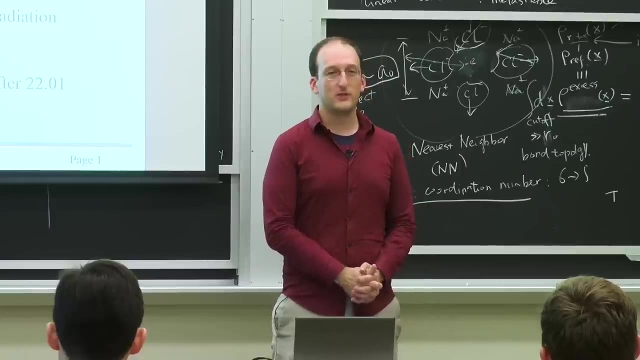 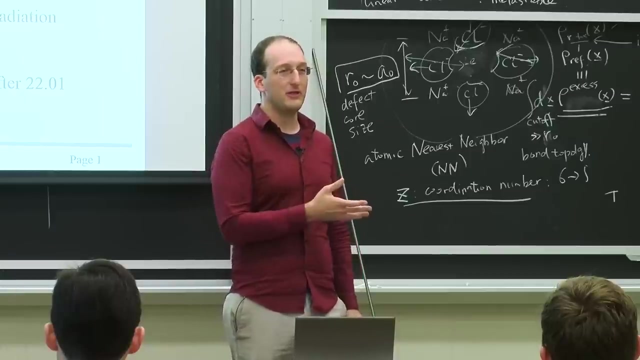 And I'm going to show you some of the applications where we use radiation and the principles of NSE in technology today And for recitation. today, since we haven't gone over any technical material, we're going to be heading to my lab to demonstrate one of these things: a sputter coater, which is a controlled system for radiation damage which applies one material to the other via the process of sputtering or actual nuclear or ionic collisions that blast material- in this case gold- onto whatever you want to coat, which in this case, is a pile of pocket change. 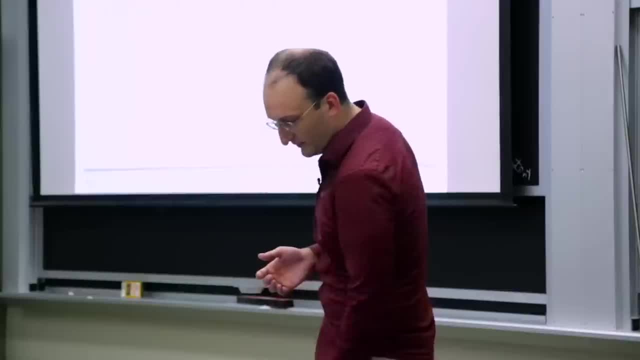 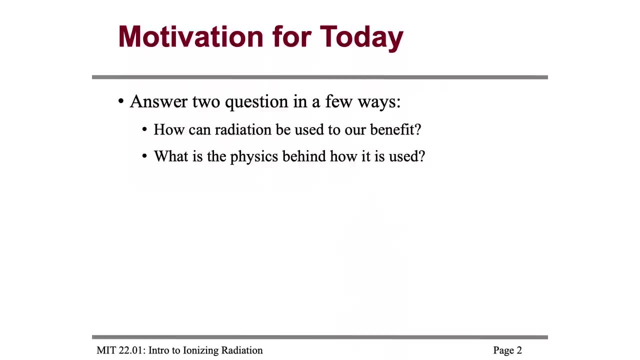 So we're going to make sure that you're all ready. We're going to make some gold change today. So the motivation today is really to get over two questions is: how can radiation be used for benefit and what is the physics behind how it can be used? 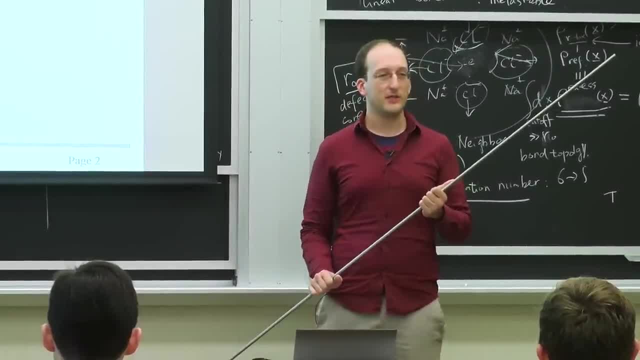 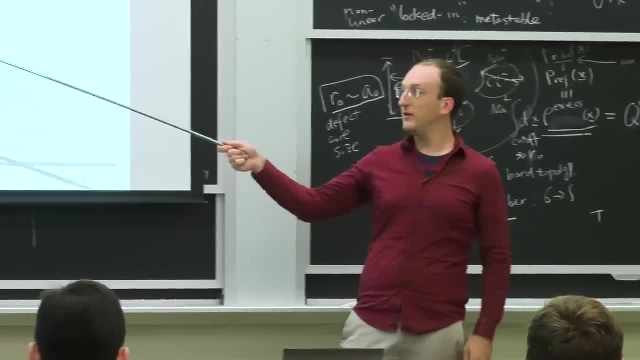 I'll be using a zircaloy fuel rod, the same kinds that you'd see in a nuclear reactor, as the pointer, because I'm not a fan of lasers, And this is actually incredibly light. I can hold it out at the end- not much visible shaking. 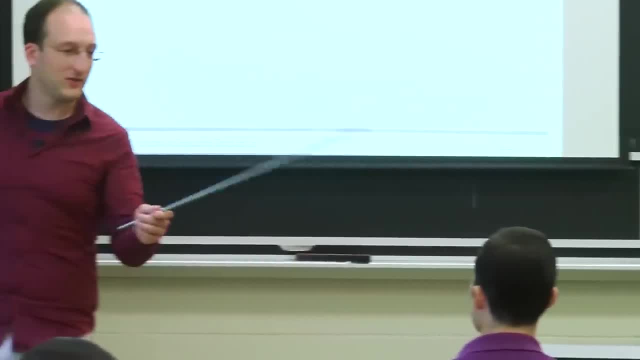 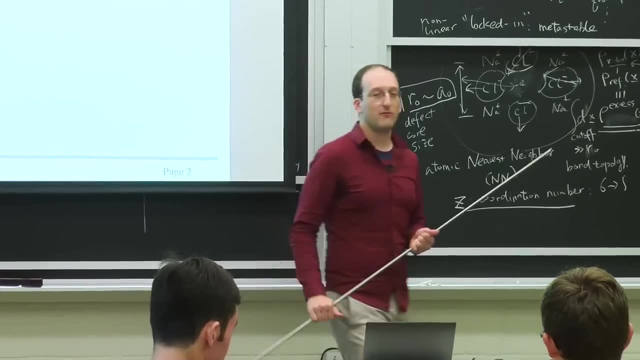 And I wanted you guys to see and feel and try and bend what zircaloy actually is like. That's a piece the same diameter and dimensions and stuff that you would see in a nuclear reactor. So give it a slight bend. If you try really hard you can bend it. 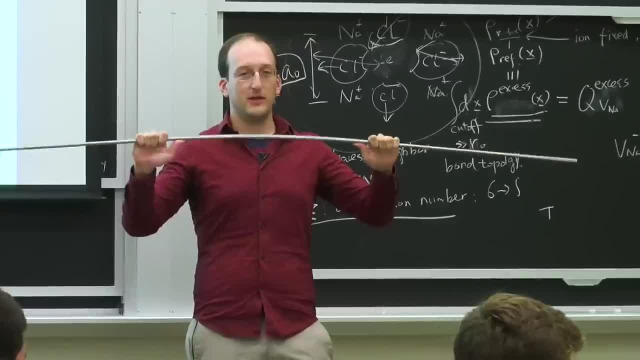 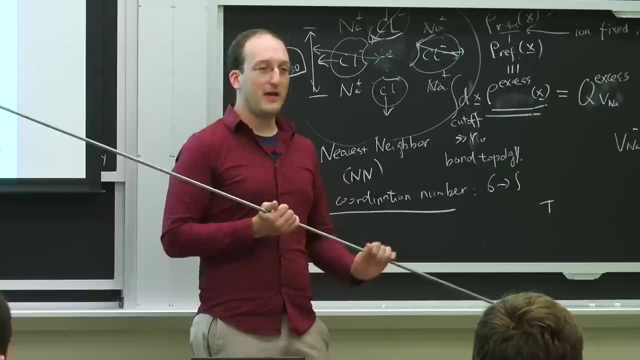 But notice how light it is, Notice how strong it is. It's about midway in density between stainless steel and aluminum, but it's a hell of a lot stronger than aluminum. It also has the added benefit that it basically doesn't absorb neutrons. 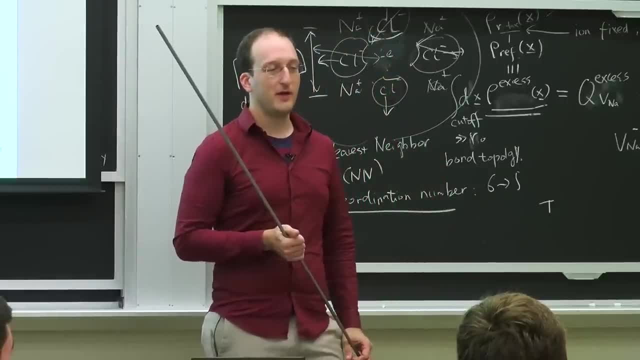 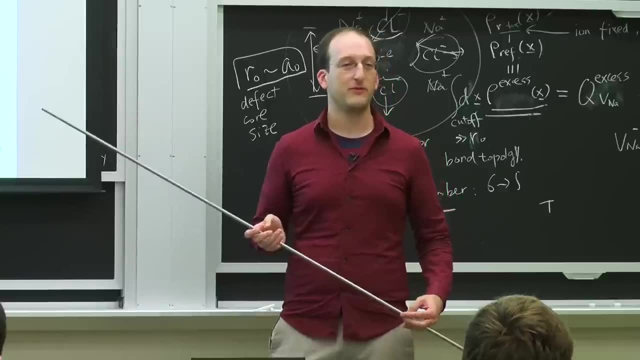 The real reason we use zircaloy or zirconium alloys in reactors is that they have very low interaction probabilities or cross-sections. And for those who don't know what those are, in a couple of weeks we'll be defining what a cross-section is. 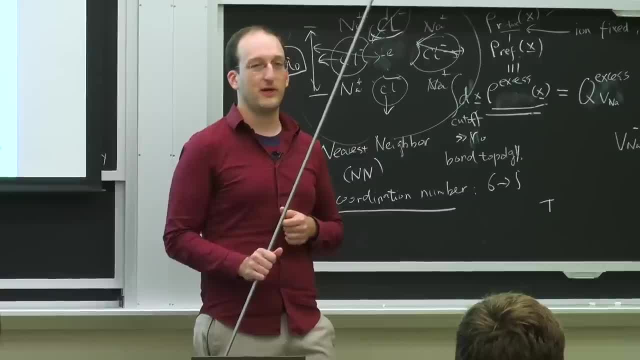 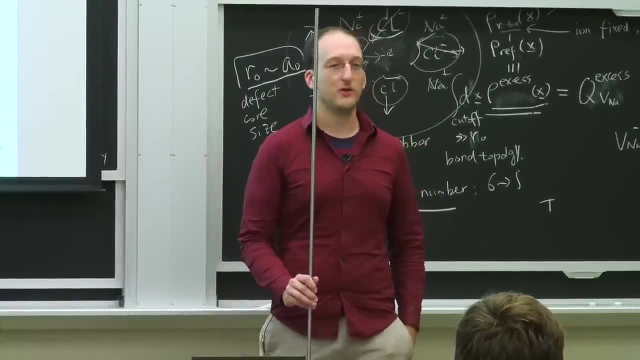 This stuff's pretty cool. Also, what makes this nuclear-grade zircaloy and not just regular zirconium is that there's no hafnium in it. Hafnium is chemically very similar to zirconium. It also happens to be one of the highest cross-section elements. 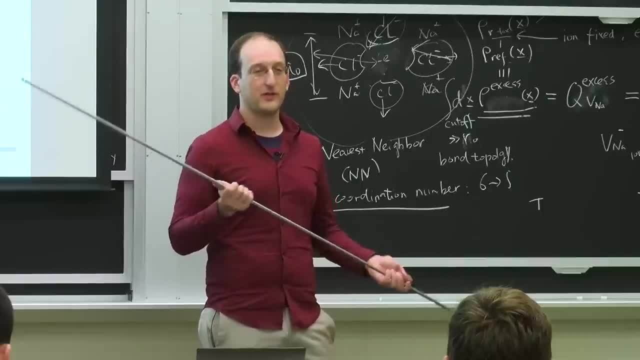 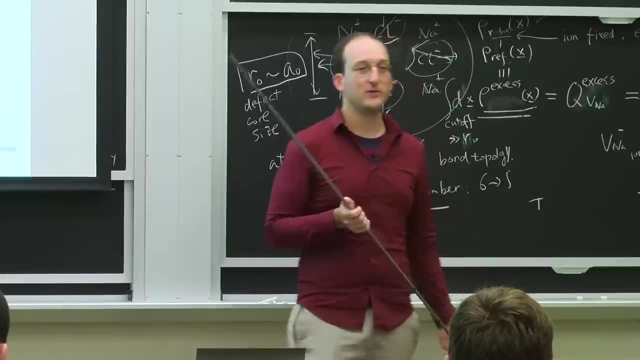 that there is. So you take the stuff that you need to be neutronically transparent in reactors. it happens to be found in the ground. It happens to be found with the last thing you'd want in your fuel cladding. In fact, you can use hafnium as a control rod or control blade. So the difference in chemistry and in cost between nuclear zirconium- what you've got there- and regular zirconium is the hafnium has been taken out by some very painful chemical separation. Usually you'd find about 3% or 4% hafnium. 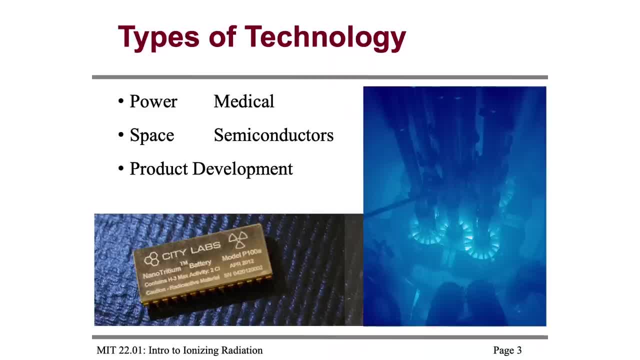 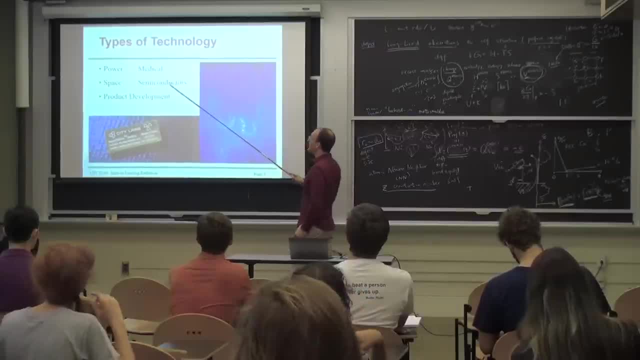 So there's all sorts of technologies that we use. the principles of nuclear science and engineering- I'm just going to say NSE from now on. You're all probably pretty familiar with power and maybe familiar with some of these other ones, like medical isotopes are the backbone of a lot of imaging. 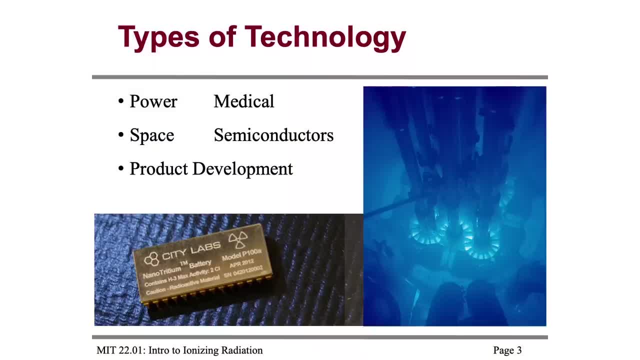 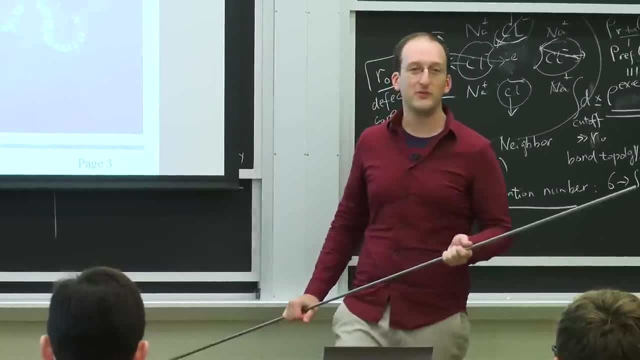 techniques to find and treat different maladies. Space is basically a giant maelstrom of radiation so you can both use it and have to shield from it. We'll go over some of the crazier ways of shielding from space radiation actually today. 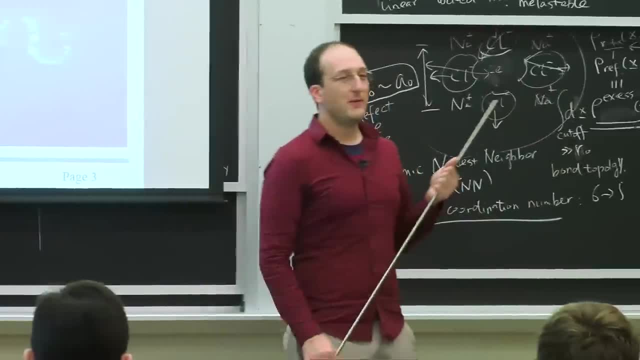 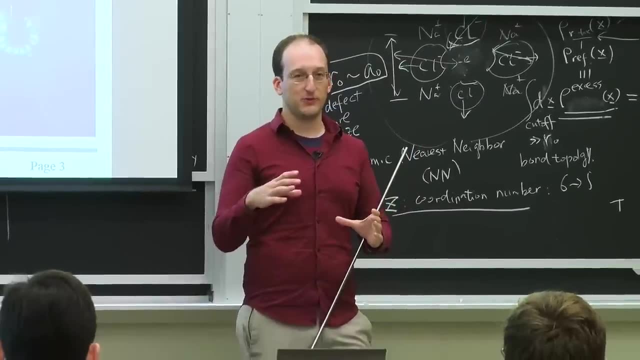 Semiconductors. the way that the MIT reactor made about 60% of its operating budget until recently was by irradiating crystals of silicon, single crystal boules or ingots of silicon to make what's called an N-type semiconductor via the following reaction: 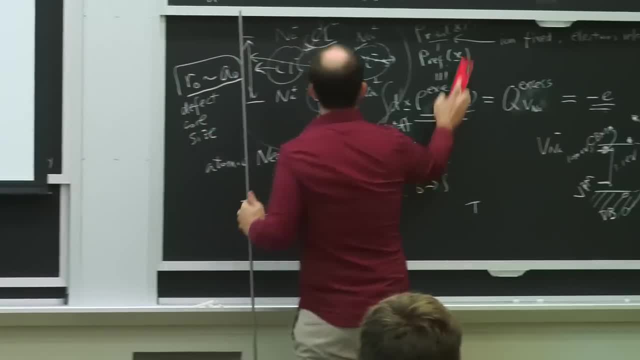 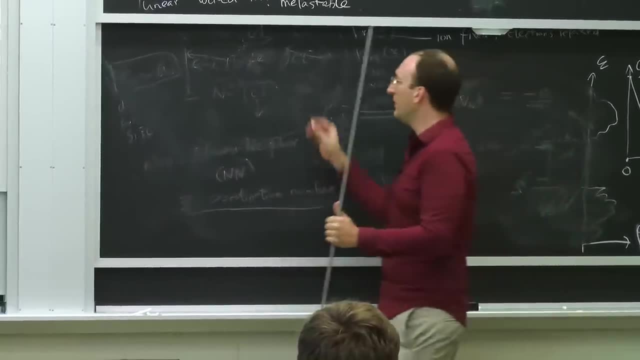 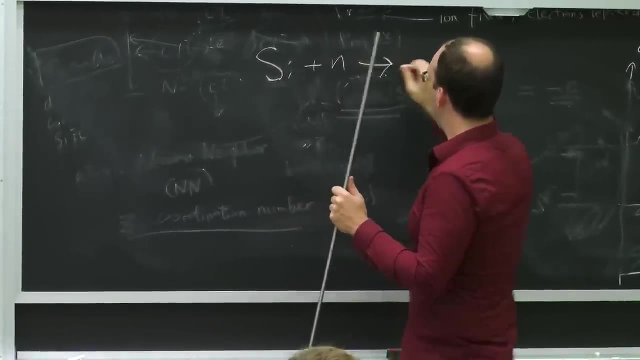 if I can find an eraser, I'm going to use the shorthand that we talked about last time. Normally, you would take silicon and you add a neutron and you end up forming phosphorus. I've not memorized the masses of the isotopes, but in the end 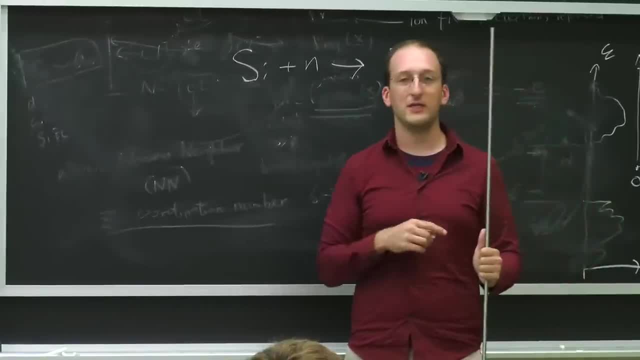 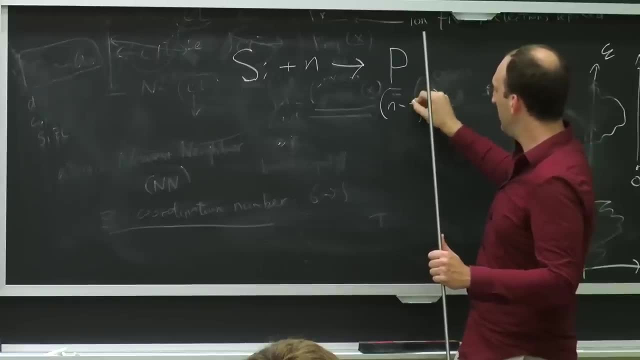 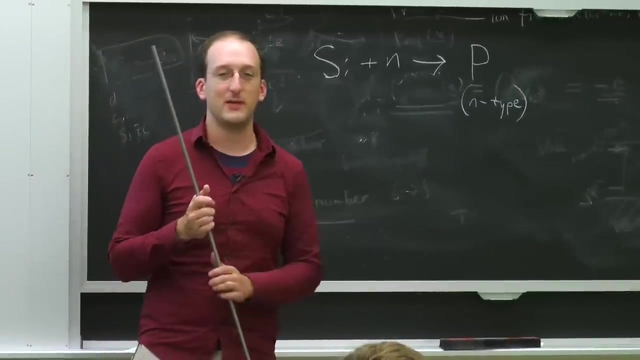 this is actually a neutron capture reaction and then a resulting decay which produces phosphorus, which is what's also known as an N-type dopant. It's a sort of extra negative charge-type dopant that changes the conductivity of the semiconductor. 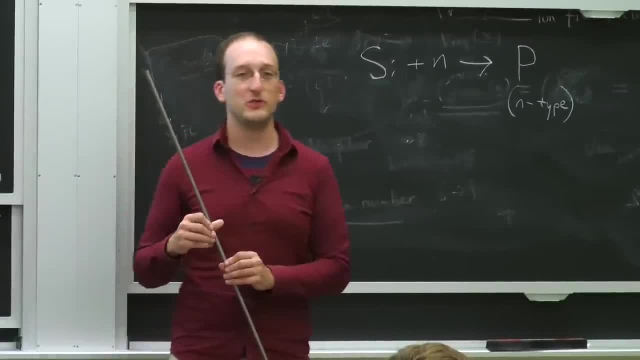 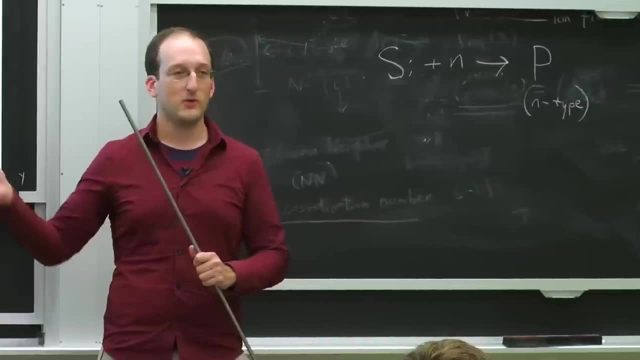 There's lots of different ways of doping semiconductors. One of the best and most uniform is to stick things in the reactor. So back when silicon ingots were smaller, like four or six inches in diameter, there was a constant a train of these things traveling. 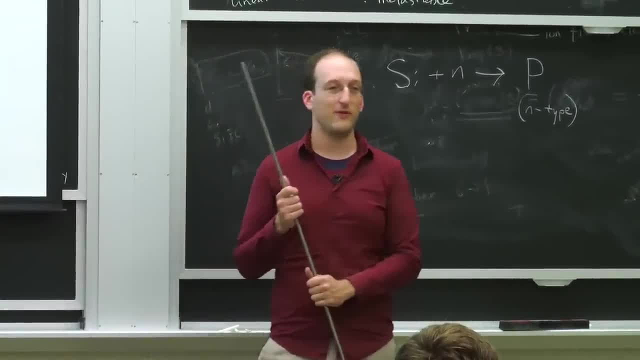 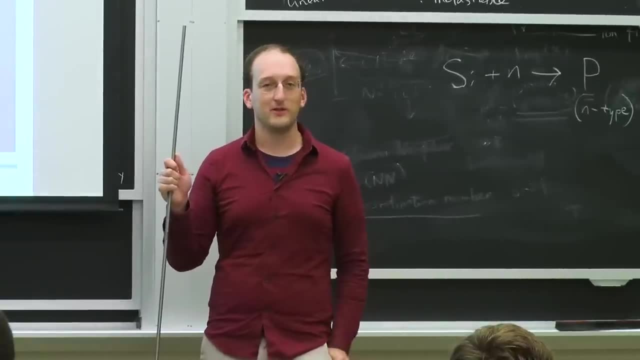 through the reactor, getting irradiated and being sold and then cut up into wafers to make devices. And it used to be student or UROP jobs to load and unload those things from the reactor. Now it's not that dangerous. 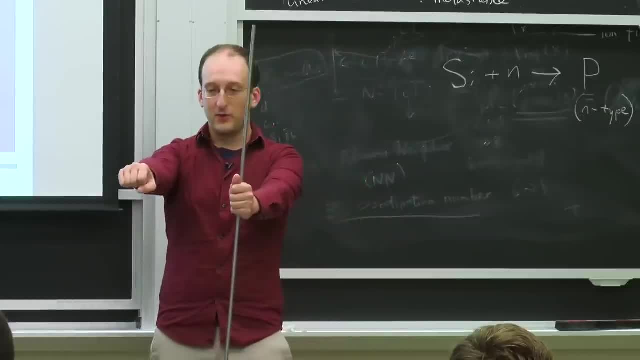 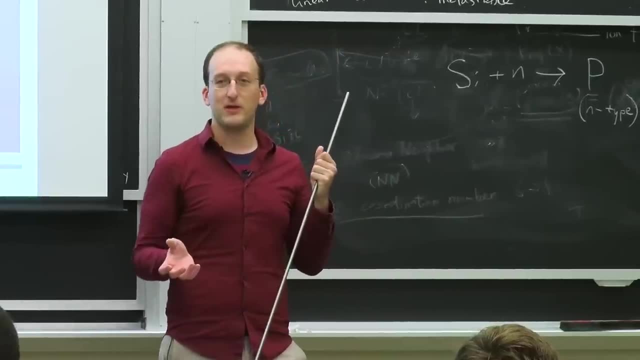 As long as you use the right handling procedures, like put them on a cart, pull the cart at arm's length and push, like that, your dose is very low. And that's because for a given point source emitter, the dose you receive drops off as 1 over r. 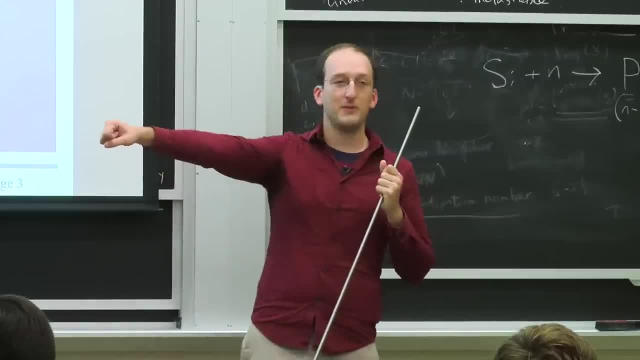 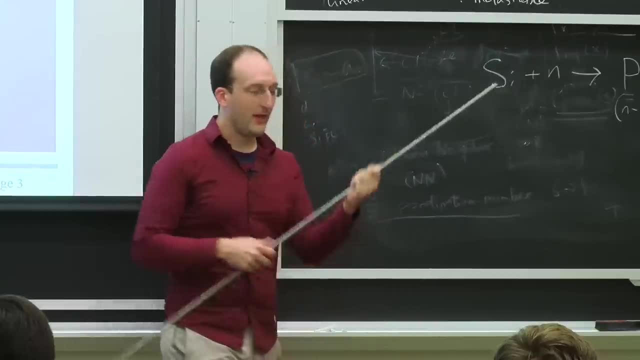 of the distance squared, which means that your arm's length, let's say your arm- is about a meter- you can drop the dose by quite a bit compared to what's called the contact dose. Well, this poor fool held the silicon ingots. 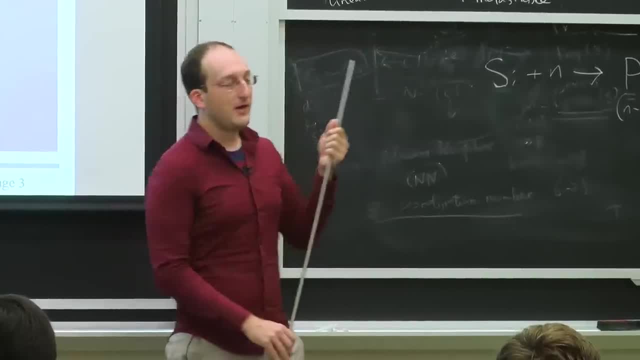 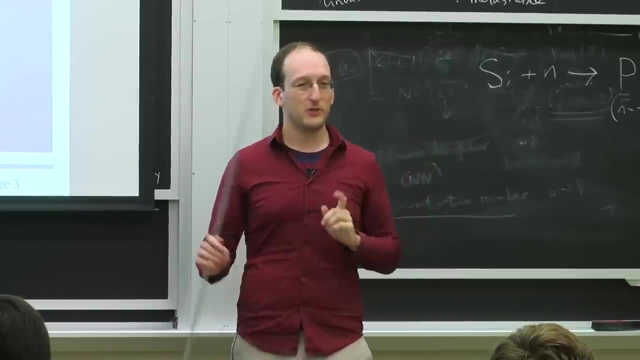 up to their chest like that. They were OK. They got about 10 months of their yearly allowable radiation dose that won't induce any additional risk of cancer. But to ensure that they would not exceed that allowable dose they became the administrative assistant for the reactor for the next 10. 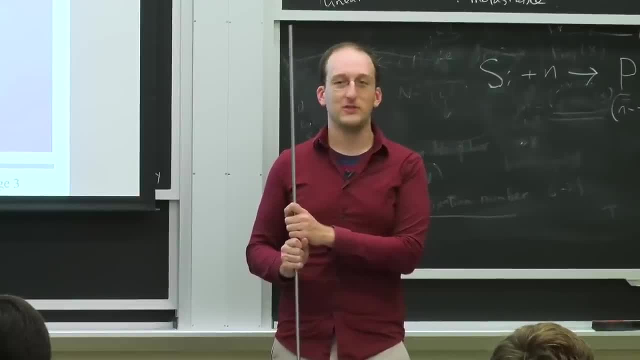 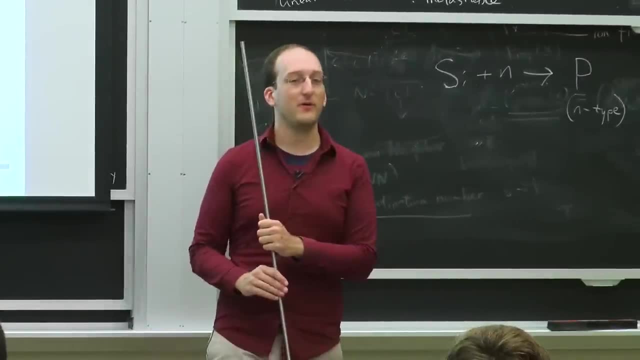 months. So their job at the reactor was to answer the phone, which is not a radioactive activity, including at the reactor First nuclear power. The reason why I know a number of you guys are here is pretty simple: It's just a hot bucket of water. 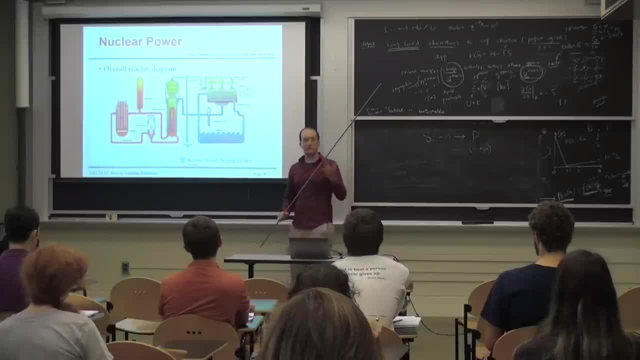 The way we make that bucket of water hot is by putting uranium or other fuel into these rods, assembling a lot of them in a small space, where they then heat up by producing nuclear fission, capturing the resultant kinetic energy of the fission products. 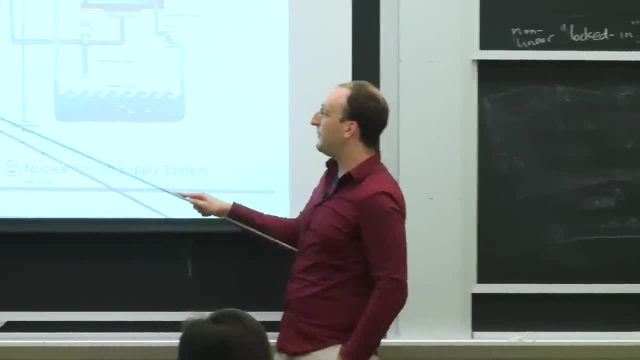 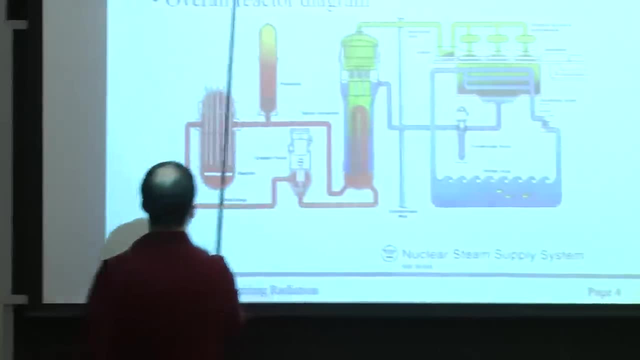 and neutrons and everything else that comes out, and using it to either heat up or boil water That's then just driven through a heat exchanger and a turbine. So, aside from everything on this side, it looks basically like any other water-cooled power plant. 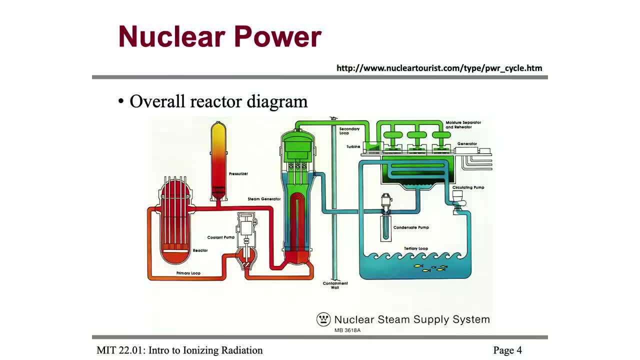 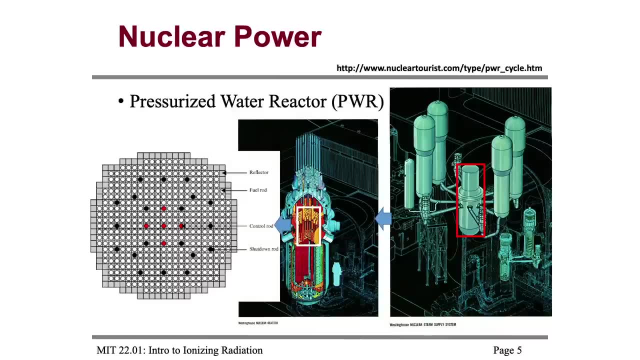 The difference is things get toasty in a radioactive sense, but also pretty well under control. And what's inside a reactor? if you say, this is the diagram of a typical pressurized water reactor or PWR, where the water is pressurized enough so as 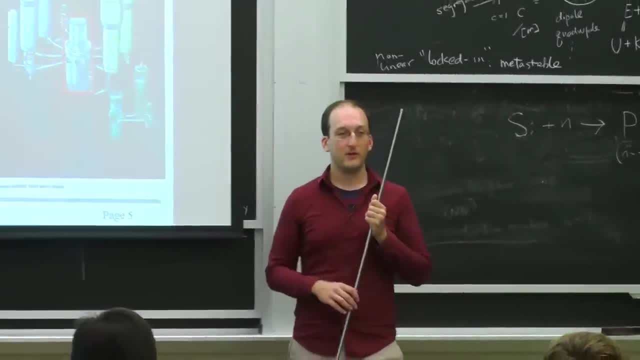 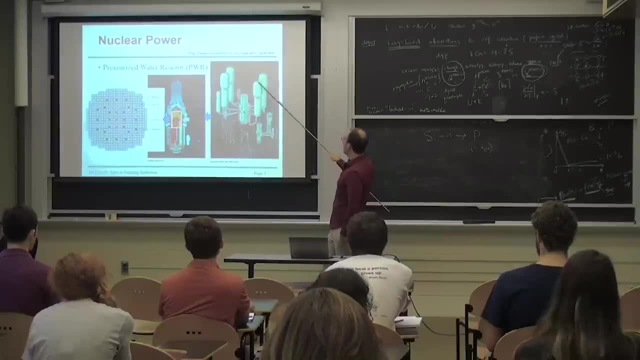 to stop boiling from occurring, keeping the water liquid, which has a number of safety implications. You've got the core of the reactor right here, And these things right here are called steam generators. It's nothing more than a heat exchanger that generates steam. 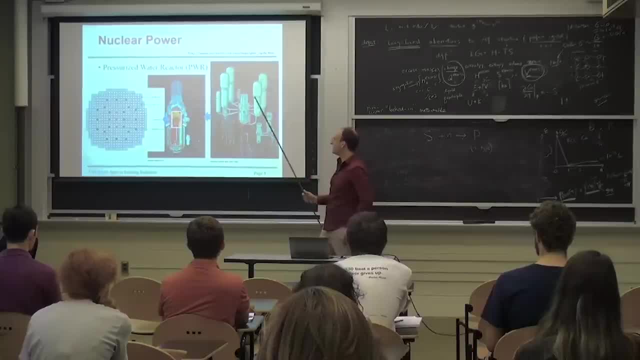 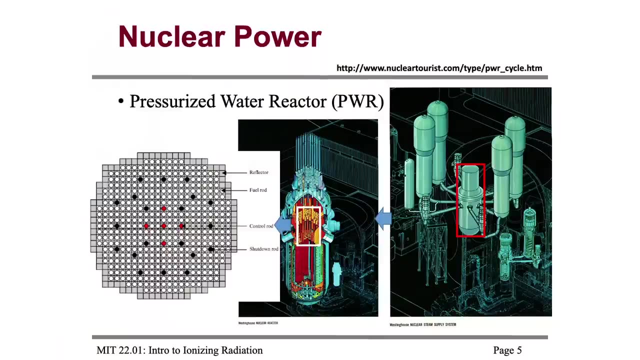 And the steam generated in here goes off somewhere else and drives the turbine. If you look inside this reactor, you'll notice a lot of different fuel assemblies or fuel rods, including things like control rods or shutdown rods- rods made of neutron absorbers, like hafnium that we talked. 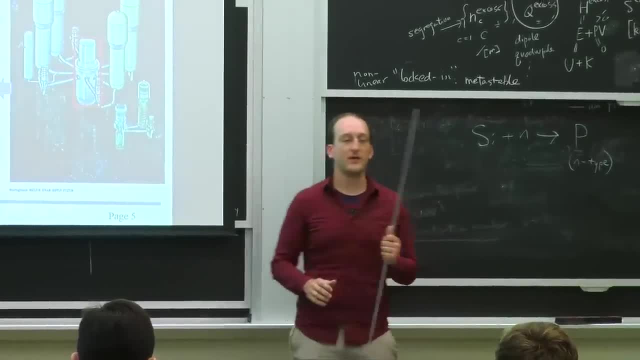 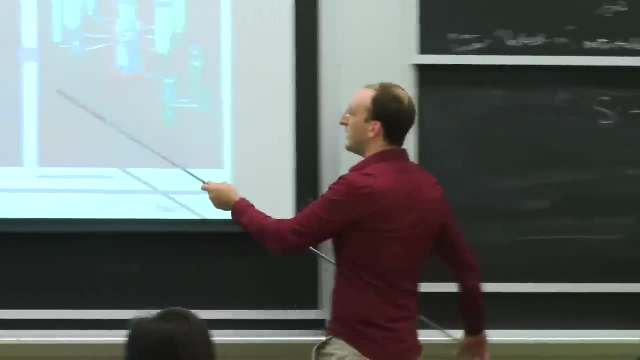 about Or gadolinium or boron 4 carbide or any other material with a high capture cross-section, meaning a high probability for capturing a neutron, rather than letting it go from one fuel element to another. to produce more fission, to produce more heat. 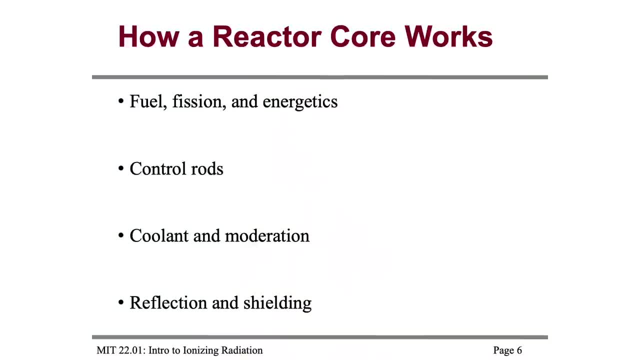 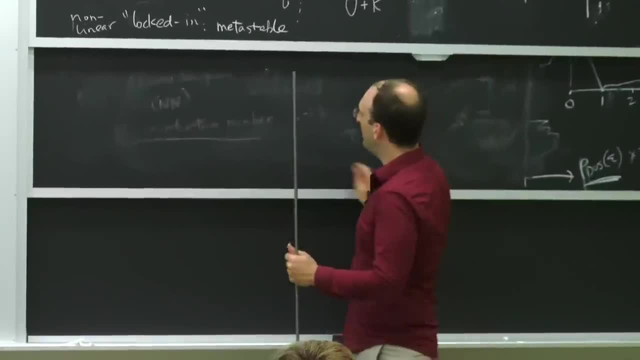 That's effectively how a reactor works. So we went over a little bit about the fuel, The fission and the energetics is kind of cool. So let's say you start off with uranium, probably the fissile isotope 235.. And you send in one neutron- I think it's 92. Don't quote me on that, though- And instead of undergoing some sort of a capture reaction or something else, it can split into what we call different fission products And plus anywhere between two or three neutrons. the usually accepted number is an average of about 2.44 neutrons plus gamma rays, plus Anti-neutrinos, plus other energy and some occasional other stuff. The main point here is these fission products. if, let's say, you had a uranium nucleus, 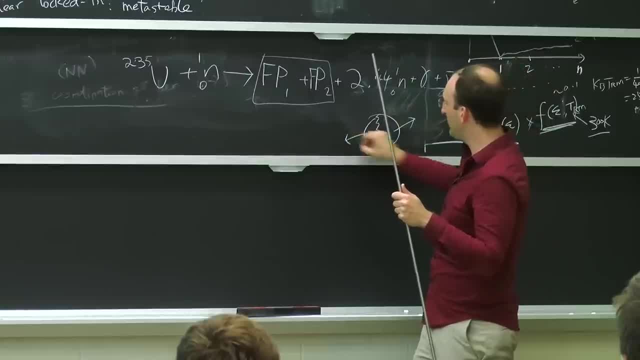 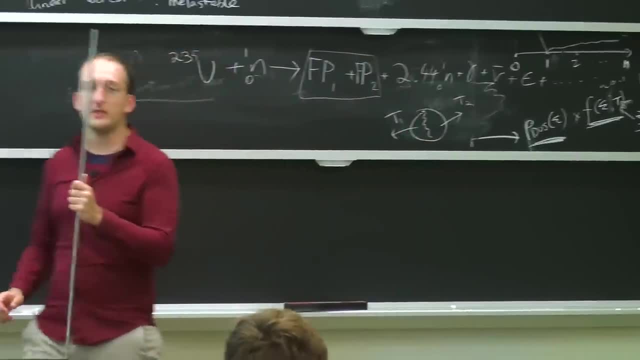 and it were to split in half. fission products go in other directions. They carry with them quite a lot of kinetic energy, And what we'll be doing a lot in the second half of this course is watching to see how do these highly energetic nuclei or atoms when they slam into other atoms. how quickly do they lose energy? How far do they tend to go? These fission products tend to stop in the fuel. Their range is going to be on the order of nanometers. I don't even think it reaches microns. 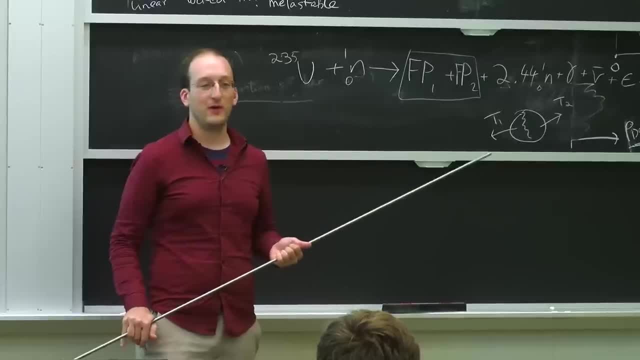 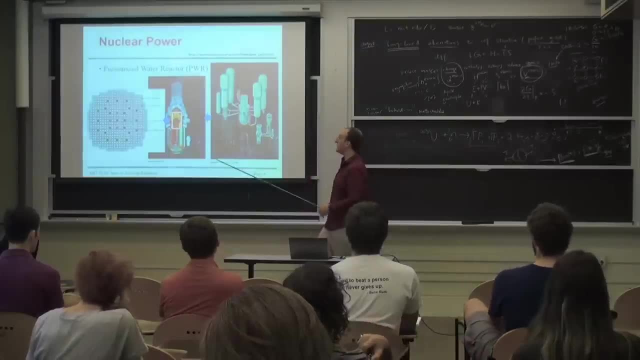 But the neutrons. however, as we saw from looking at Chadwick's paper, they can go pretty far, usually on the order of around 10 centimeters in a reactor before they go do something else. So it might make it a few fuel rods over. 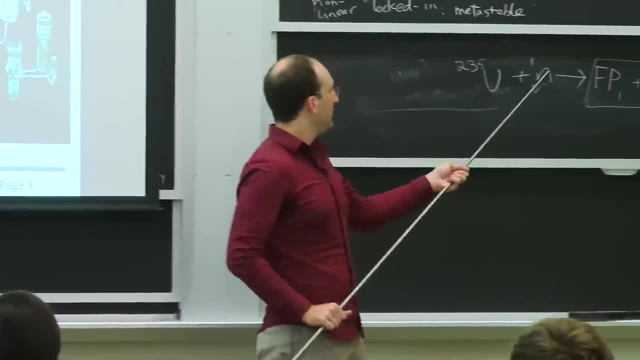 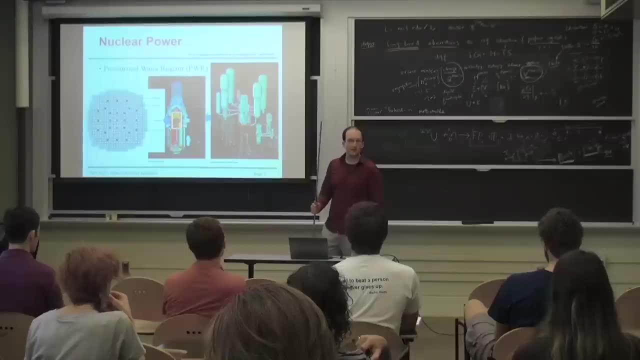 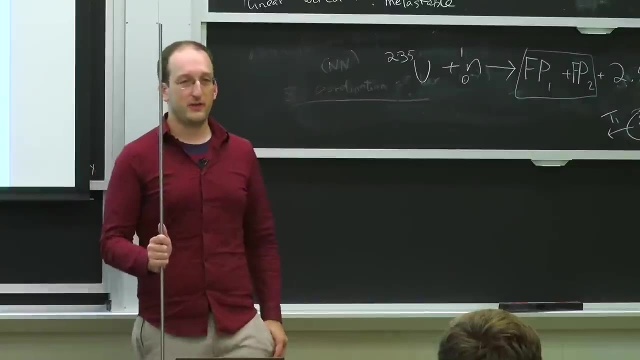 and chances are get captured by another uranium nucleus, making more fission, More neutrons and some other fun stuff like gamma rays and neutrinos. Anyone not know what a neutrino is. So a neutrino is a very, very low mass, but not massless. 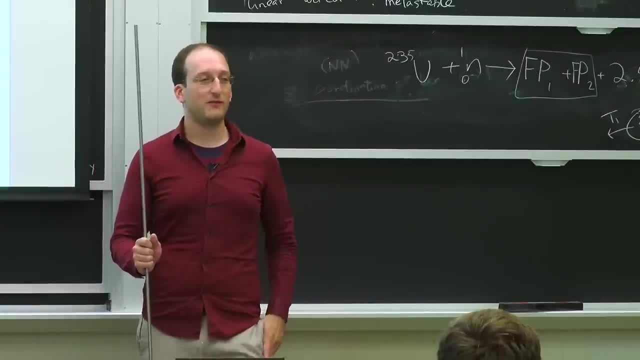 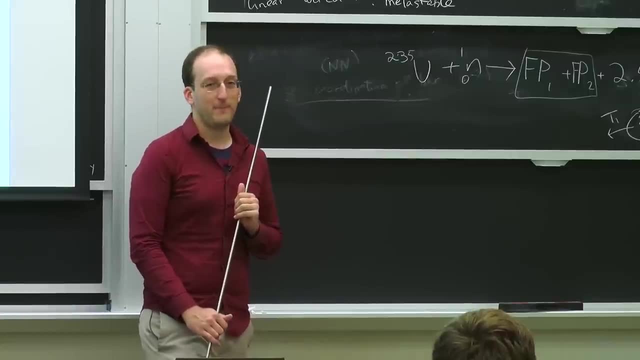 as was found, I think like last year, almost speed of light particle that's released as part of radioactive decay. They basically don't interact with matter, but once in a while they do. What that means is that they travel straight through everything. 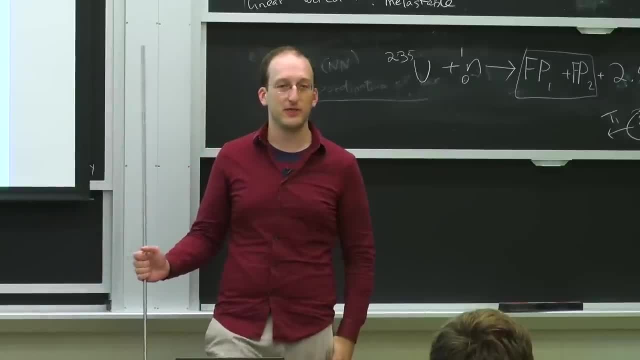 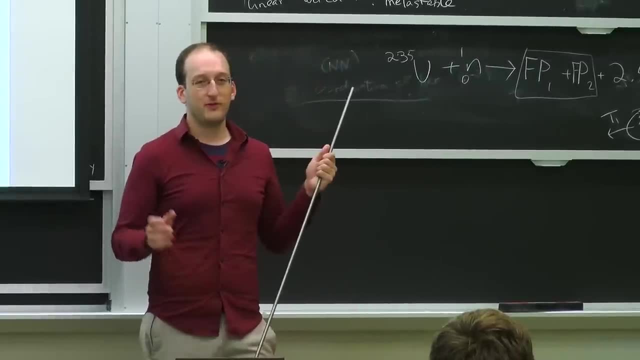 It's been estimated that trillions of neutrinos from space are passing. They're passing through us per second And on average, you won't get a single interaction during a day. In fact, to detect neutrinos, they've had to fill old, hollowed out salt mines with water. 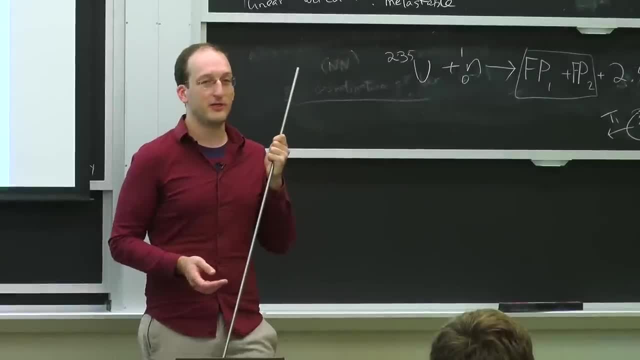 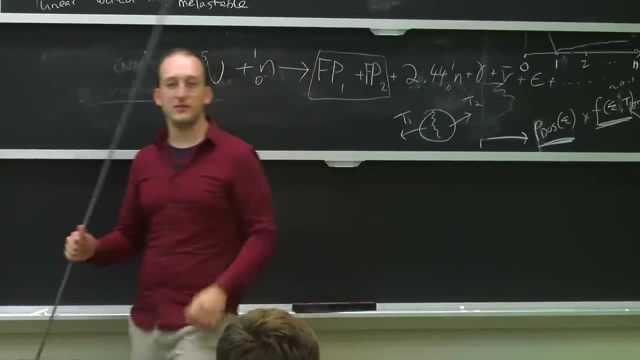 and fill them with photo tubes in the hopes of catching two or three a day. What that means is if someone turns on a reactor somewhere anywhere in the world, it's releasing tons and tons of neutrinos And if, all of a sudden, you start to see two or three coming, 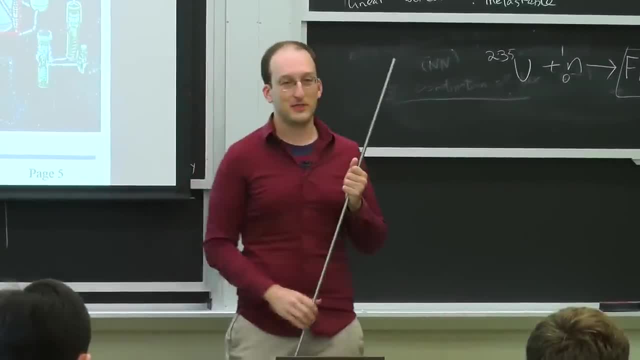 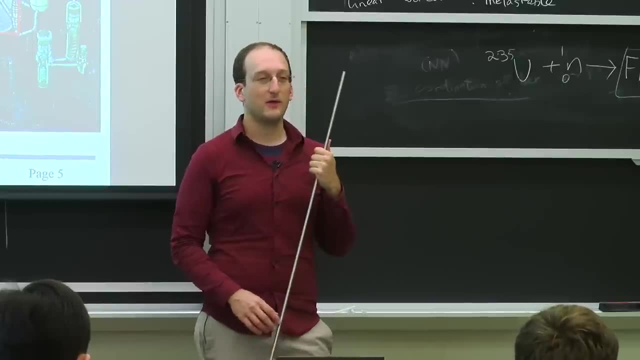 from the same place. that's a rare event, That's something with some statistical significance, And there's been projects And are still in our department using neutrino detectors to try and detect where reactors are turning on anywhere in the world. So we've been able to sense that the MIT reactor is next door. 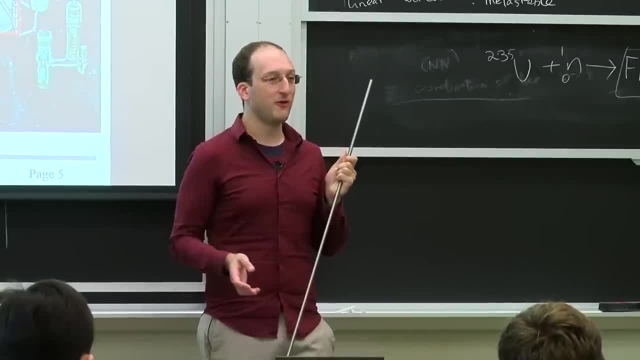 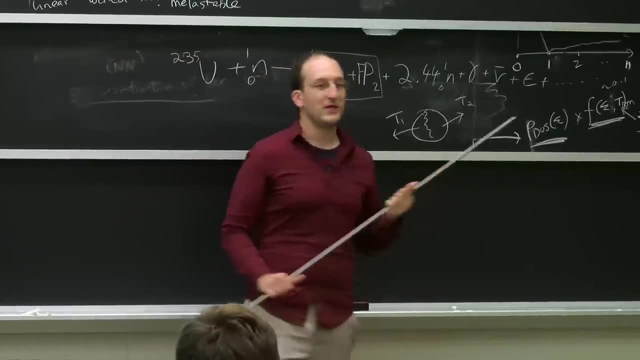 from the building next door. I don't know how well this is going to work when you get to farther distances, but the physics is pretty much there. It's an engineering problem to figure out. well, how do you detect enough neutrinos to get a statistically significant signal? 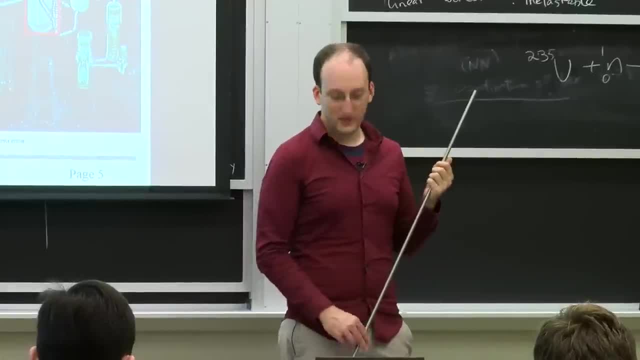 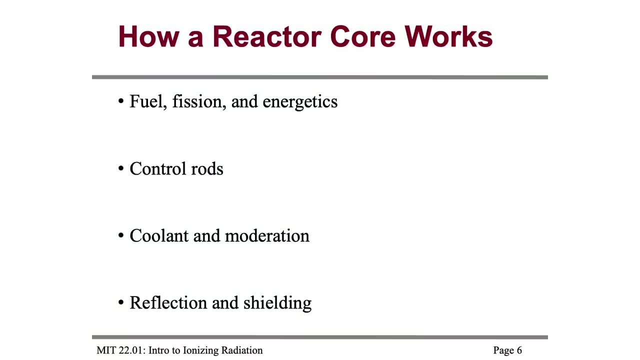 That, as far as I know, has not been solved. Hopefully by this time next year it will. There's also control rods, rods filled with absorbers, like I mentioned before. If you want to stop this nuclear reaction, you send in something like hafnium or gadolinium. 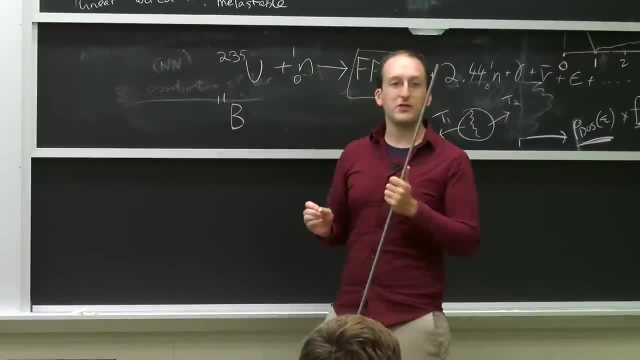 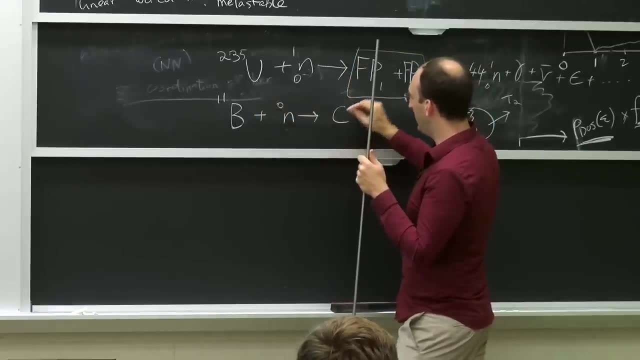 or boron. So let's say boron-11,, like Chadwick knew, would be able to capture a neutron, And then it would turn into what's the next one over? Well, sorry, that's a 1 and a 0.. 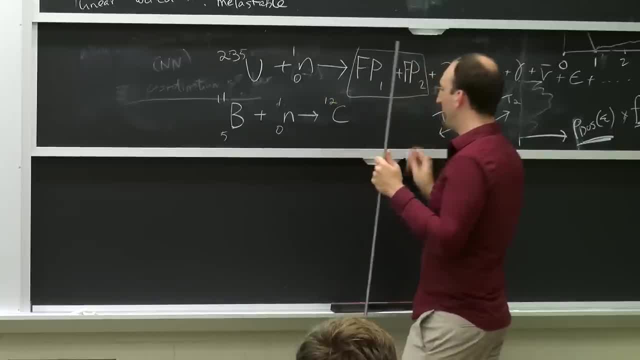 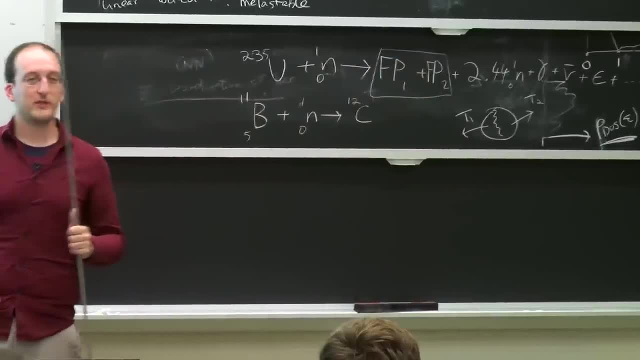 That's a 5.. That should turn into carbon-12.. And then you've captured it. That's a 5.. You capture the neutron instead of letting it get into more uranium and cause additional fissions. So when something's going wrong or you. 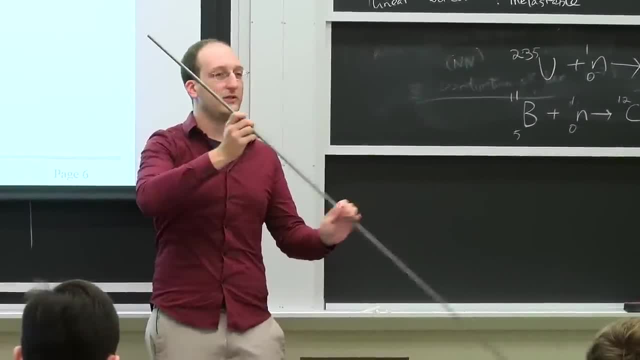 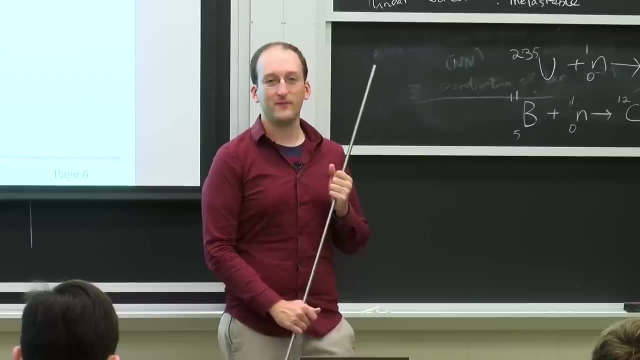 want to control the power level in the reactor, you insert control rods. They soak up the neutrons and make the reactor go subcritical, And we'll go over what all these words mean in due time. various points in the course. There's also coolant and what's called moderation. 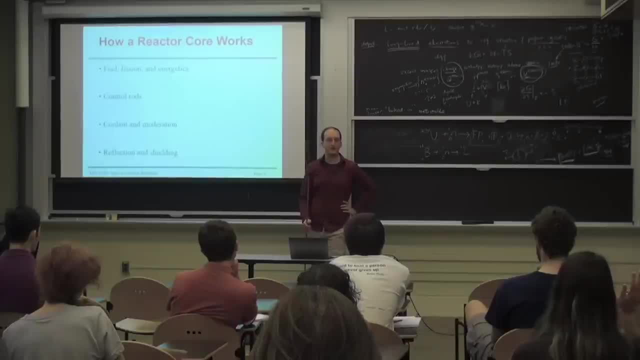 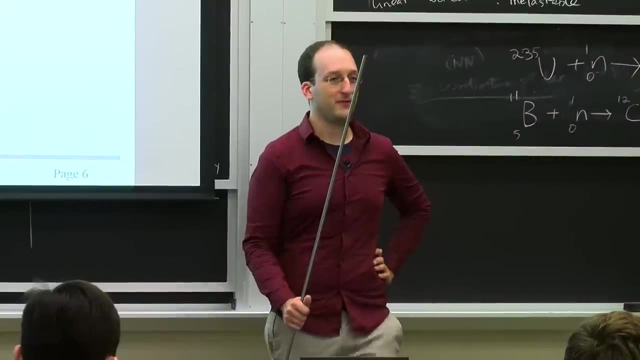 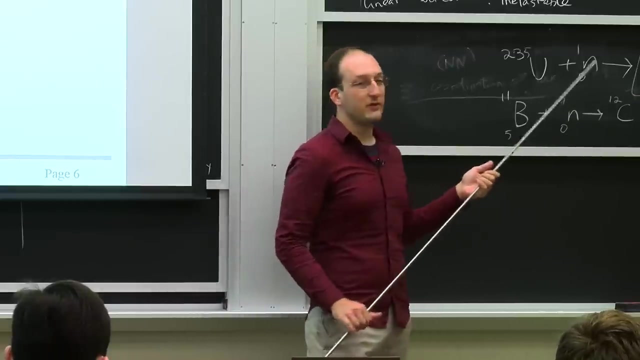 Does anyone know what I mean by moderation of neutrons? Yeah, What do you mean? It thermalizes them. It thermalizes them And, in other words, it slows them down, Because the probability that each uranium nucleus can capture a neutron depends on the energy of the neutron. 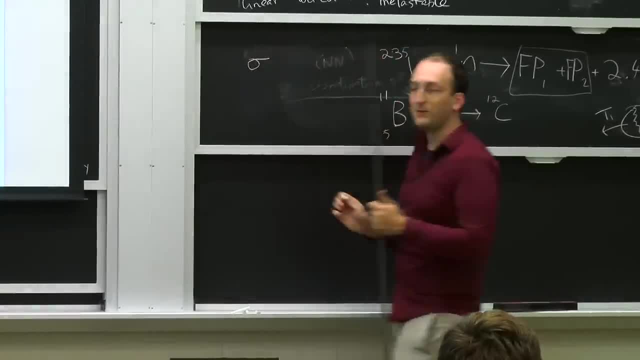 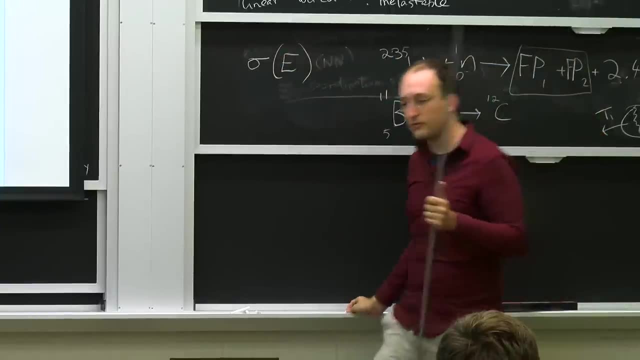 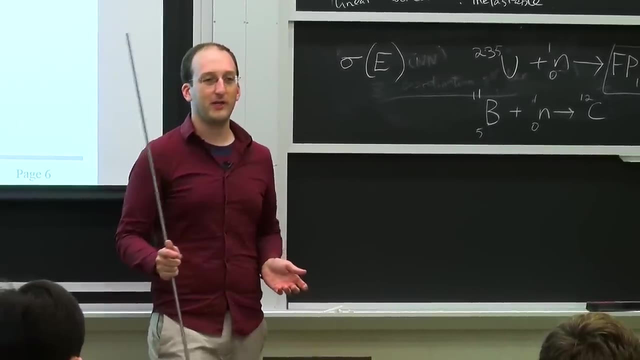 The cross-sections for interaction which we give the symbol sigma for the microscopic or sort of mass-independent cross-section. they're functions of energy. They're extremely strong functions of energy over the energy ranges we're interested in, Because we're interested in an extremely large energy range. 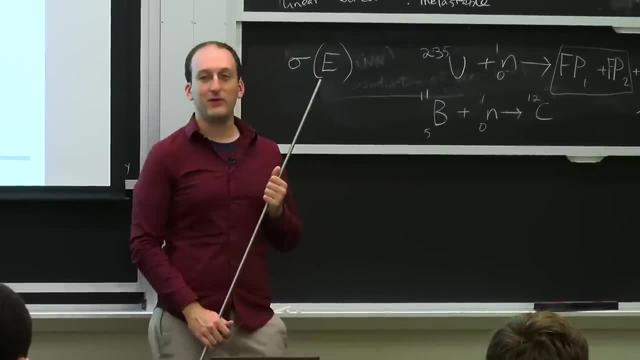 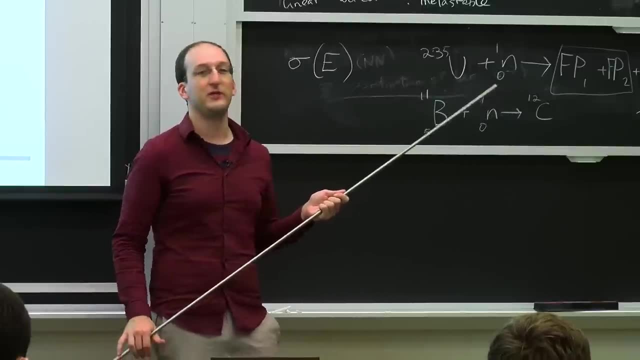 These neutrons Tend to be born at around 1 to 10 MeV or mega electron volts And by the time they thermalize, like you said, or reach roughly room temperature, kinetic energies of about 2,200 meters per second. they can be a 40th or 0.025. 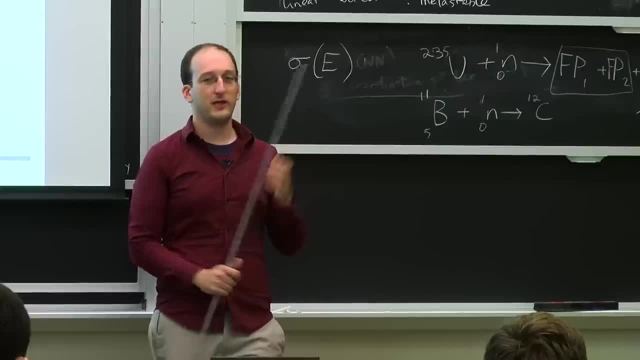 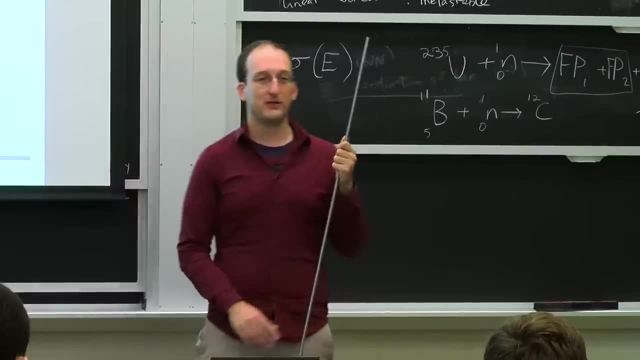 Ev, a fraction of an electron volt. So we're interested in nine orders of magnitude of energy And the cross-sections vary wildly over these nine orders of magnitude, And I'll show you what some of these look like pretty soon. And In this case, in the case of light water reactors. 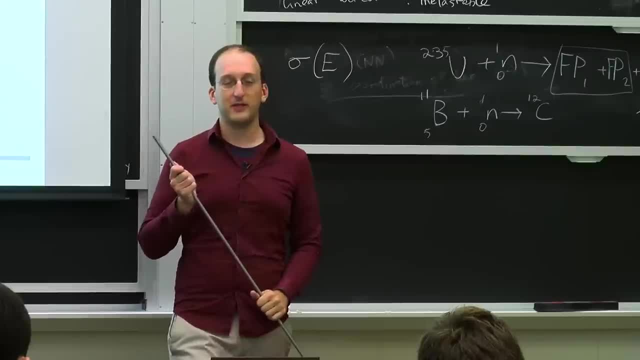 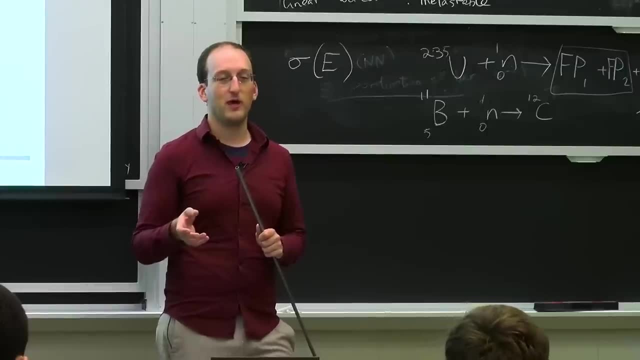 like the PWR we saw the coolant and the moderator are basically the same thing. You guys remember how, when Chadwick put the paraffin in front of the neutron source, he started to see more ionizations. That's because the paraffin is a great source of hydrogen. So is water. Water is an ideal coolant because it takes a lot of energy to heat it up and a lot to boil it, So you can store a lot of energy with less of a temperature difference in water, And it's full of hydrogen. And kinematically it's a lot of energy. It's easier for something the size of a neutron and the mass of a neutron to slow a neutron down, Because a neutron hitting a proton can transfer up to all of its energy ballistically. Then that proton won't move very far because it's also got charge on it. If a neutron hits something heavier, like stainless steel or other stuff in the reactor, it cannot, by conservation of energy and momentum, transfer all of its energy. 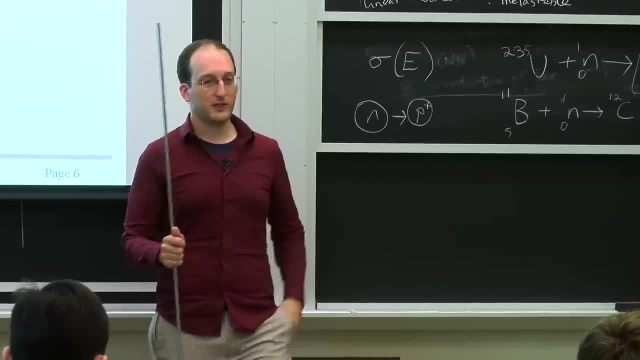 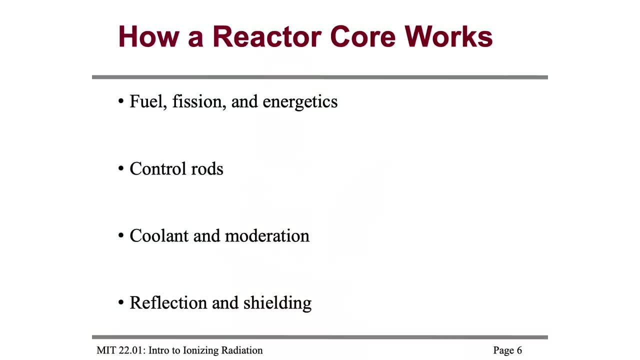 That fraction's actually pretty small. So you'll see, we'll actually calculate what that fraction is, But it drops off pretty precipitously as you start to get heavier than hydrogen. And finally there's reflection and shielding. We'll get into shielding in terms of how much stuff. 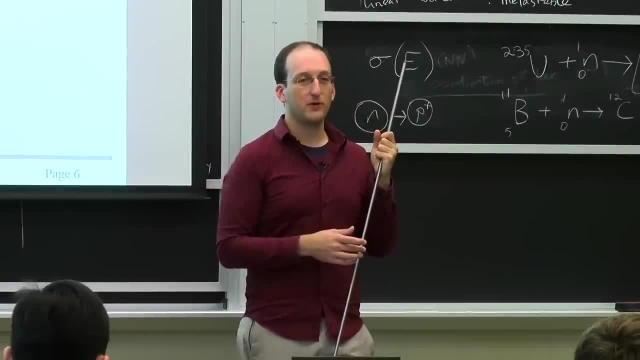 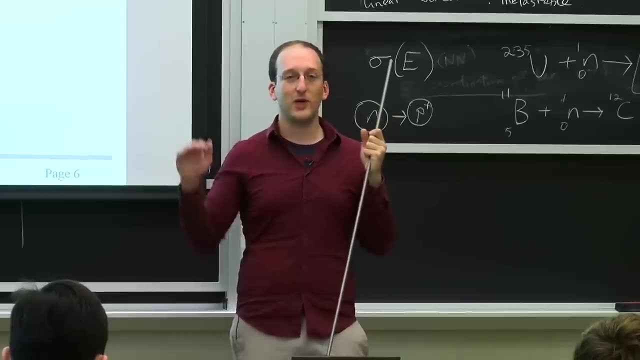 and how much matter does it take to stop radiation from getting through? In some cases you can stop it all. In some cases, like gammas, you technically never can. You'll just get what's called attenuation or continuous removal of gamma rays. Chances are you can't remove every single photon from getting out. It's only a matter of how much do you need it to get down to. And there's a neat aside: Who here has looked down into a nuclear reactor before Three of you? 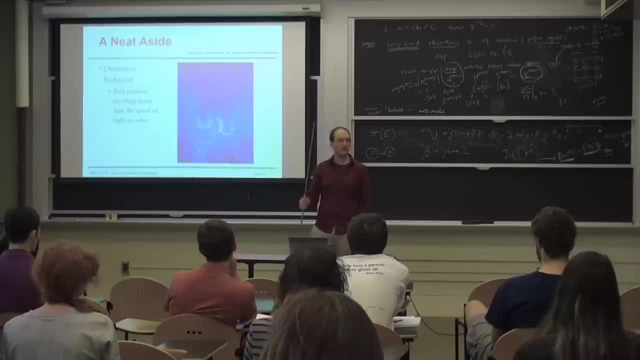 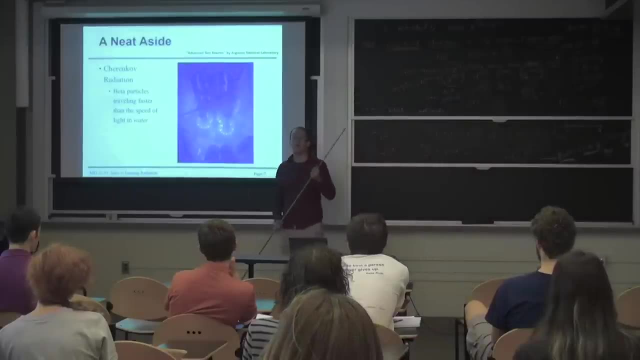 Wow, Four. OK, What did you see? Not that much, Not that much. This is a particularly powerful reactor known as the Advanced Test Reactor, or ATR, at the Idaho National Laboratory. You won't see any others that look like this. 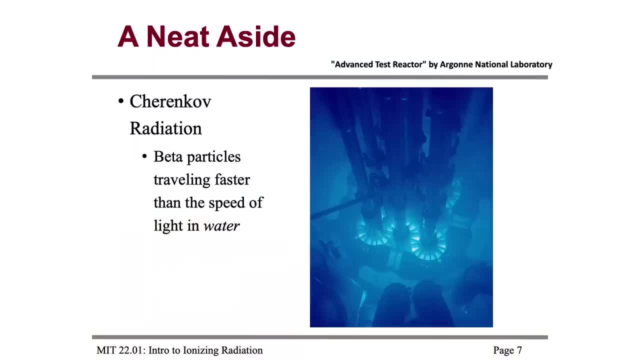 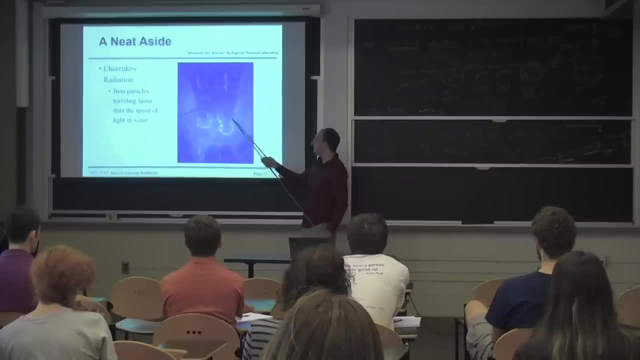 One, because these crazy shaped fuel elements are not that easy to make. This is a test or a research reactor where things get irradiated. It's about 125 megawatts And the blue light being produced is called Cherenkov radiation. 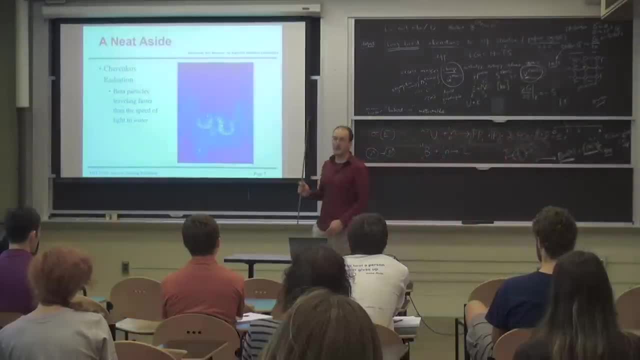 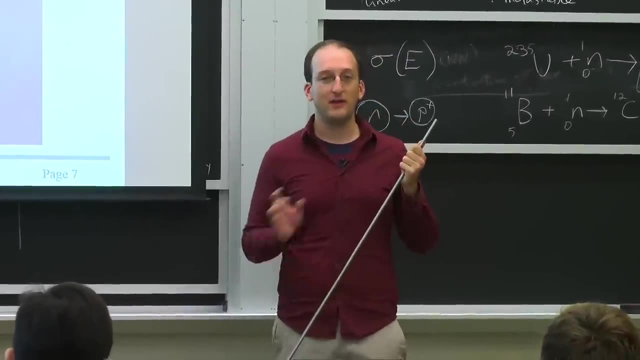 It's from electrons and things moving, or beta particles, electrons moving faster than the speed of light in water. Now, as you know, you can't exceed the speed of light in a vacuum, But things can move through other media faster than the speed of light in that medium. 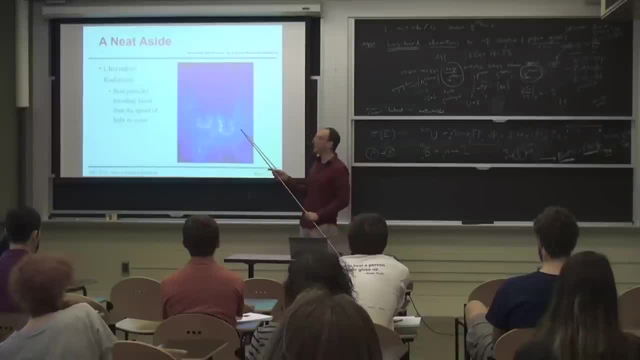 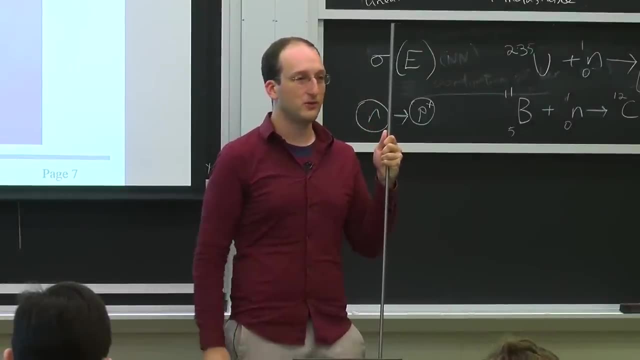 effectively producing optical shockwaves. And you can see that in this example. you can see that there's a little blue cone of light in the middle of each particle. And you can see that there's a little blue cone of light in the middle of each particle. 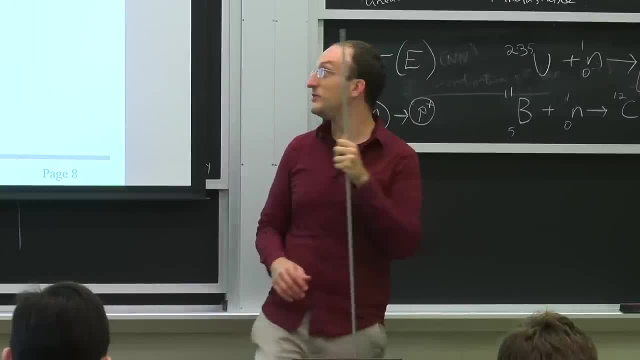 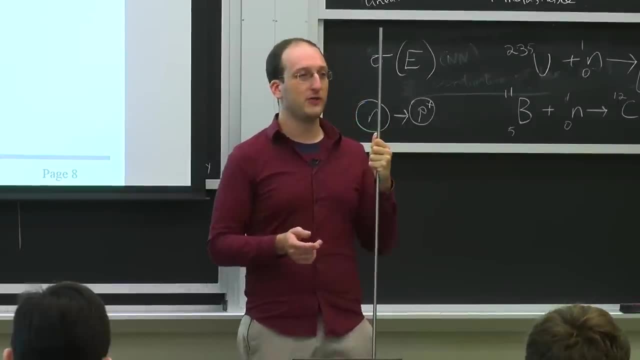 So when folks say, oh, am I going to go green when I get near radiation, You can say no, you'll glow blue. They've just got the wrong color on all the TV shows. And then on to fusion energy, since most of us 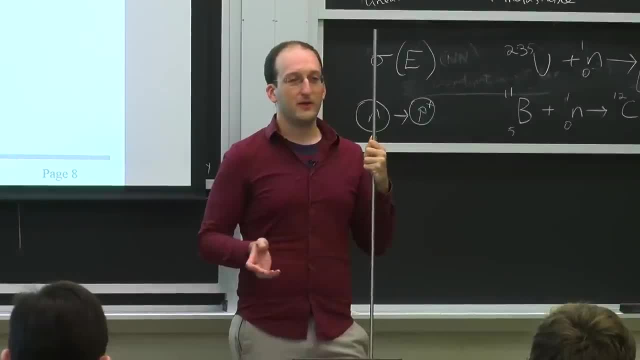 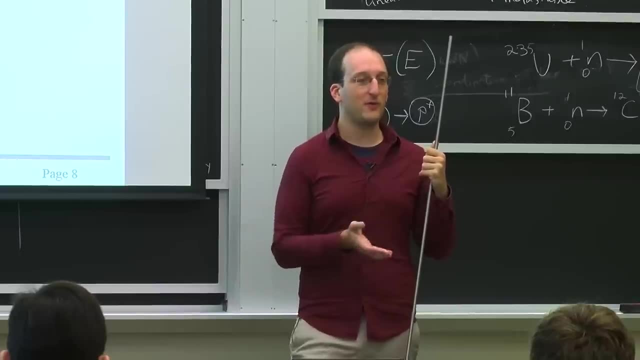 tend to talk about fission a lot of the time, But how many of you here are interested in going into fusion? Usually it's at least half the class, And so I figured this used to be where there was equal time, because about an equal number. 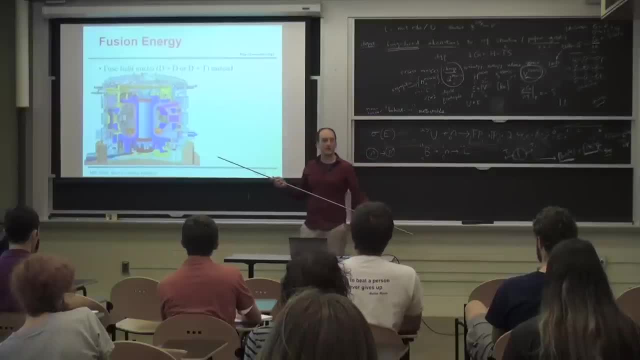 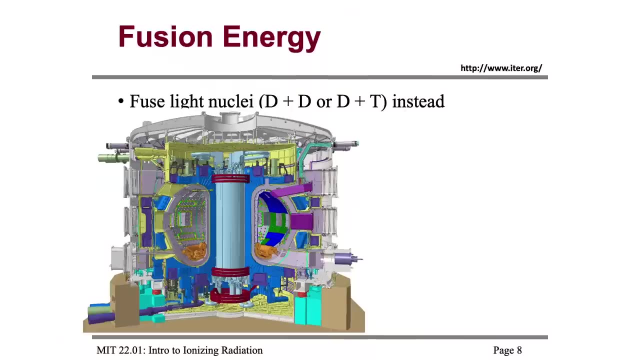 of you want to go into fusion to make it a reality. These reactors are laid out fairly differently. What they'll be is a big hollow vacuum chamber that's shaped like a donut or a torus and lots of magnets to confine a plasma or sort of a charged mess. 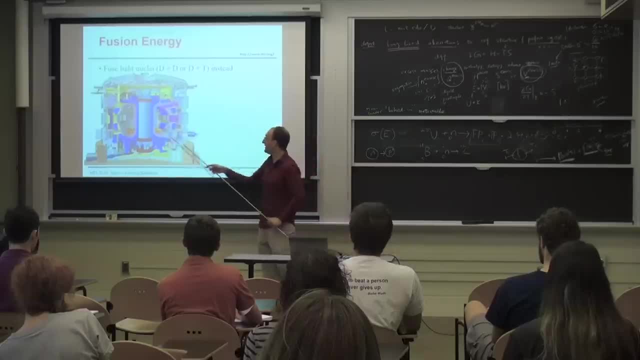 of separated ions and electrons that whirls around at millions of meters per second. Once in a while, these ions and electrons, or especially these nuclei, will collide with each other and undergo a fusion reaction, or one of a few fusion reactions that I've written up here for you. 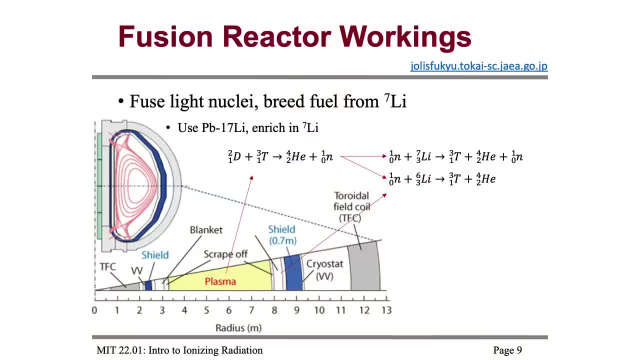 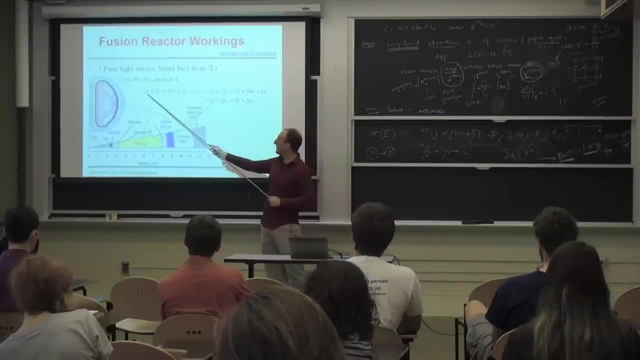 So in this case there's no elements with the symbol D or T. We're just using those to refer to deuterium or tritium as a visual aid. But you should know that they're deuterium and tritium from their atomic numbers 1, which 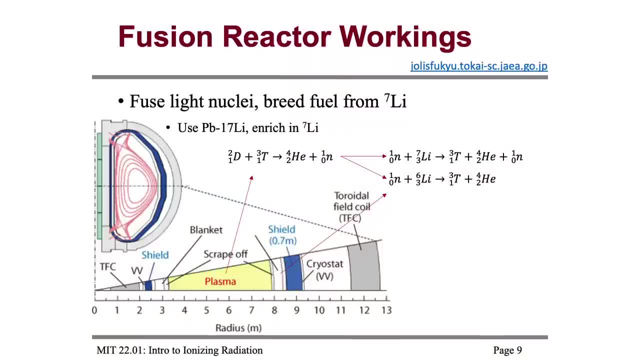 means it's an isotope of hydrogen and their mass numbers 2 and 3, which is not the mass number for normal hydrogen, And in this case, when you fuse deuterium and tritium, you can produce helium. 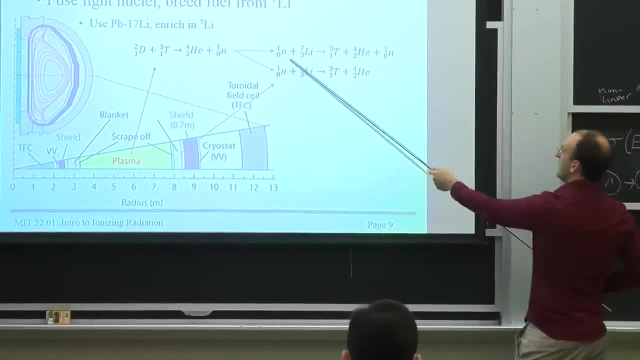 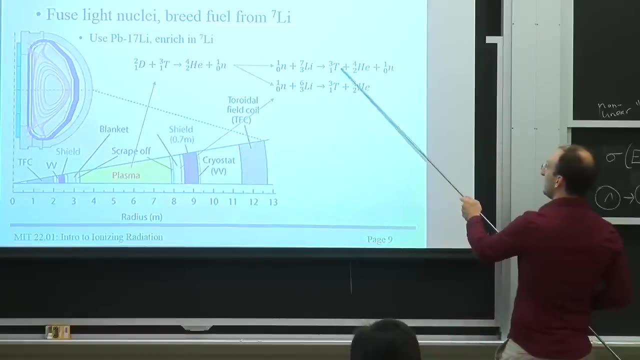 And another neutron, And so then those neutrons can be used to hit lithium, which they'll usually have in what's called a breeder blanket around the outside which releases more tritium, So fusion reactors actually can produce their own fuel. 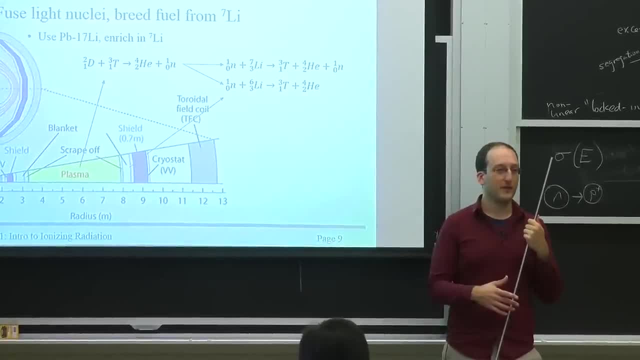 The trick is they're radioactive gases, so containing them can be kind of tricky. You also need a way to get the helium out of the reactor, But we have one of these on campus. We have one of the only three in the country. 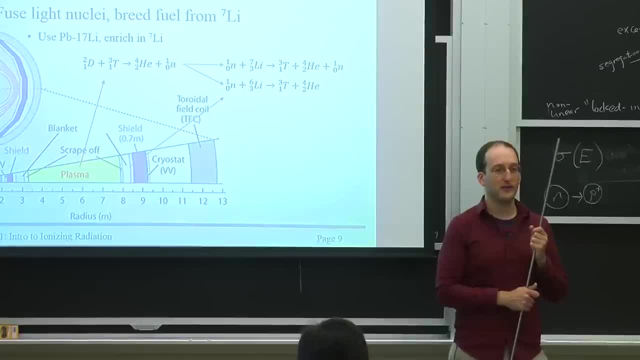 It's called the Alcator C mod. Have any of you guys seen a tour of this place yet? Almost all of you, So if ever, who hasn't do it this year? because this may be the last year of Alcator C mod's? 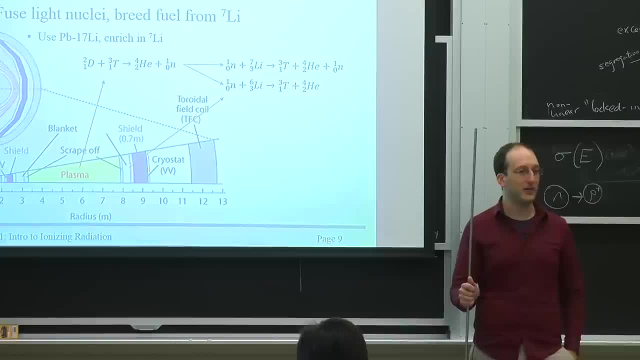 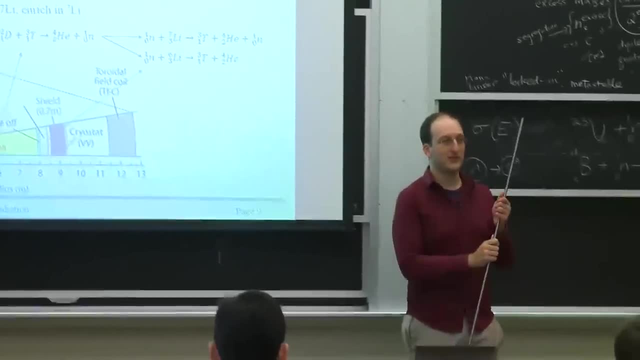 operation. That's not to say there won't be the next fusion device on campus, but there's one here right now and it might be a while before the next one's built. So if you haven't seen it yet, go and see it this semester. 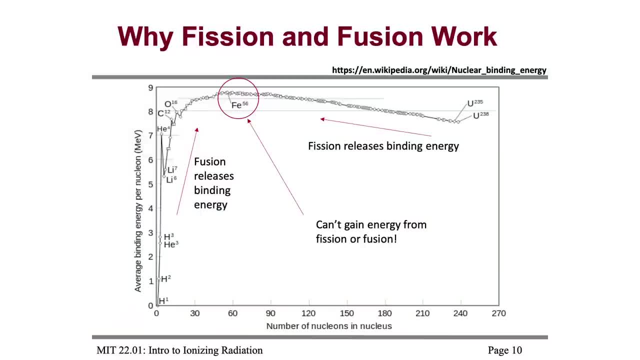 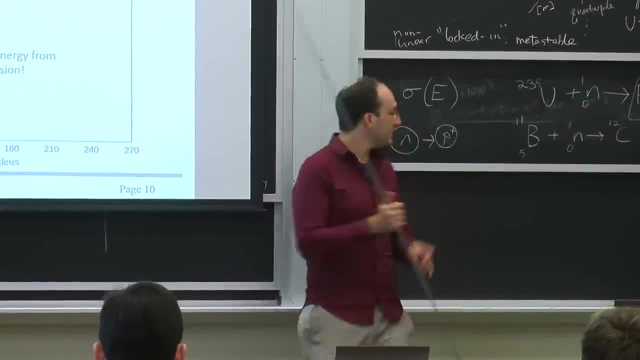 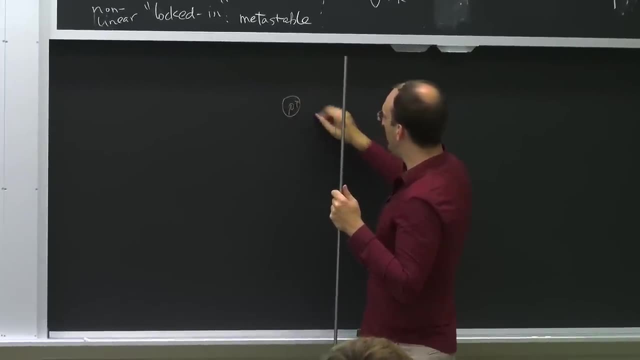 definitely. The reason why fission and fusion work from an energetic standpoint is if we look at the binding energy per nucleon. remember last time we mentioned the binding energy Is the difference in energy if you were to take, let's say, a proton and a neutron from infinitely far away. 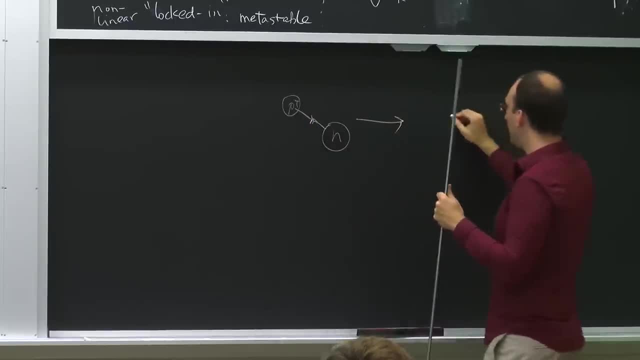 and bring them together to create a nucleus of deuterium. we'll call this d, These two, the energy of the proton plus the energy of the neutron, the rest, mass energies rather, would be greater than the energy energy of just deuterium. 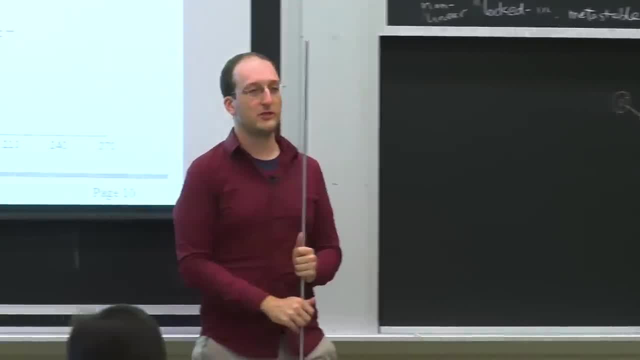 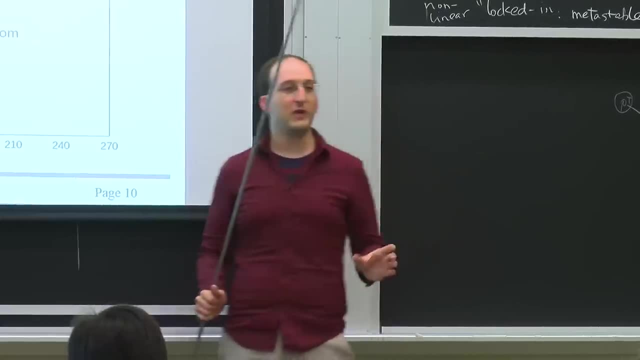 And that little bit of mass that's changed is converted into energy, And this is what's known as the binding energy. If we look at the binding energy per nucleon, or per proton or neutron, we can get a relative ranking of how tightly bound each nucleus is. 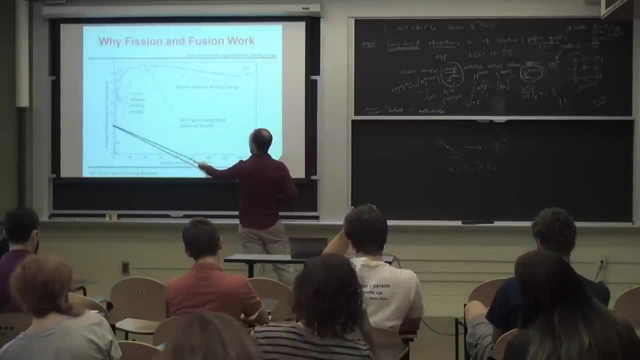 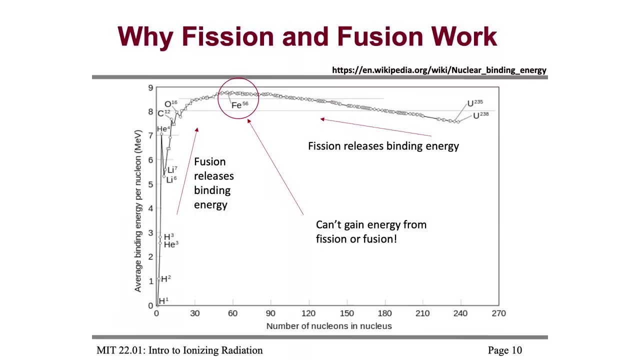 So for the light isotopes, smashing them together should liberate excess binding energy, or sorry, excess energy, because you'll gain back some of that energy by the conversion of mass to energy. Same thing over on this side, just not as extreme of a gradient. 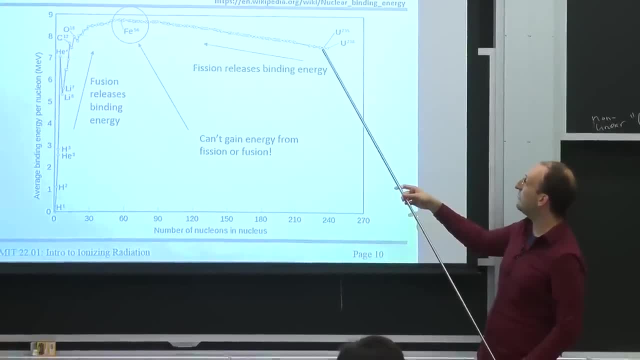 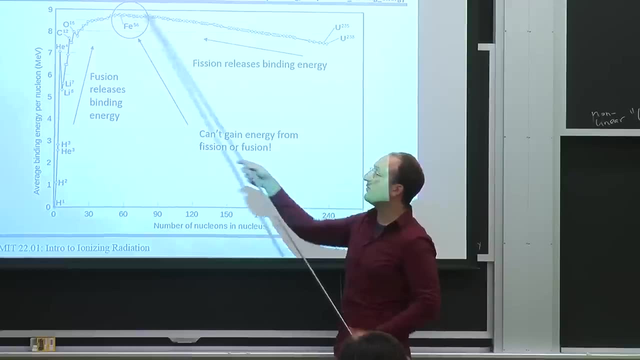 If you were to split apart heavy nuclei like uranium-235,, you can release a little bit of energy in fission, And once you get up here to iron, you can't go either way, which is why, if you think about the biggest fusion reactors, that exist in the universe. anyone know what they are? Stars, right, They tend to hit cores of iron before they either die out or go. They go all gravity crazy and become black holes or supernovas or whatever you will. This is kind of the energetic limit. 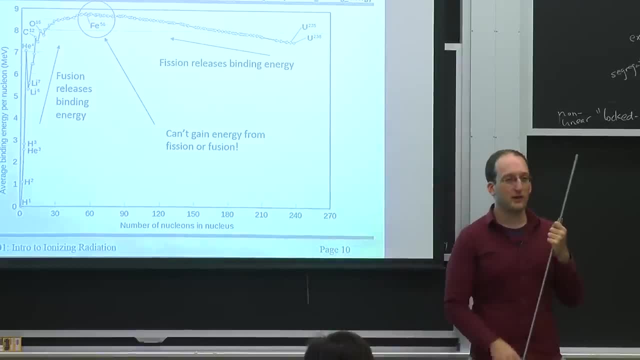 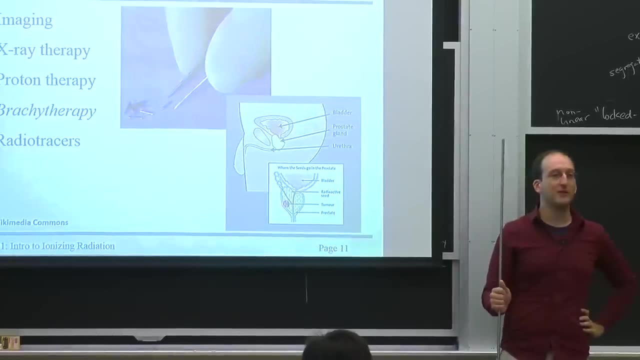 for normal nuclear processes Or if they become a neutron star, then things get beyond the scope of this course. I won't be explaining neutron stars. There's a lot of medical uses of radiation. I don't know if any of you guys have seen these things. 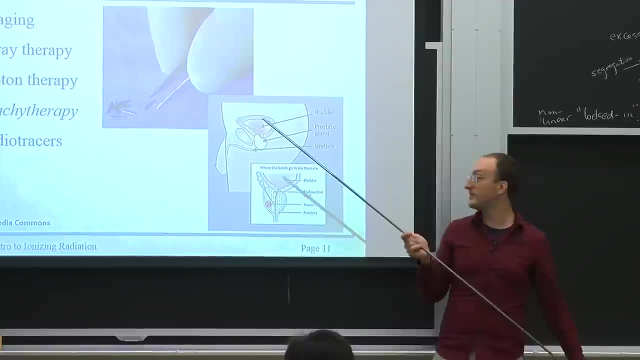 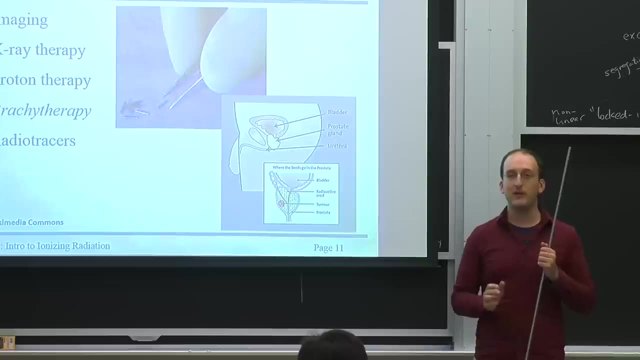 It's the only time I'll show a tricky looking biology diagram, because it's kind of interesting to note. These are what's called brachytherapy seeds, little seeds of isotopes. These are isotopes that emit a certain type in energy of radiation, selected for their applicability. that 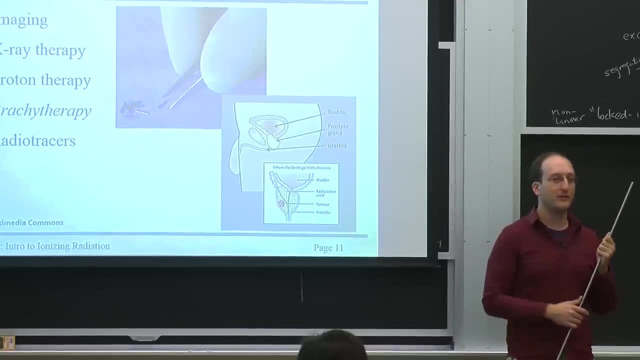 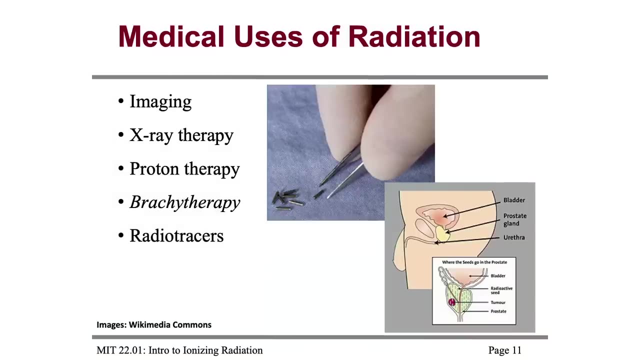 can be implanted in the body at the site of a tumor to deliver localized radiation treatment. You can either go in through existing ports on the human and not having to drill or cut a hole in someone, or they can be implanted laparoscopically or surgically. 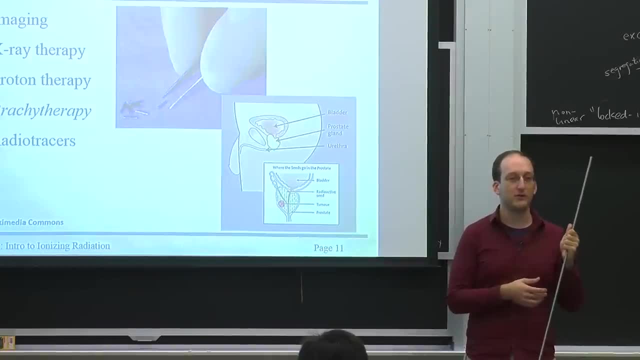 So this way, if you don't want to subject someone to a whole body radiation dose or chemotherapy, or if you want to use it in conjunction with chemotherapy, you can implant a tiny little seed of a radioactive material in there to deliver a certain dose to a tumor. 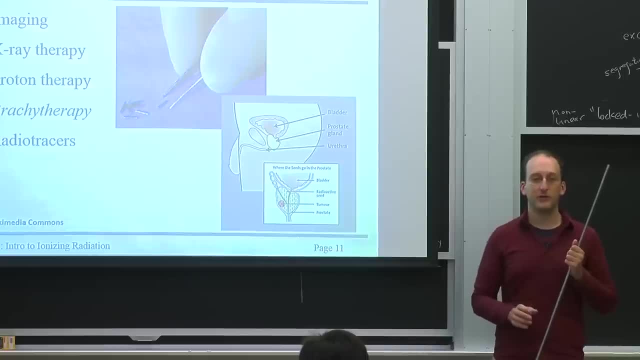 and then take it out And that way you know very, very well what the dose is going to be, because you can measure the activity or the number of decays per second of that brachytherapy seed and you know how it's going to change over time. 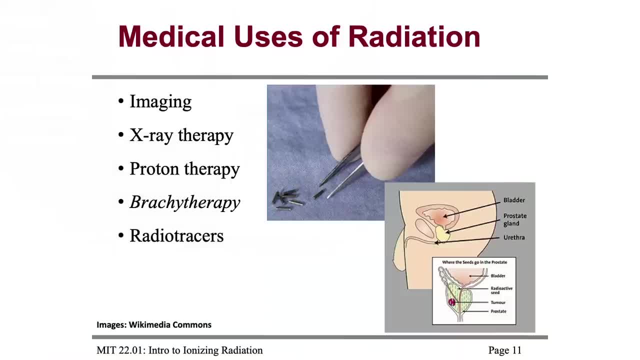 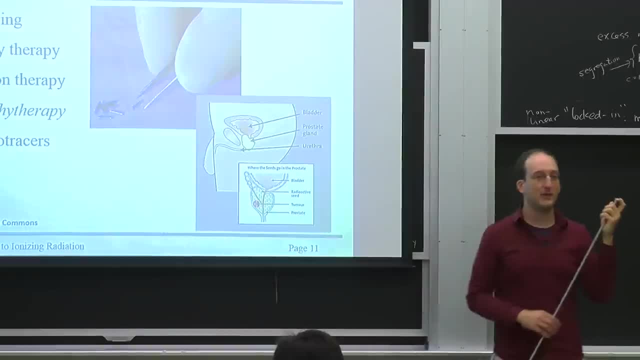 because you know the half-life of the particular isotope that you've looked at. There's also things like imaging. You can have someone ingest an isotope like technetium-99 metastable to highlight certain organs or things in the body. 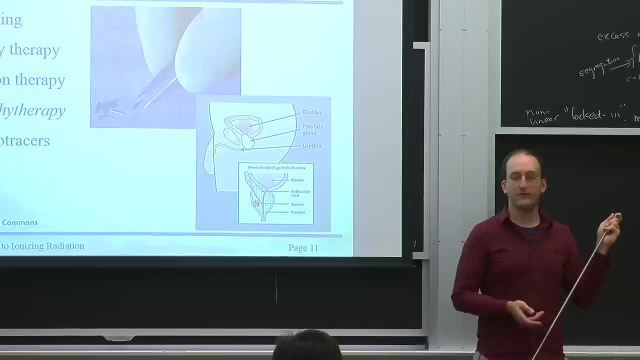 That you can then image later by their decay, gamma rays or other phenomena. It's also one of those reasons why, when you go in an airport, you have to tell them if you had a medical imaging procedure, because a lot of these places have radiation detectors. 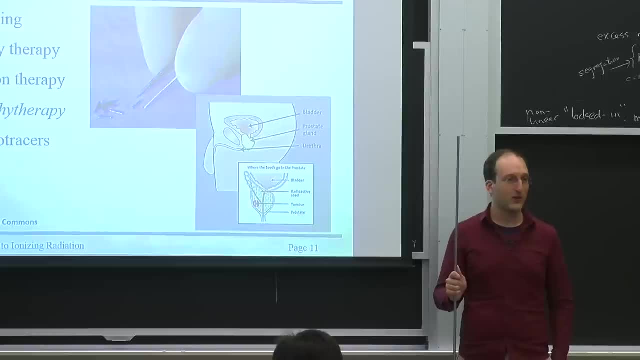 And if you are radioactive and don't identify yourself, you will quickly be identified and taken into the back room to the probulator or whatever they're going to do at the airports. I don't know. I've never been searched. I don't plan on that happening. 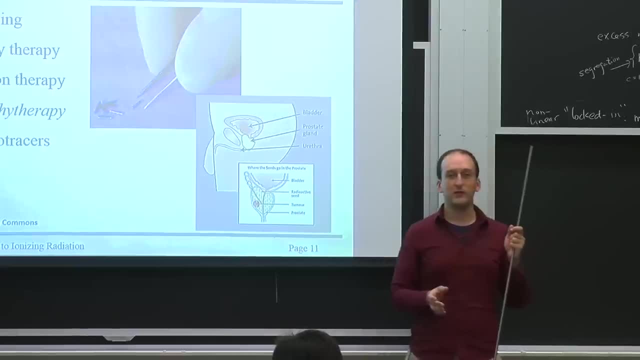 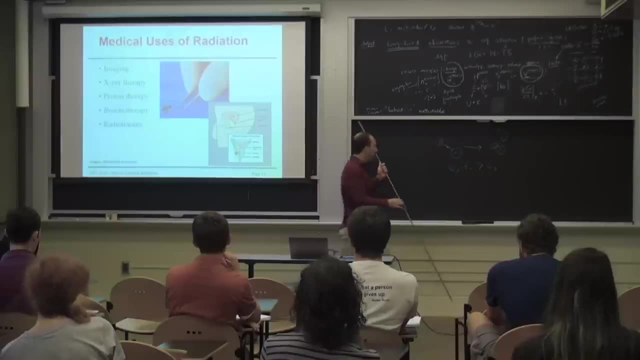 There's also x-ray and proton therapy, sending in well-known, well-energy-characterized radiation to fry tumors or other things. In the case of x-rays, you're relying on what's called exponential attenuation If you look at the distance into a material. 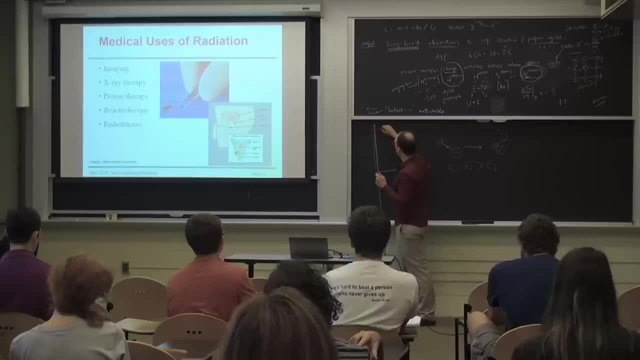 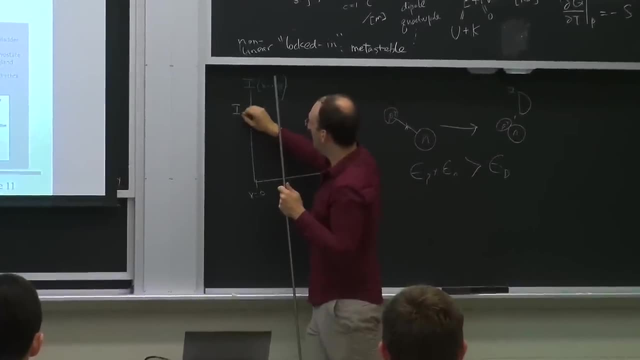 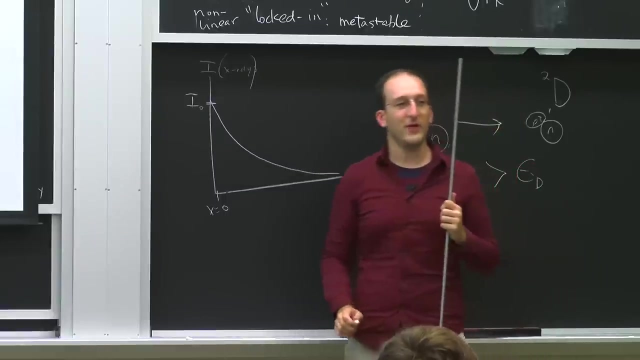 and you look at the intensity of the x-rays, say, at x equals 0,. this is your x-ray source. This is your incoming intensity. It falls off exponentially with distance. You might then ask yourself: all right, if my tumor is this deep? 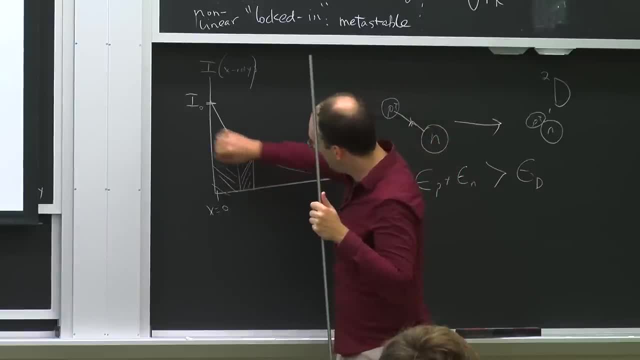 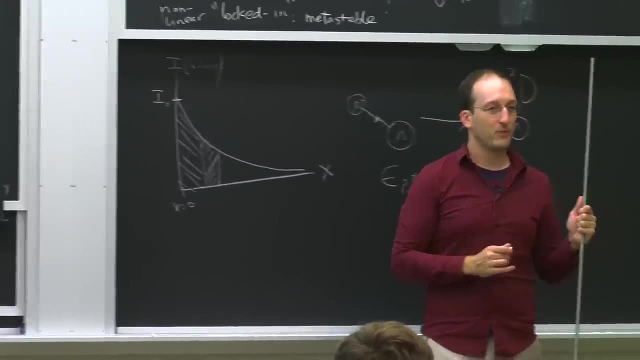 and I apply that radiation dose to the tumor. what about the rest? What about the part of the body that the x-rays have to travel through in order to get to that site? Anyone know how you would deliver more x-rays to a tumor than the surrounding tissue? 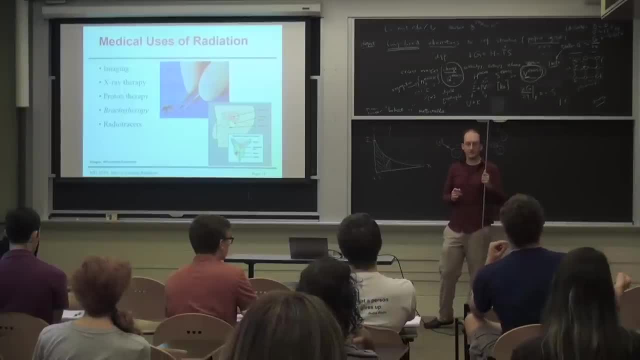 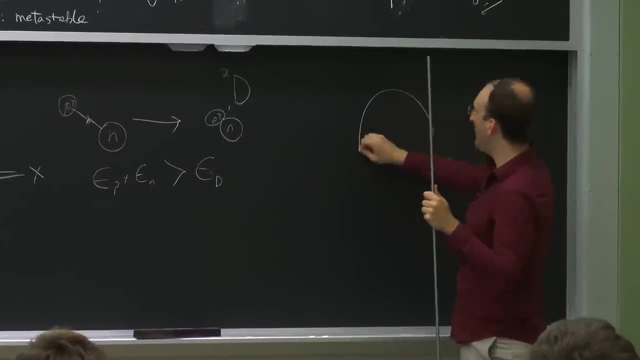 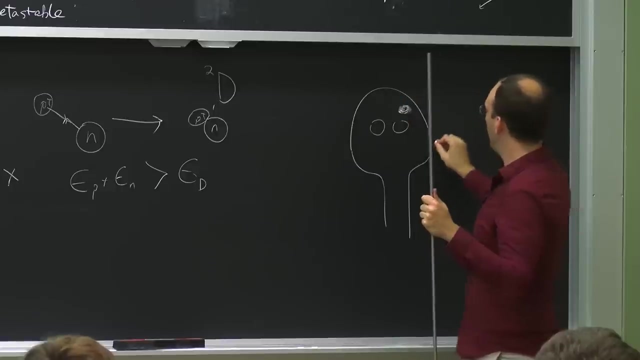 Anyone have any ideas? Yeah, Go from different angles so the rays intersect on the tumor. Exactly, Go from different angles so the rays would intersect on the tumor. I'll have a better diagram, but I'll draw one for now. Let's say: that's the eyes and that's the tumor. 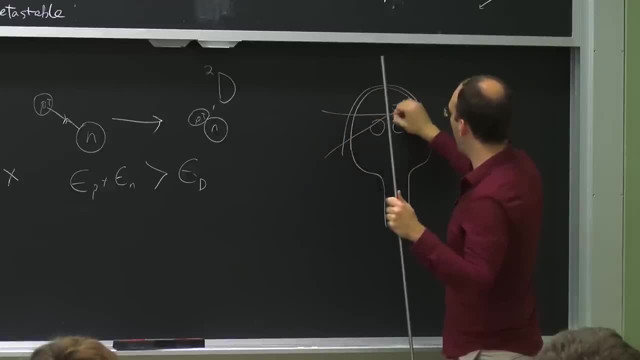 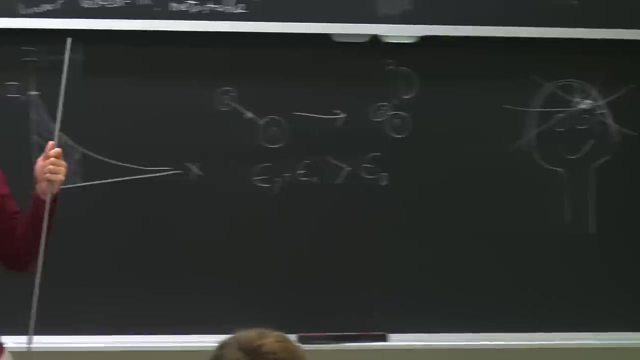 You can wear this helmet where x-rays can come in from all different angles And the x-ray emitter would have to come in from different angles so that, as all the rays intersect, this part gets fried the most, while keeping you from getting too much radiation to the rest of your brain. 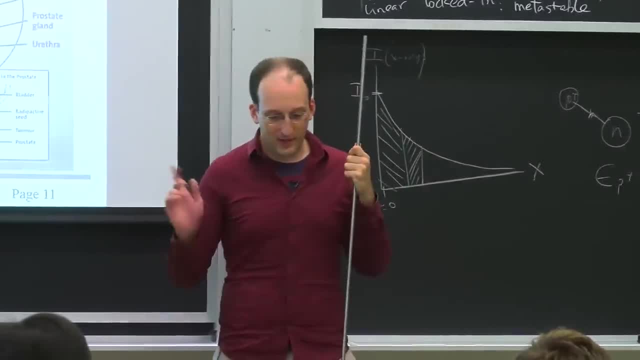 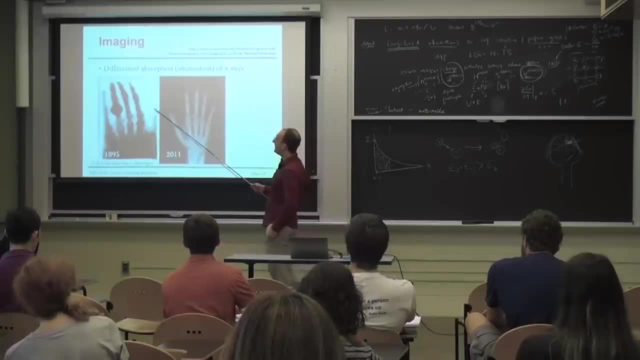 and ceasing to function. There's also radio. There's also tracers. I think I already covered those. So imaging- we already showed an image of what this looks like. The first x-ray back in 1895 didn't have that good resolution, but it was striking in that. 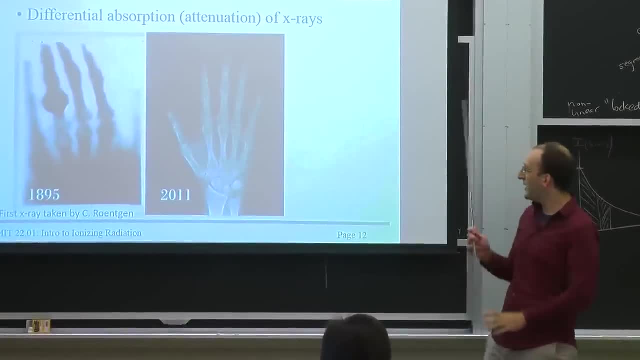 You could see the difference in contrast between bones and tissue. I should replace this with the x-ray of my foot. That was my signing bonus at MIT. My first day on the job, I went down to clean one of the old rooms in Northwest 13,, which. 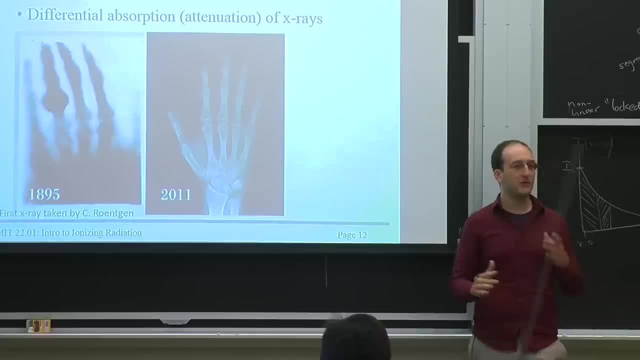 is now where my labs are, And I moved a bunch of boxes aside and a 200-pound steel plate, Jagged, cut with plasma torch, went down and smashed down on the bones of my foot And I had one of those temporary feats of superhuman strength. 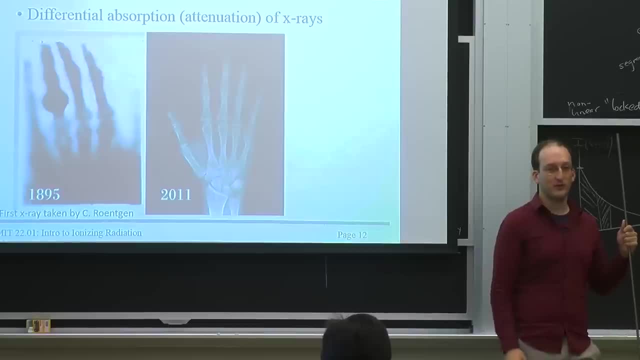 and was able to lift it up. I went back to try to lift it up and couldn't move it an inch. I don't know how I got out of the plate. The next thing I remember I was crawling up the stairs to go to the hospital. 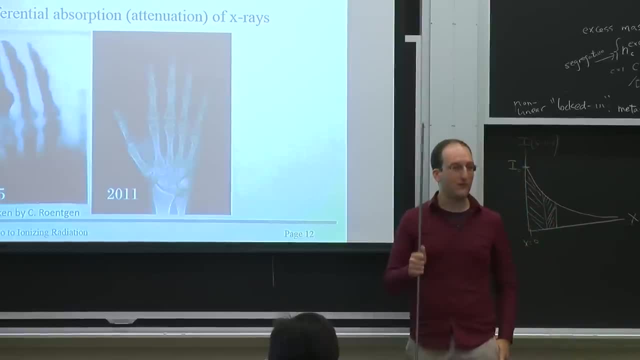 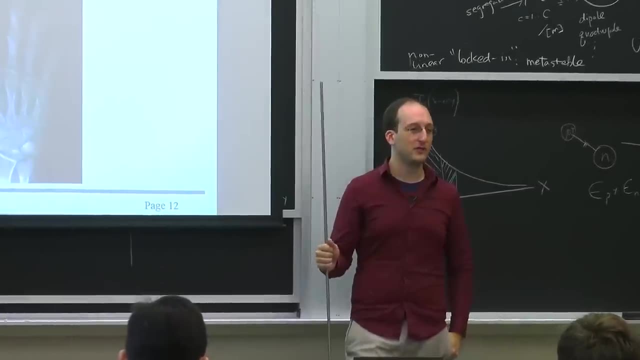 But I did get an x-ray and they were able to sense that the pain in my foot was due to a hairline fracture. It was like a fracture in the bones that basically came back together. But the improvement in contrast resolution in x-rays- 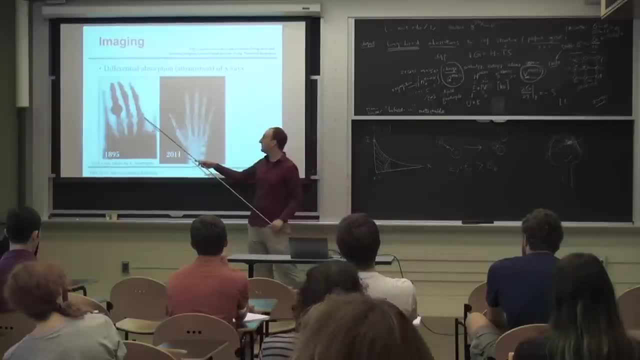 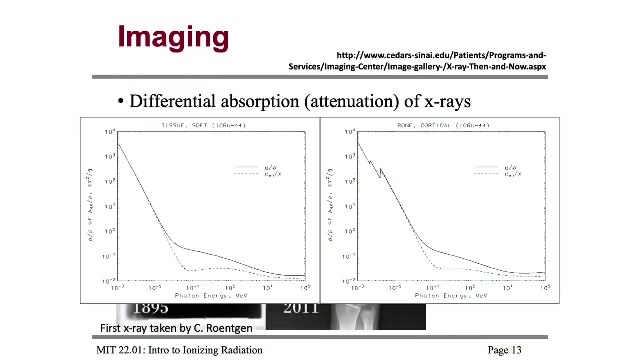 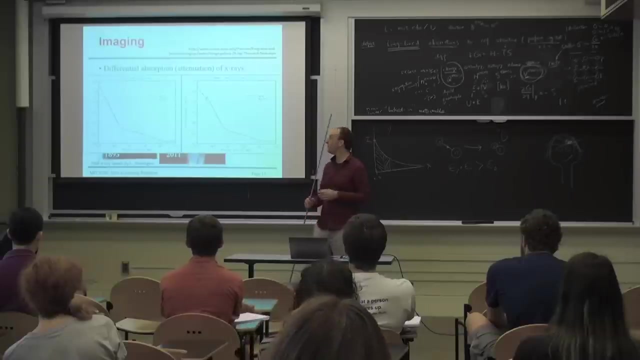 is what differentiates the ability to see a hairline fracture from just the ability to see that you contain bones. And the reason for this- and we'll be looking at a lot of these curves in this course- is the differential absorption or attenuation of x-rays or any photons of any energy. 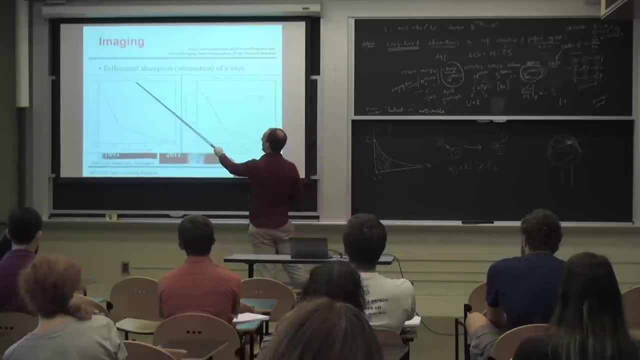 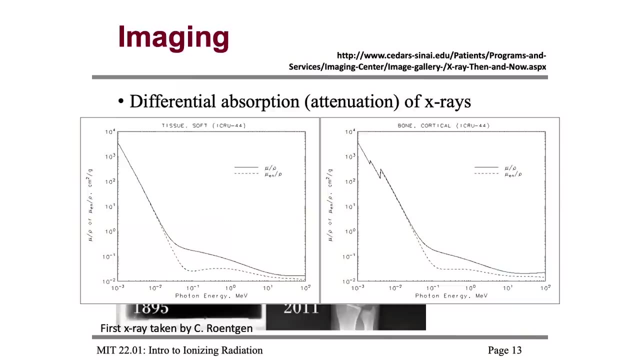 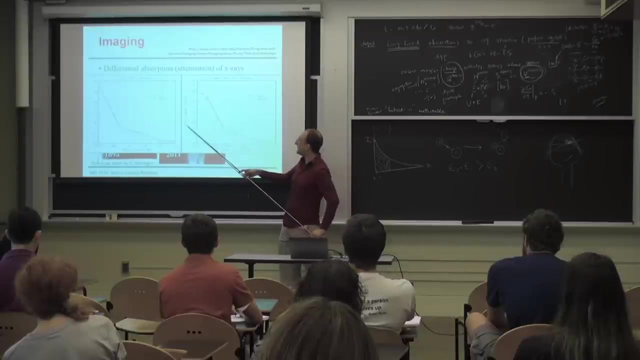 through different types of matter, And so, for example, here we have the ICRU standardized average, soft tissue attenuation as well as bone, And you notice that there's a few differences in these curves, So also there's some similarities. I'll note that these actually have the same axis. 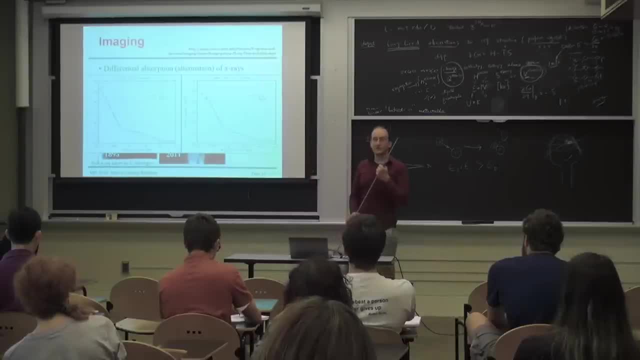 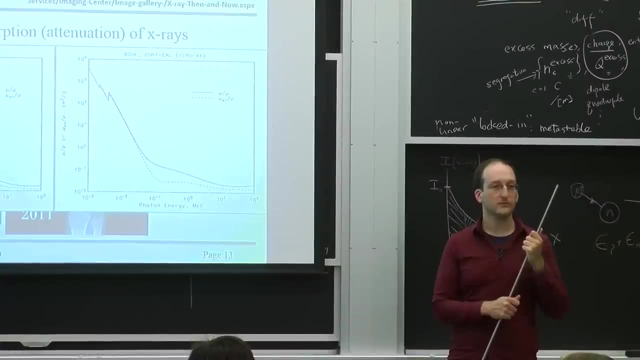 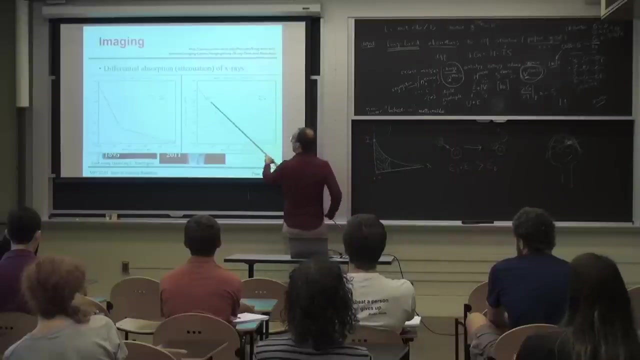 and the same units. What do you guys notice? that's the same about these curves. How about the value? They're basically the same mass averaged with very little differences If you look at where it hits the y-axis- about 3 times 10. 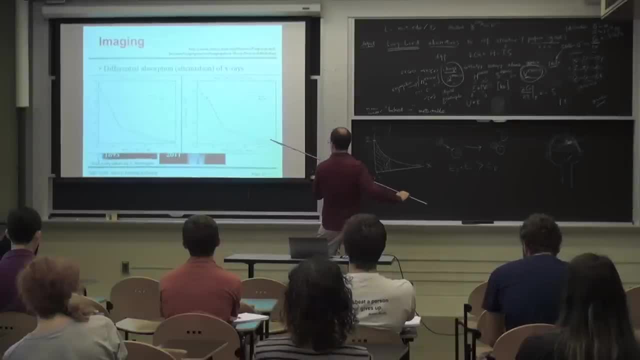 to the third, 3 times 10 to the third. The curves follow basically the same shape. What's the differences? So, Sean, what do you think? Oh, that little jagged one out there- MICHAEL SHORTLAND- These jagged edges right here. 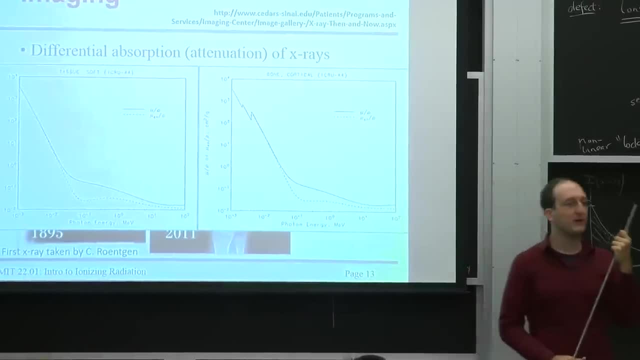 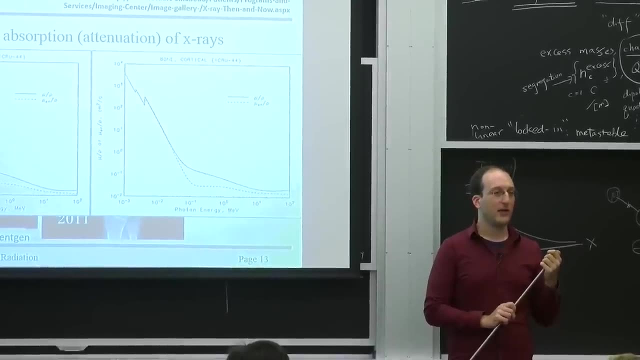 Anyone have any idea why? And these reasons go back to what you learned in high school in 802, in terms of atomic transitions, not nuclear. Anyone here remember the k-lines or the l-lines Or the- what was it? The which? 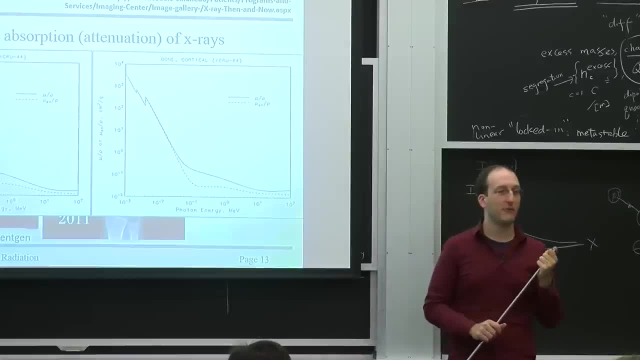 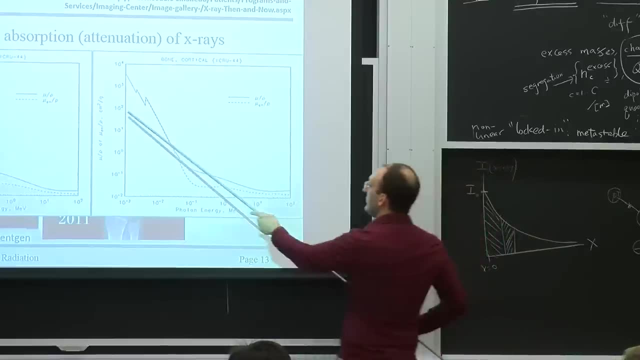 Emission series, what are they called? The different emission lines that you can get from emission or absorption spectra? It all has to do with allowable electron transitions And notice, the units here are in centimeters squared per gram. What's the main difference between soft tissue and bone? 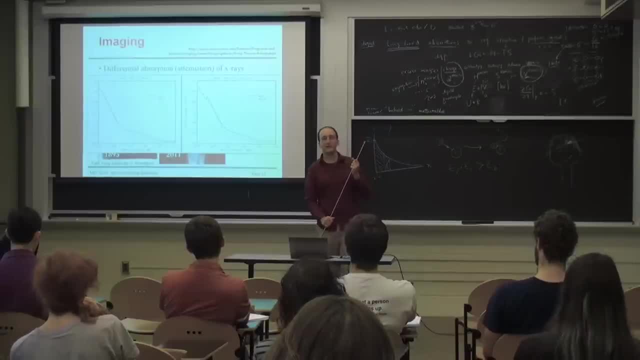 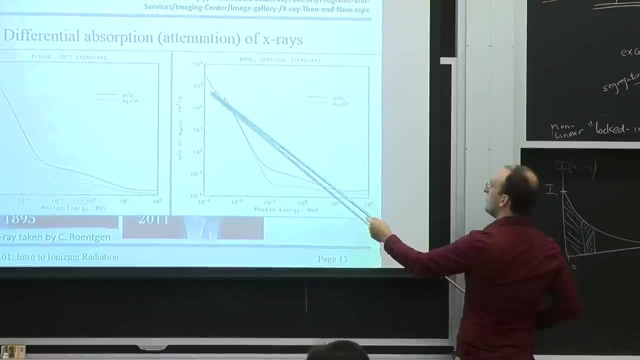 Say it loud enough so I can hear Density: Bone tends to be a fair bit denser than soft tissue. So these are mass out. what is it? Mass, normalized curves. But the fact is, if you have bone that has a higher density, 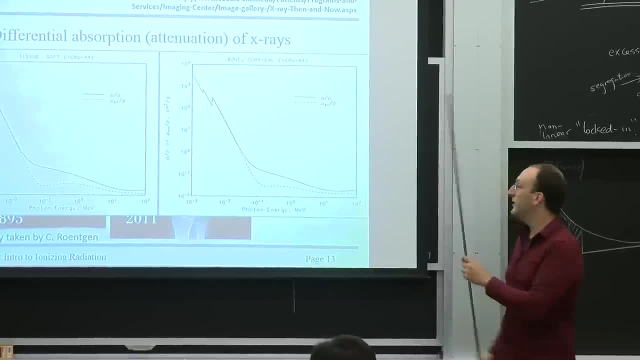 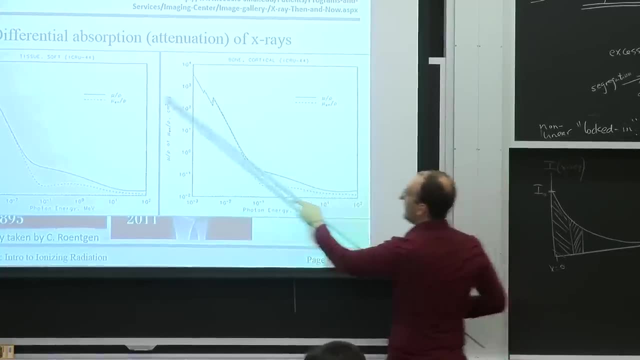 then you're going to end up with more absorption. In addition, you can use some of these features and differences to your advantage. Like, if you choose a photon with energy here, it might not be nearly as absorbing in soft tissue as it would in bone. 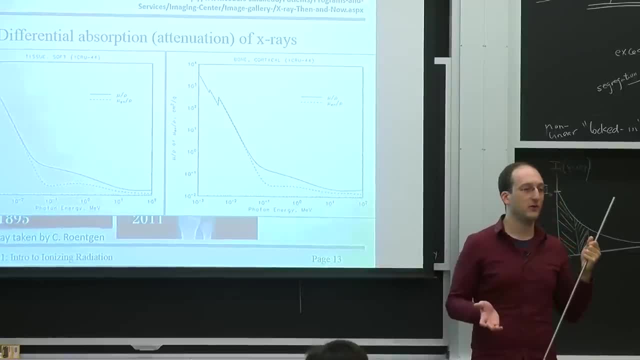 So by selecting the mass of the thing you're trying to image, which you don't control, and the energy of the photon, which you can control, you can produce as much possible, as much contrast as you can between two different things. 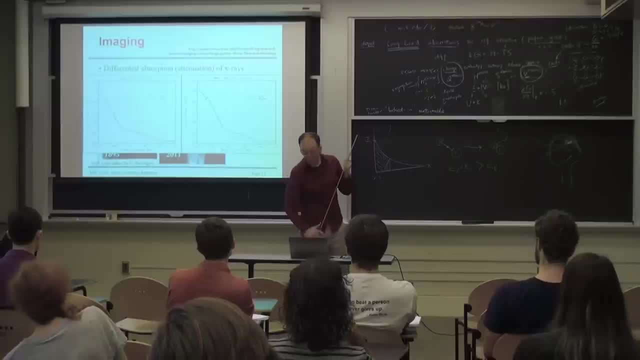 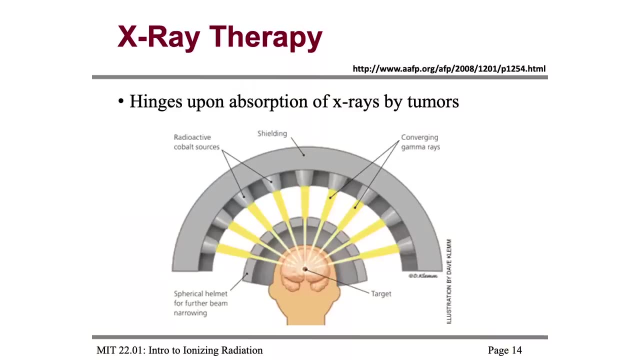 Is everyone clear on how that could work? Cool, We'll be going over why the curves has these shapes, especially these jagged edges, pretty soon. And, like you said, this is how you irradiate a tumor with X-rays, because you can't quite. 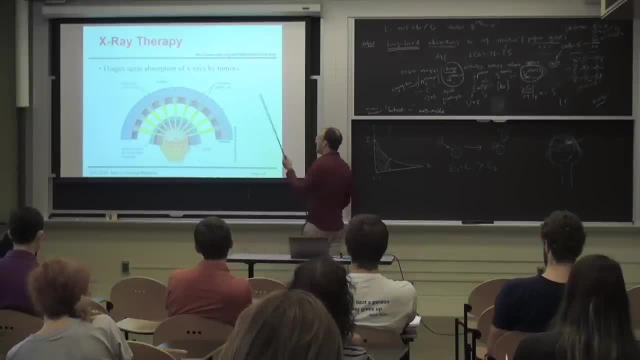 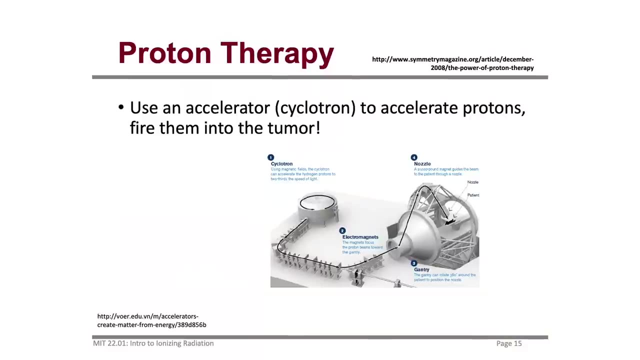 control the amount of dose to any one part, unless you split it up into a whole bunch of different rays. Proton therapy is quite different. It's a newer technology And it relies on very well-known and distinct ranges of charged particles to enter the body with very little. 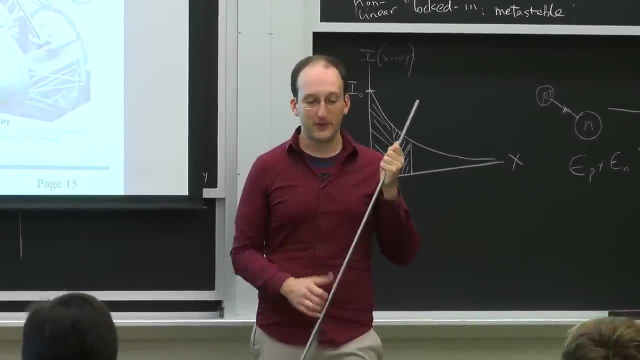 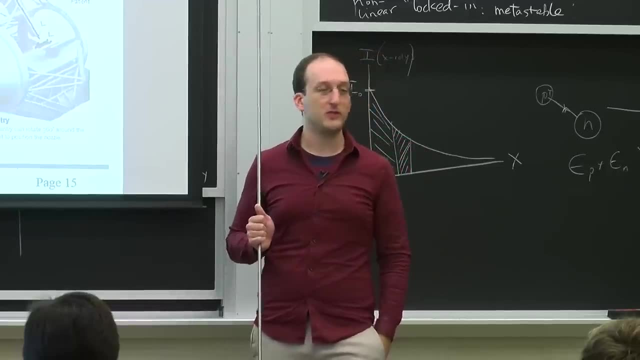 damage. stop and do their damage in the tumor and not come out the other side. They just require significantly more expensive hardware. There's one of these at Mass General Hospital or MGH down the road. It consists of a cyclotron or a particle accelerator. 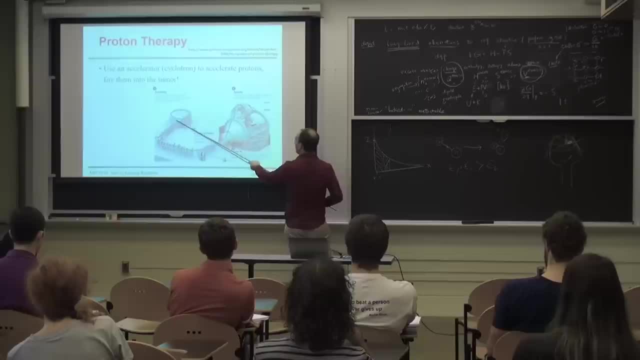 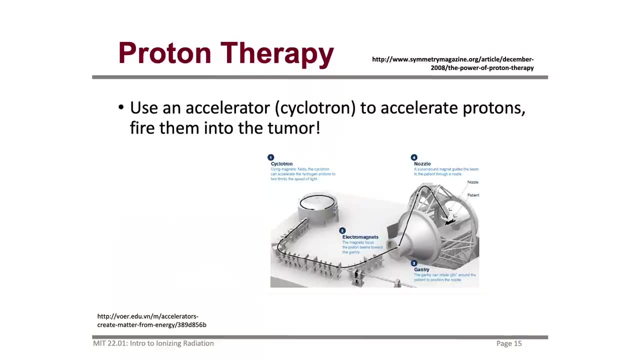 which injects and speeds up protons so that they're moving very fast, then sends it in a beam through a bunch of bending magnets and up to deliver The protons to the patient. The way this works is you start injecting the beam. 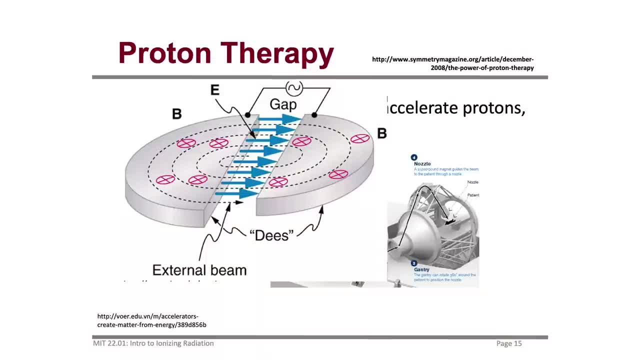 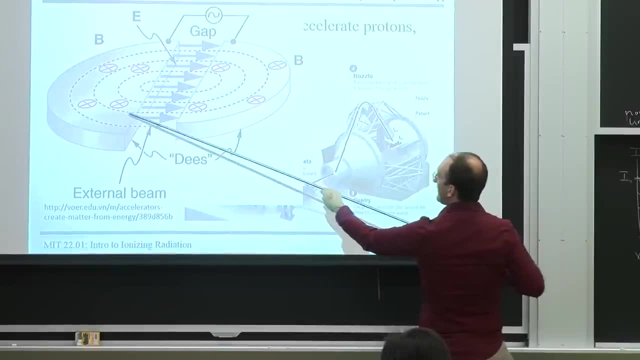 And as it goes through these two magnets, or what's called Ds, every time it moves through the magnet it's a charged particle in a magnetic field. It has a fixed curvature, But every time it's accelerated through this electric field. 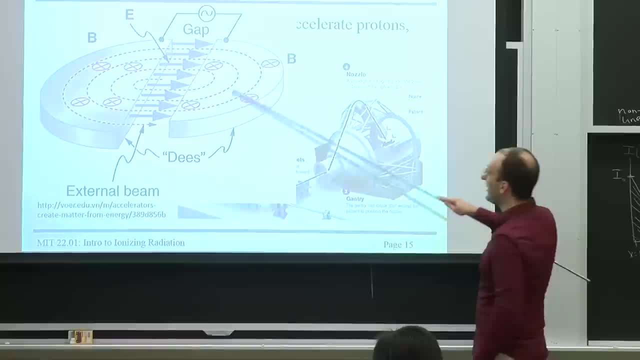 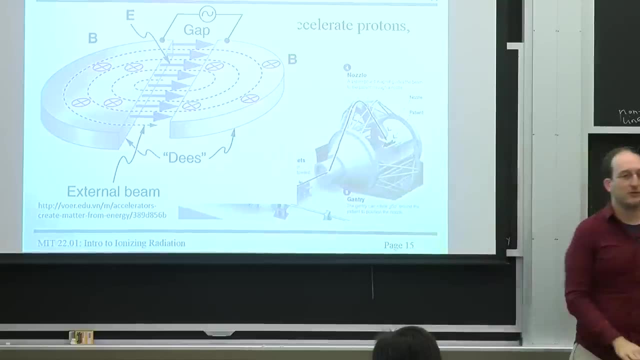 it speeds up, So the curvature gets greater and greater and greater, And it spins outwards in a spiral until they exit the beam. And by deciding how long they get to spin, you get to choose the energy of the protons. Why do proton therapy work? This has to do with the difference in interaction between charged particles and photons which have no charge. Charged particles will lose their energy in a very well-known way- what's called a stopping power formula, until they actually stop in the matter that they are going through. 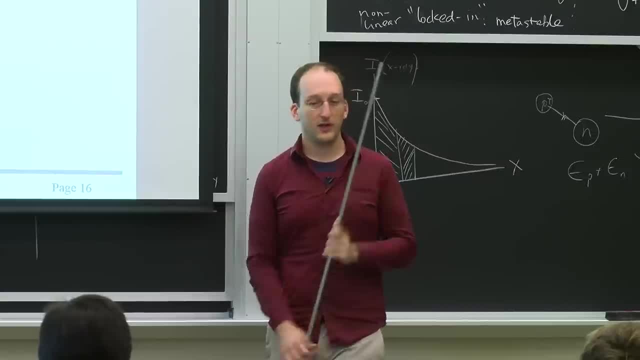 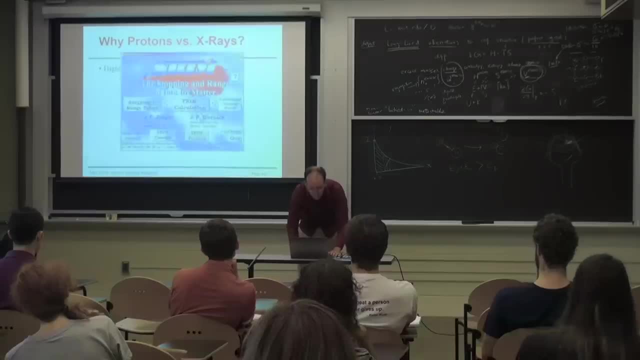 Photons either scatter or attenuate or they don't, And you can't stop them all. So I want to run a quick Monte Carlo simulation for you guys and show you what proton stopping in matter looks like. So this is a program called SRM, or the Stopping Range. 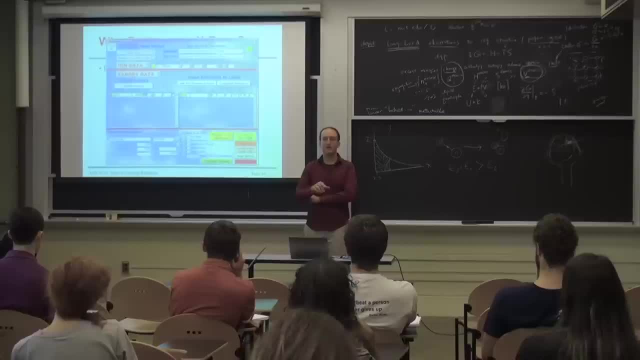 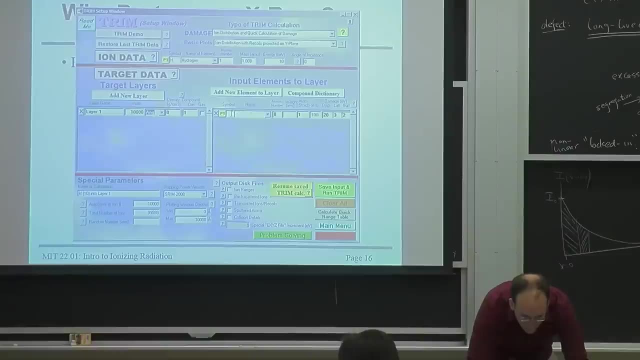 of Ions in Matter. It uses the formulas that we'll be deriving and developing in this class to calculate the trajectory of protons in anything. So let's say you are made basically of water. So let's say you consist of hydrogen and oxygen. 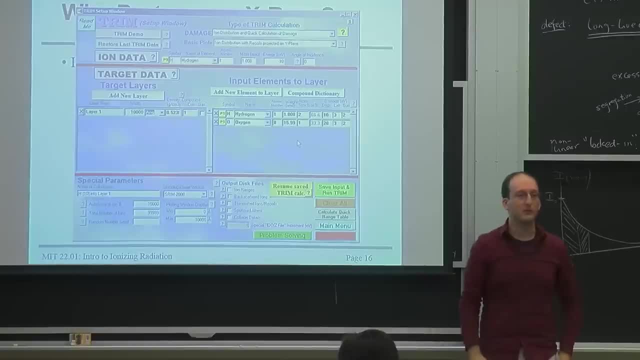 in a stoichiometric ratio of 2 to 1.. I think water approximates humans pretty well, So we'll find out what the range of these actual protons is in humans. So what we do know is that it's a proton accelerator. 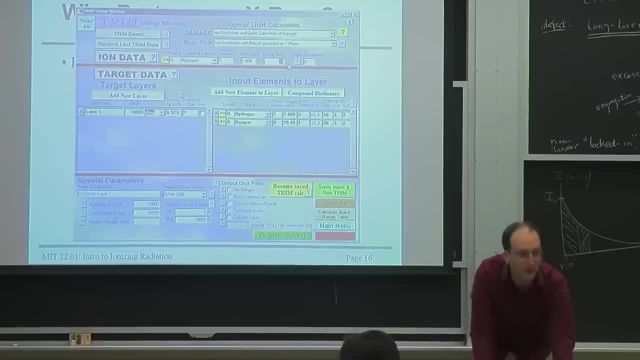 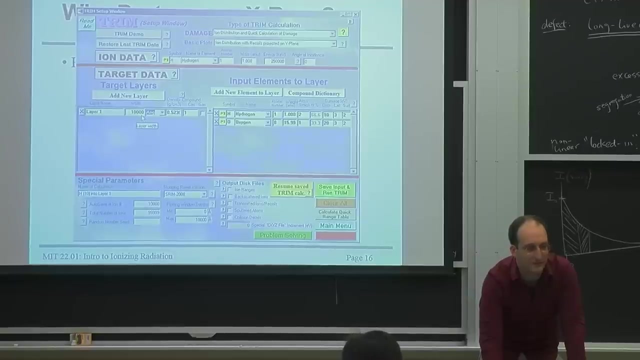 And I know that the MGH accelerator has an energy of 250 MeV or 250,000 kiloelectron volts, And finally we decide how thick is the person. So how thick is a person typically? How many? what units do we get? 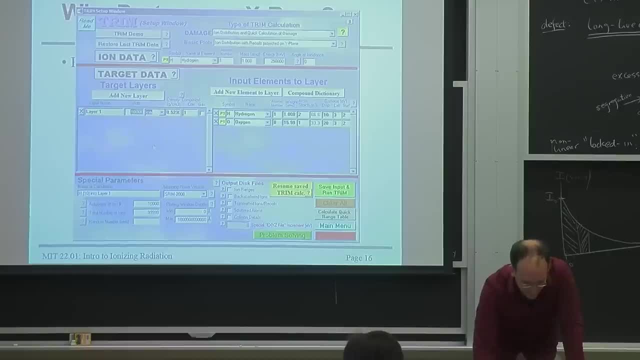 How many centimeters thick is the average person? Let's go the shortest distance in, So front to back, maybe 10, right, 10 centimeters, about that much They get halfway through. you Only has to go halfway because you can always. 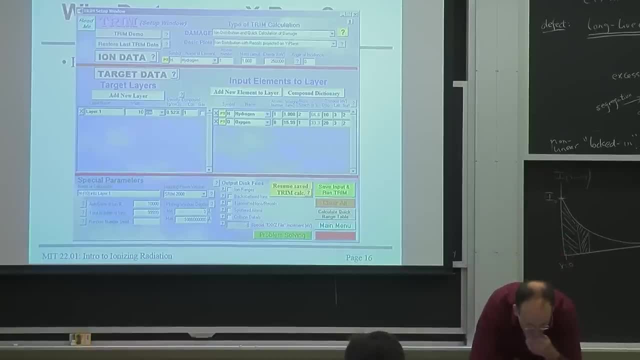 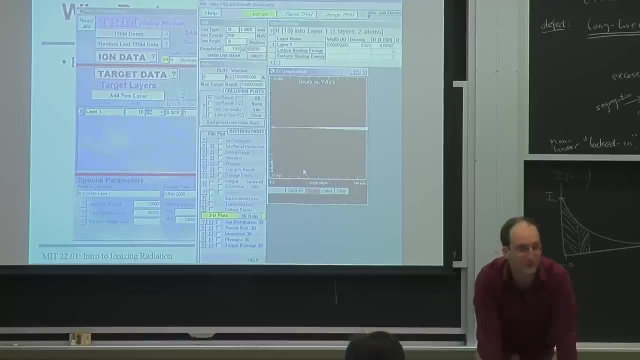 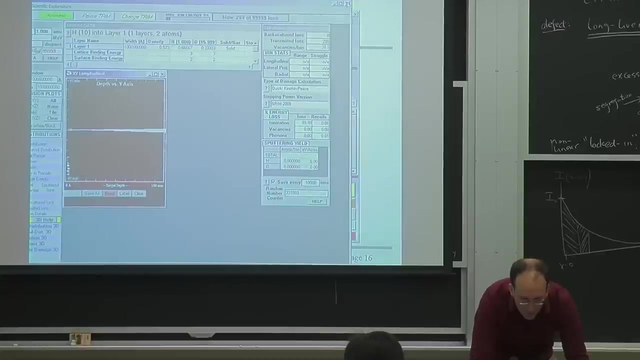 lie on your stomach. All right, Let's go 10 centimeters. Most of the protons go screaming right through. You notice they don't actually stop in the person, So you don't tend to irradiate people with 250 MeV protons. 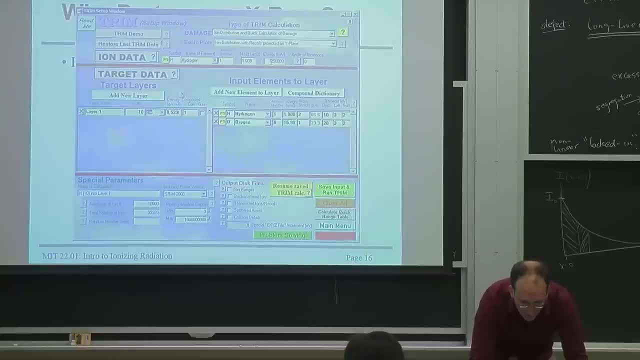 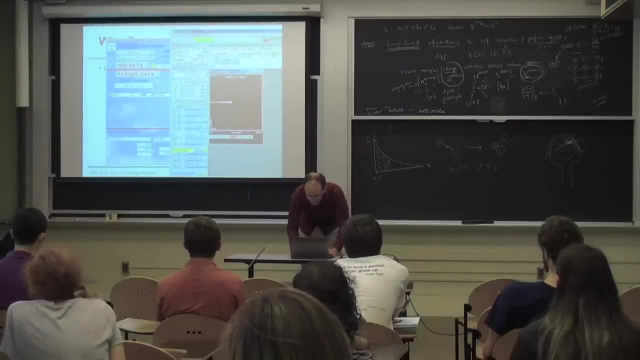 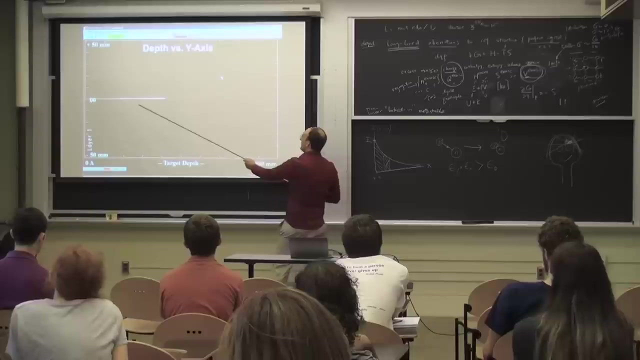 directly, You'll actually slow down their energy to something a little more reasonable, maybe 50 MeV, And then you can actually watch each of these charged particle tracks being computed As it hits, let's say, imaginary nuclei or electrons. the paths will be slightly deflected. 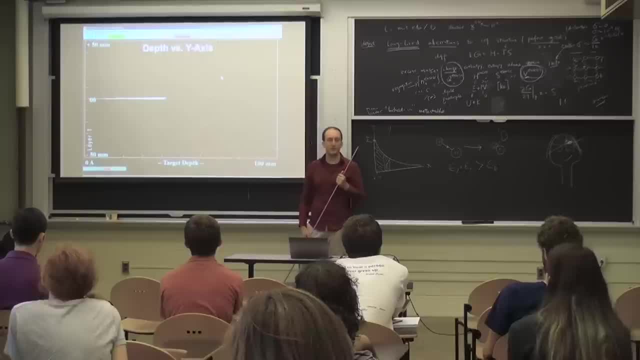 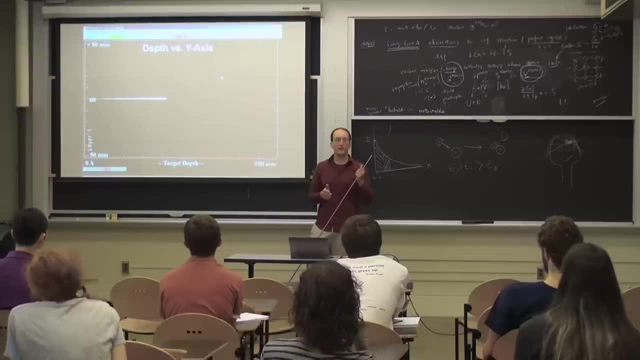 But what's really striking is They all tend to stop at about the same place. That's the really cool thing about charged particle interactions is if you know the charge, you know the nucleus, you know the energy, you can calculate the range. 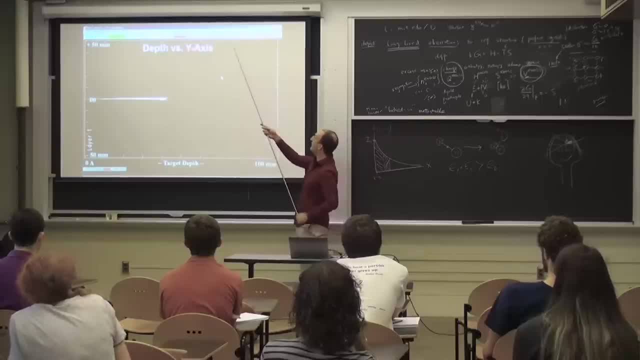 to within a very narrow margin, And what this is doing is just flying. Looks like it's done 70 ions so far And it will keep on flying them until either you hit the end. Let's say we set it to do 100,000 atoms. 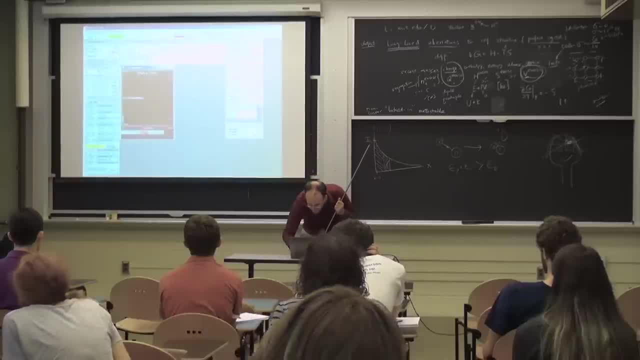 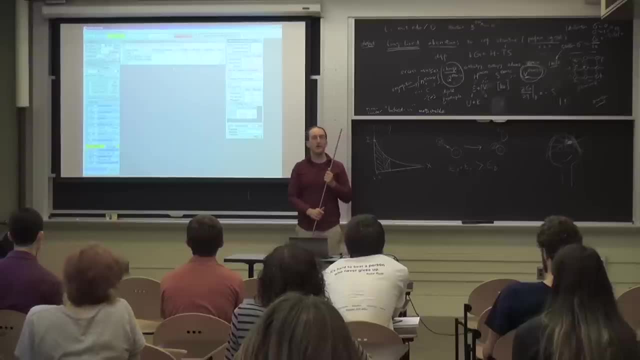 or you just tell it to stop. Also, when you don't have to draw the lines, it goes way, way faster. So let's let it get maybe 300 or 400 ions And we'll show you what the average range of the protons. 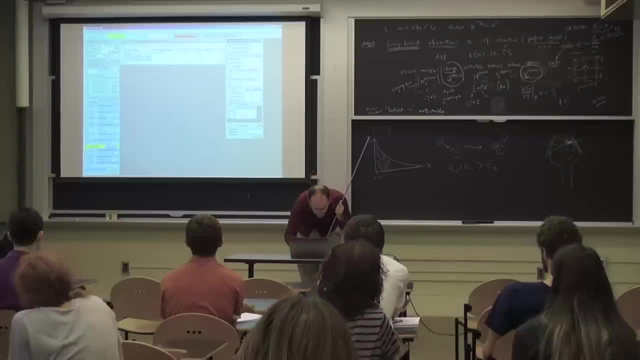 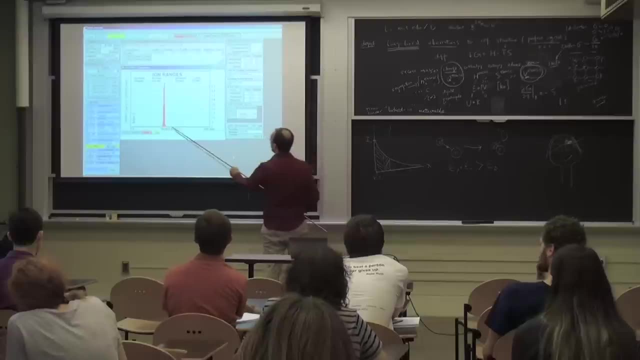 looks like. How far do they go before they stop? If we look at the ion distribution, it's pretty striking. All of the protons, except it looks like one of them stopped at a very fixed depth of 41.9 millimeters. 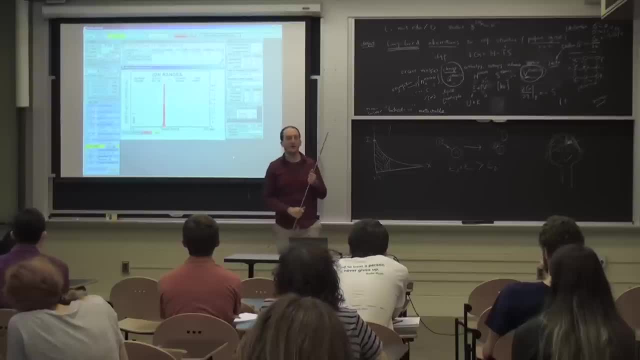 with very little straggle, maybe 0.6 millimeters on either side. So, depending on the depth of the, You can even get a deep, very shallow, very small tumor if you get the distance just right and the proton energy just right. 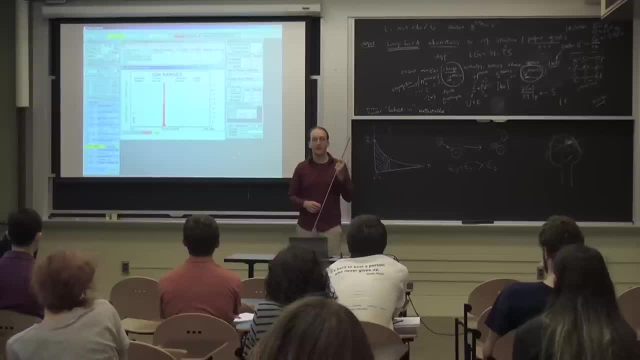 This is why proton therapy centers are popping up all over the world. This is a much more effective, though expensive, treatment for certain types of tumors. At the same time, since we're nuclear engineers, we may be concerned with the amount of radiation damage. 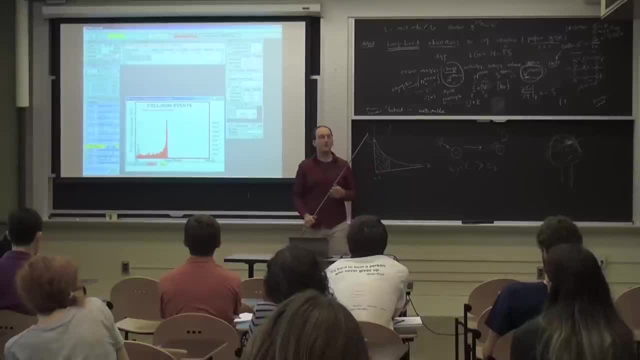 being done to different materials, And so this is kind of a measure of how much energy the protons are losing as they travel through Notice it's not zero. As soon as the protons enter the person, they start to scatter around undergoing. some different interactions, But they mostly don't lose much energy until they reach almost their target depth, And what's called the stopping power is very low at high energies, very high at low energies, which means once they get slow enough, they almost all stop right there at what's. 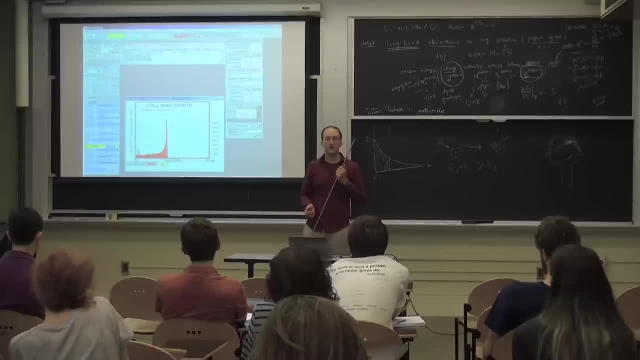 called the Bragg peak, And that's the basis behind proton therapy, And you'll be able to understand why every feature of this curve looks the way it does by the end of this course, probably by the end of this month. So let me stop that simulation, because we really 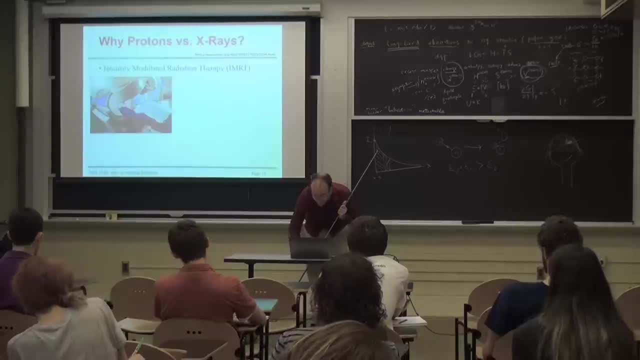 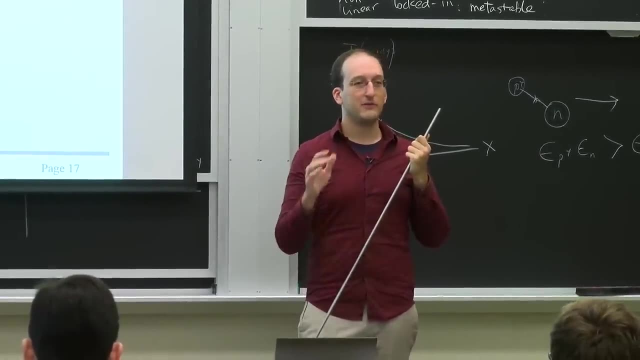 could go on forever, but we won't. Then the question is, what do you do if the tumor is too big? If the tumor is larger than that straggling, you actually have to sweep the energy of the proton beam So you can vary the energy continuously. 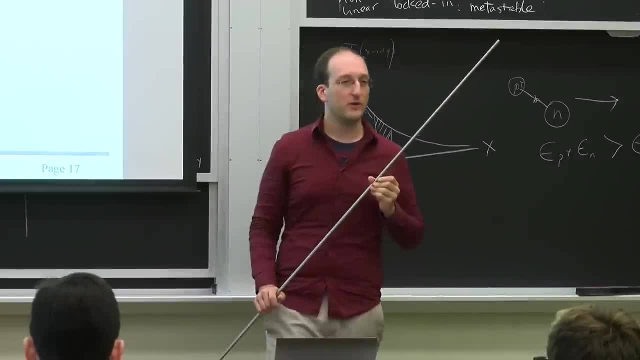 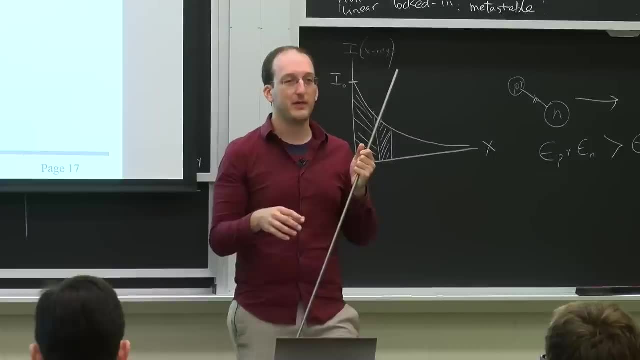 in what's called intensity-modulated radiation therapy, where you change the energy of the proton, sweep it back and forth across the tumor to cover the whole thing, so you can sweep out in 3D space the size of whatever you want to die without affecting the stuff that you. 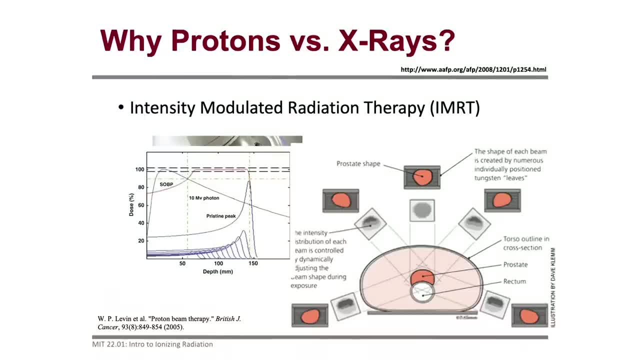 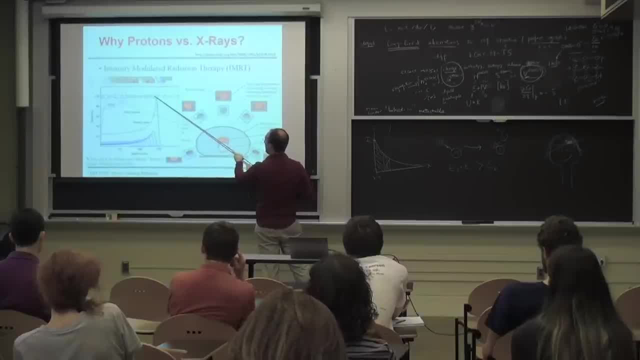 don't want to die. So in this case, let's say you'll apply protons of a certain energy for some point, and then another energy, then another energy, And you can maximize the dose to a pretty flat level while minimizing the rest of the dose to the patient. 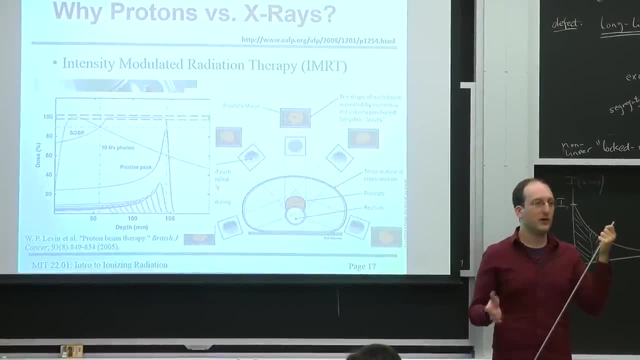 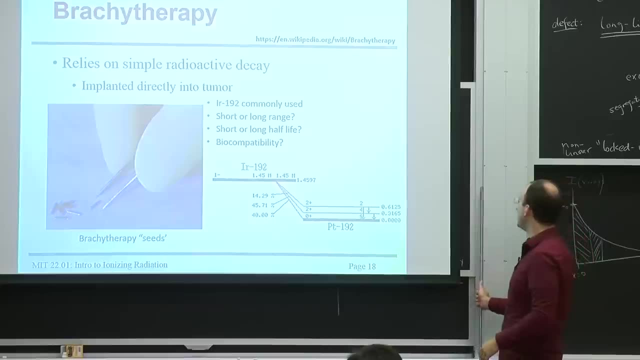 So, even while changing energies, the most dose is done to the tumor and as little as possible is done to the rest of the person. We already talked about brachytherapy, but we didn't say why it works. This is the first major topic we'll 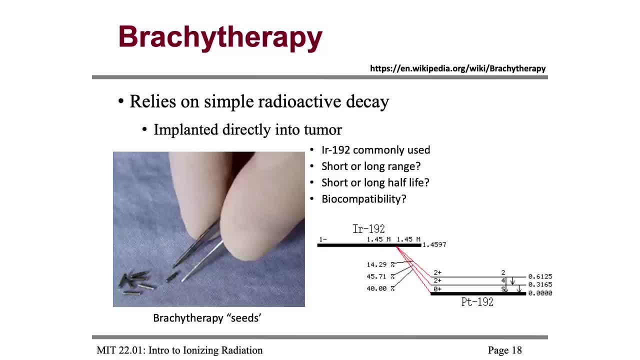 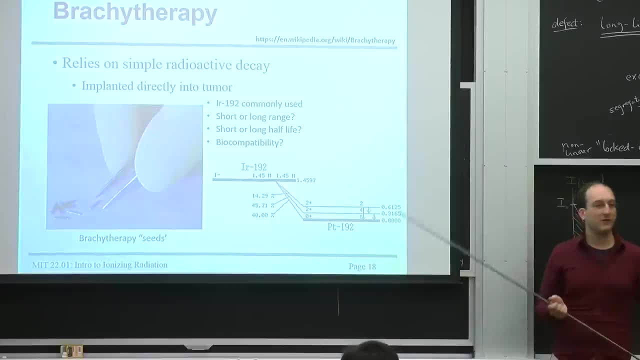 be talking about in this course. It relies on natural radioactive decay, And for natural radioactive decay you need to understand decay diagrams, which are energy-level diagrams of which isotopes turn into which others, by which methods and how much energy they release in each type of decay. 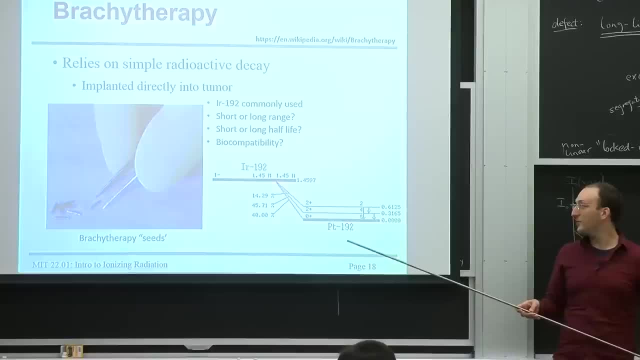 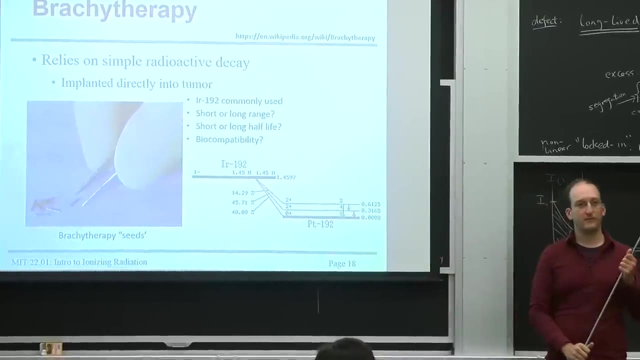 So, for example, a common run is iridium-192.. A pretty biocompatible isotope, because it's well, it's like a noble metal. And iridium-192 can decay by one of three pathways and become platinum-192, gaining a proton. 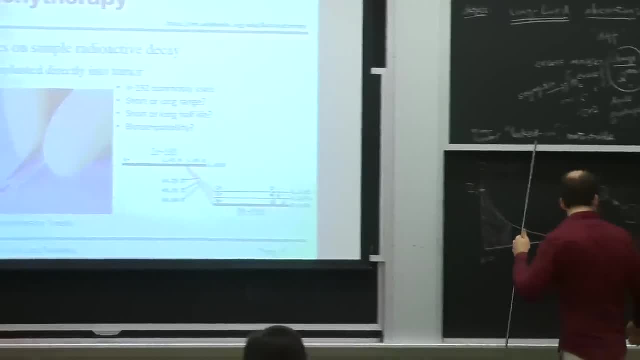 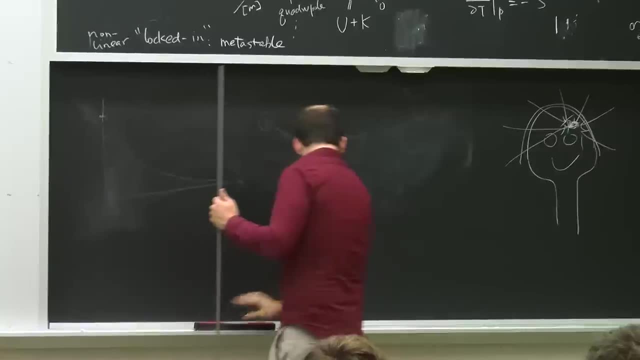 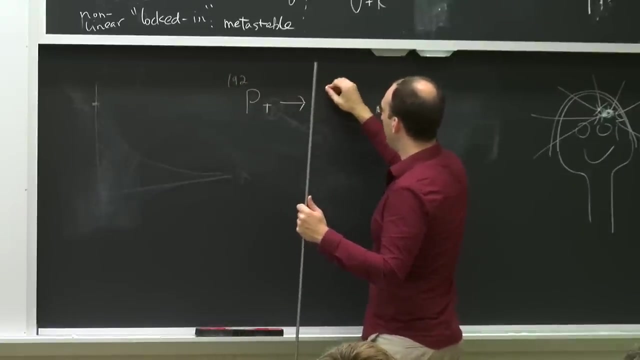 Gaining a proton. What has to happen for that to be conserved? So let's think about this. Let's say we have platinum-192.. Let's say we have platinum-192.. Let's say we have platinum-192.. Which decays naturally into iridium-192.. 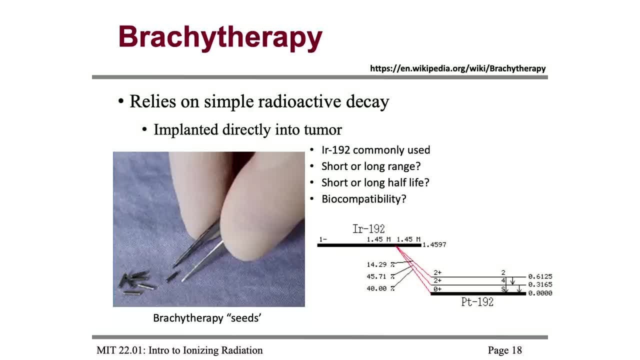 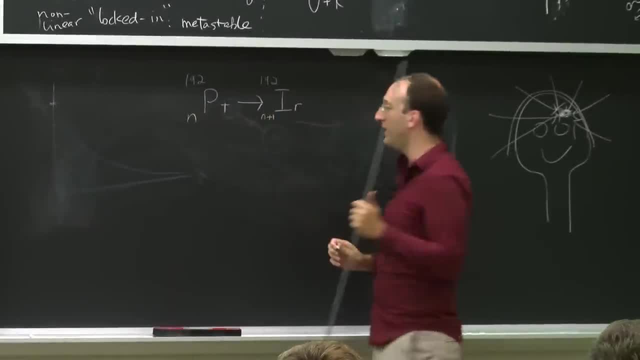 I can tell you because we've drawn the diagram to the right, it's going up one atomic number. So let's just say that it had n protons and it now has n plus 1. How do we balance this nuclear reaction? 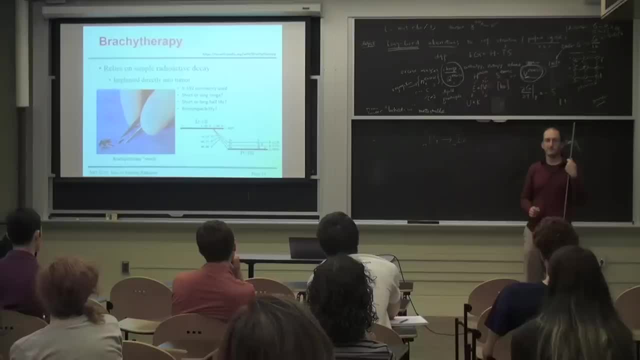 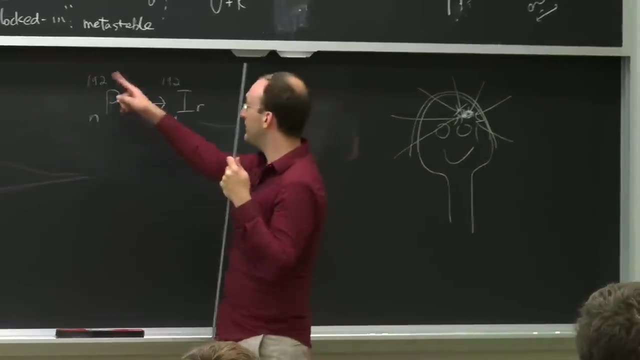 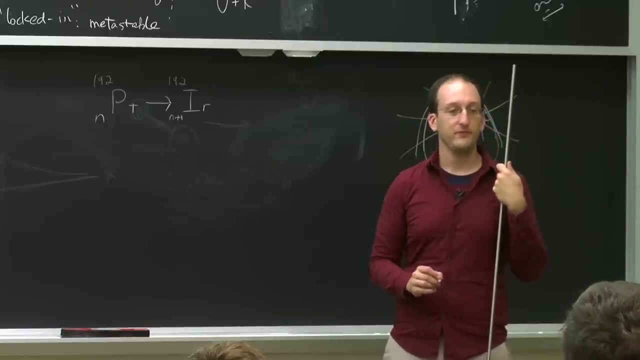 What are we missing? Yep, The neutron turns into a proton. OK, so there's a neutron somewhere, There's a number in this nucleus that turns into a proton. What are the things that we have to conserve in any nuclear reaction? Yep. 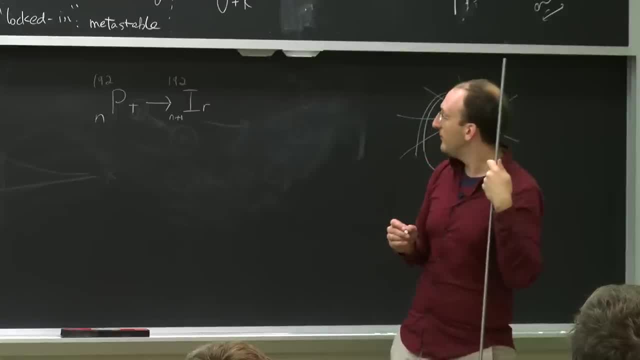 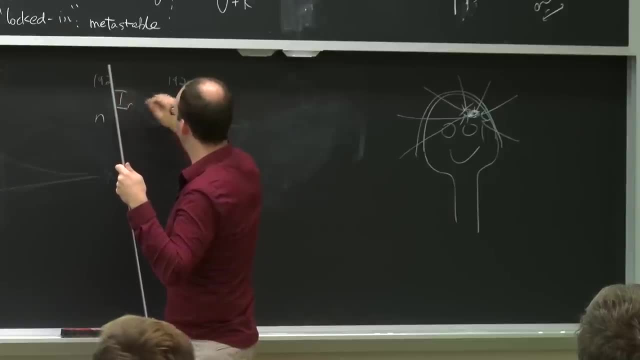 Just a question: Doesn't it go from iridium to platinum-192?? Yes, thank you, I got that backwards, But the numbers are right. The symbols are wrong, Something else I'll mention about this class. Please do stay on your toes to correct silly things like that. 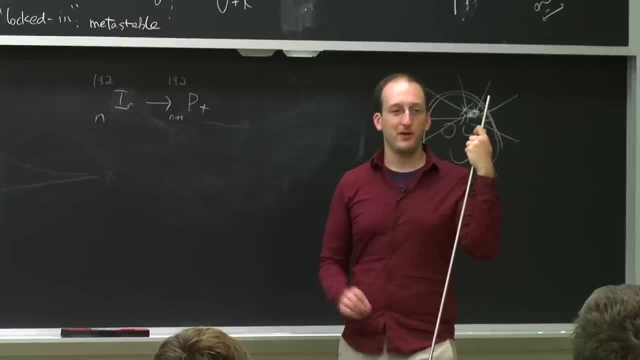 I don't do scripts because you didn't come here to see me read off a piece of paper. Everything's live, All the derivations are going to be live, because it's more interesting- certainly more interesting- for me to teach. So thank you for catching that. 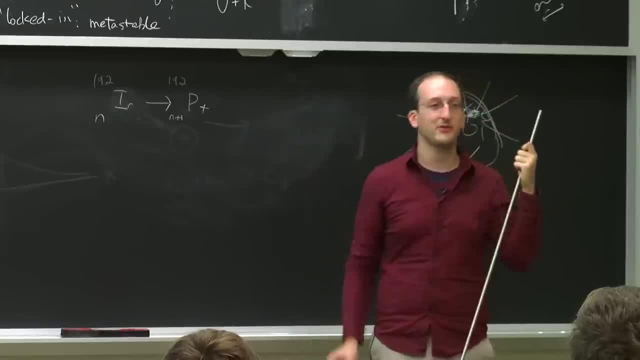 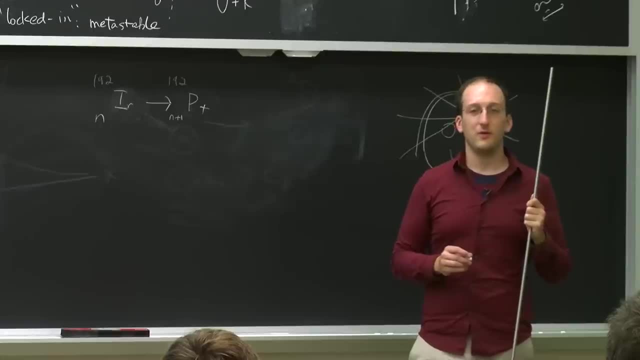 And please do stay on your toes if you see something silly, especially if it's just not the same as on the screen. So, like Luke said, we made a proton, or a neutron turned into a proton, What's not conserved in this reaction. 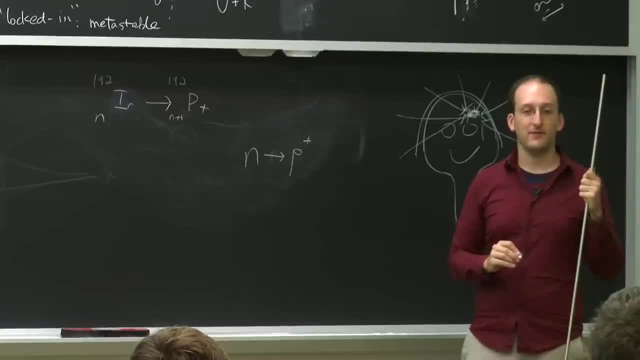 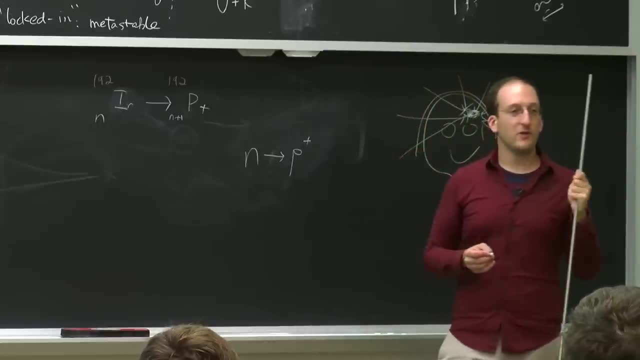 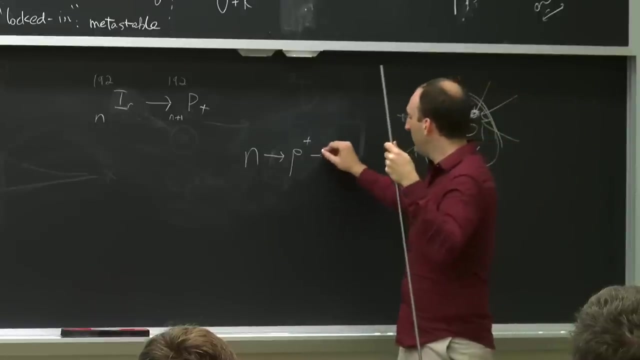 Yep, Charge, Charge. How do we balance that? Well, let's add some other particles. There's got to be some sort of radioactive decay. So what are our choices of particles? Yep, Sure, an electron, or more specifically, 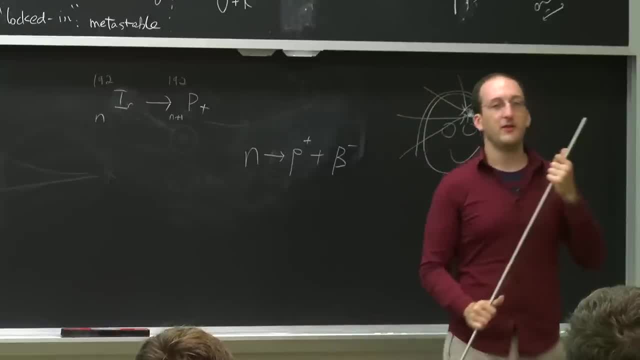 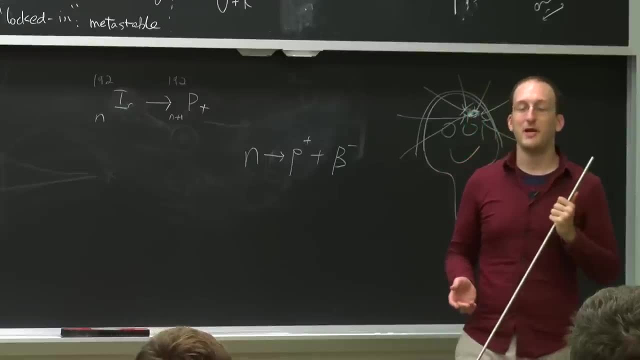 we'll call it a beta particle. Just like a gamma ray is a photon that originates in the nucleus, a beta particle is an electron that originates in a nucleus. You can't tell it's a beta particle just by looking at it. An electron's an electron. 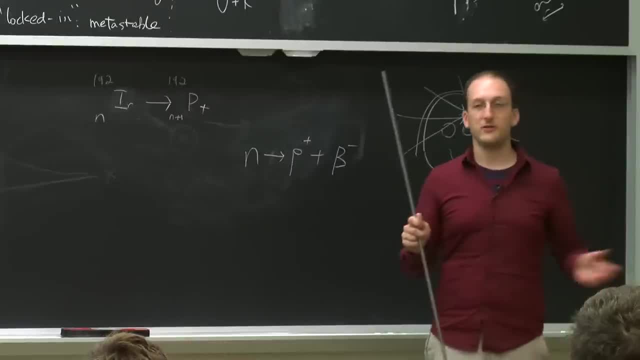 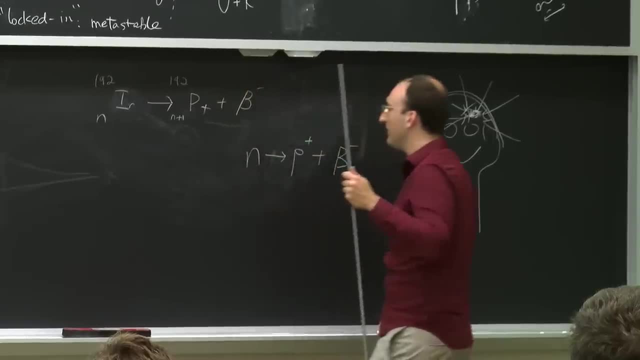 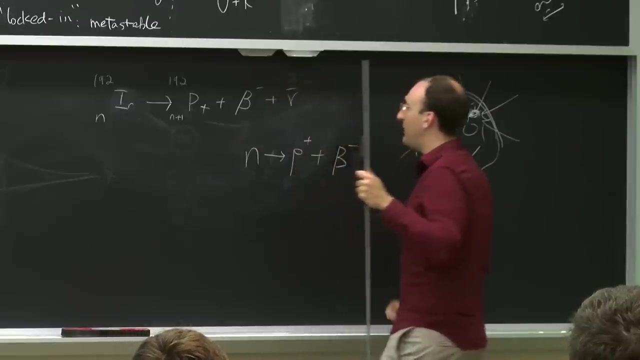 The only way you'd know is either by its energy or because there are another source of electrons nearby. So in this case we get beta decay. This looks fairly balanced. One thing that I'll put in is beta decay is accompanied by an antineutrino. 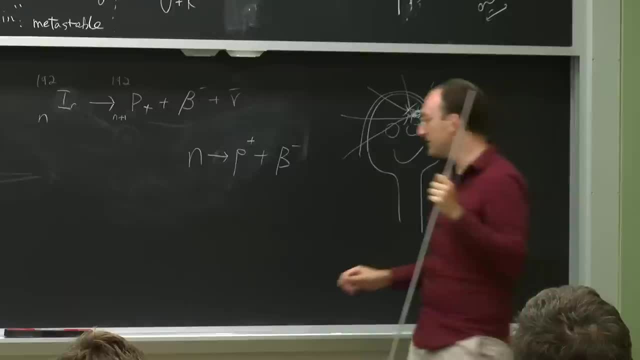 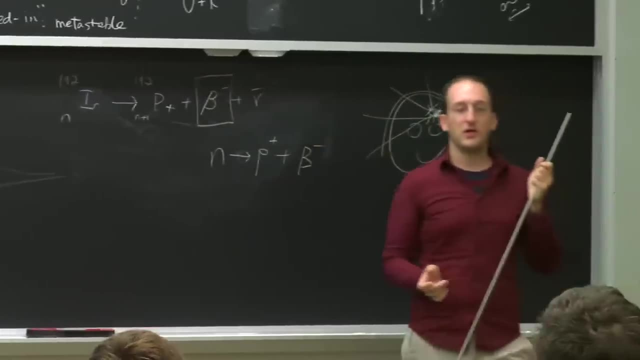 but I did not expect anyone to know that. I just want to make sure it's up there for completeness. So what we're relying on, It's the movement of these electrons, which are high charge and low mass, which means they're very low range, which 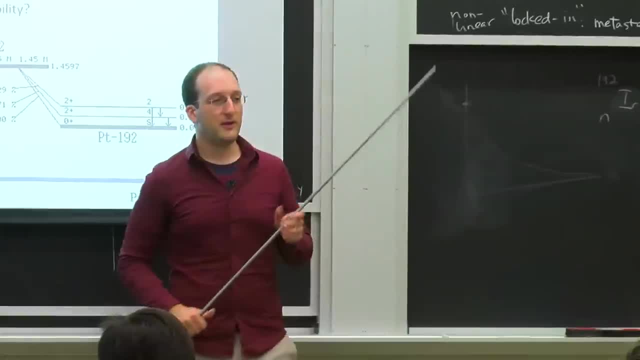 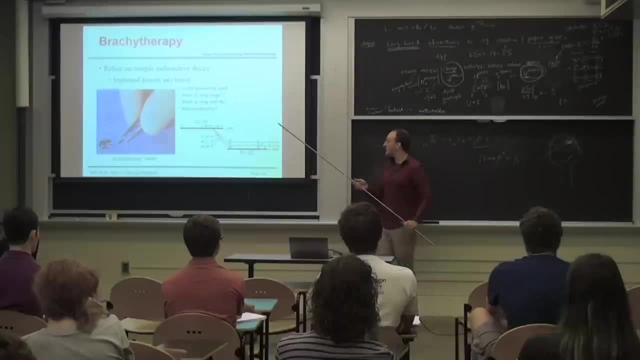 means when you implant a brachytherapy seed into a person, the irradiation volume is only as large as the energy of that beta particle will allow. The maximum energies for these beta particles are given by the differences between the starting and the ending energy. 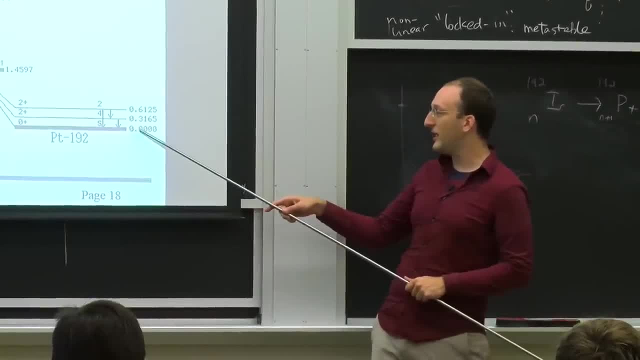 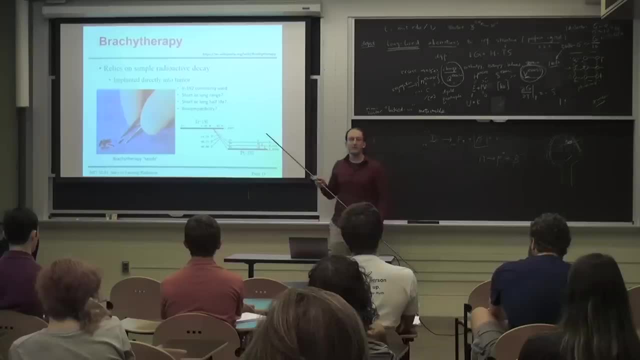 The way these diagrams are constructed is your ending energy usually has an energy of 0,, which we refer to as the ground state of that isotope, And all of these are relative energies in MeV or mega electron volts. So, for example, this iridium-192 has a 40% chance. 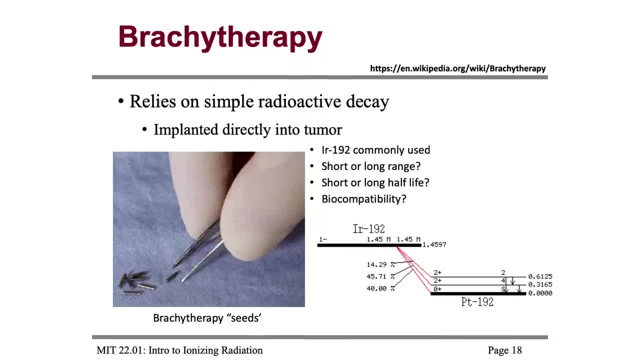 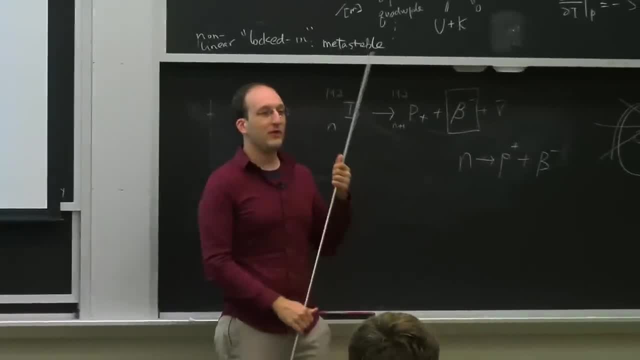 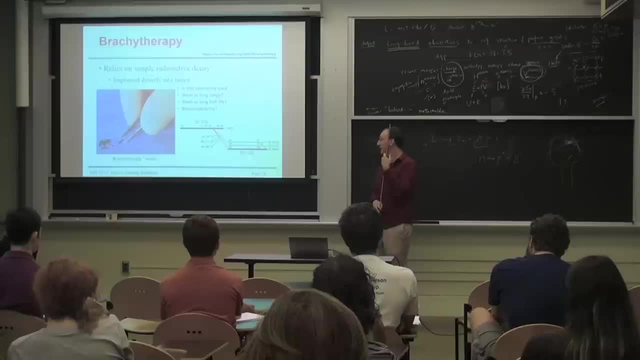 of decaying by beta to platinum-192,, which means the electron can have up to 1.4597 MeV, And if we know its energy we know its maximum range. So selecting the right isotope and the right activity for the right tumor is quite important. Notice that there's also other ways in which this thing can decay. It might release a beta particle of a lower energy and reach what's called an excited state of platinum-192, which can then decay by just giving off this extra 612 keV of energy to the ground state. 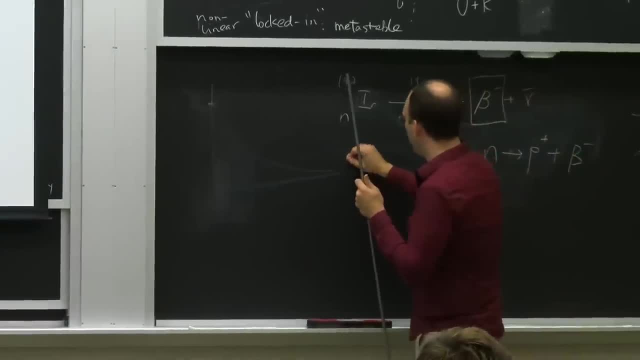 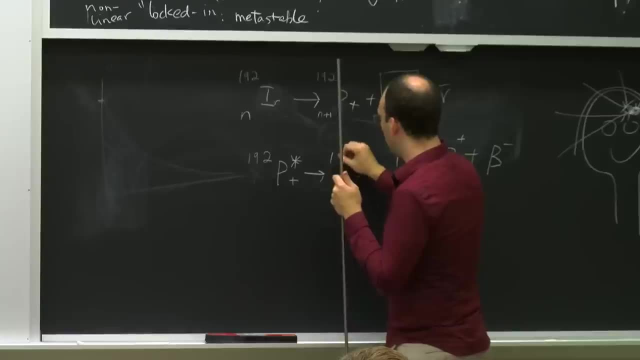 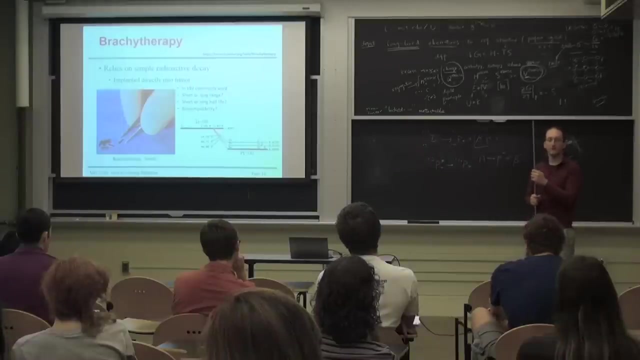 So let's write that nuclear reaction. Let's say we have platinum-192.. And I'll put a star to mention that it's excited. It becomes platinum-192.. Where'd the energy go? Gamma MICHAEL SHORTENBERG- Gamma. 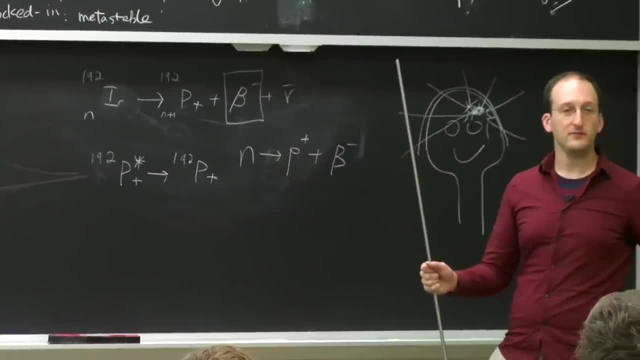 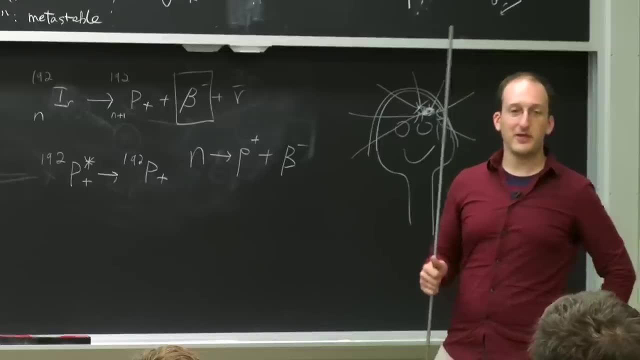 So why do you say a gamma ray? Because that just seems to be the biggest source of energy that's released in a reaction like this. MICHAEL SHORTENBERG- So you said it's because it's the biggest source of energy that. 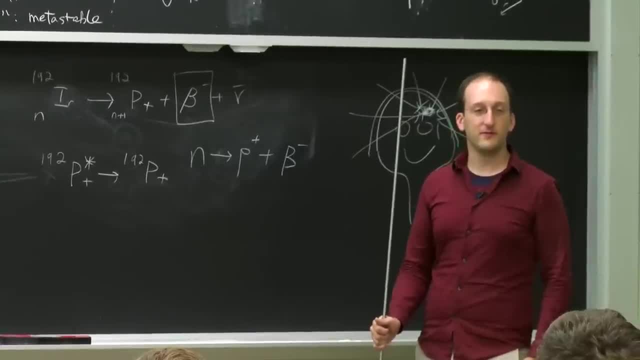 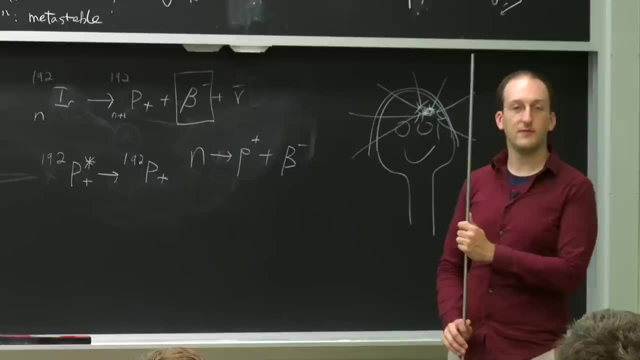 could be released. No, It just seems to be integratively. that makes sense. MICHAEL SHORTENBERG- OK, What do you think? Isn't it a thing where an electron loses, Or it drops at energy levels and releases a photon? 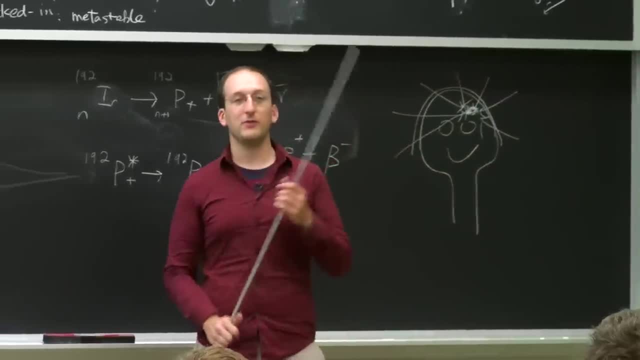 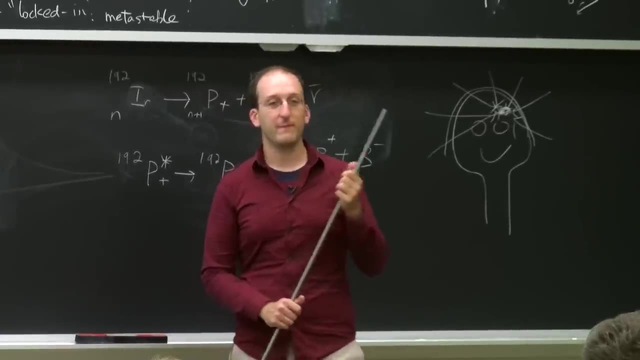 MICHAEL SHORTENBERG- Indeed, if an electron drops down at energy levels, it will release an x-ray or a photon, But that's not a gamma ray. It's not coming from the nucleus, Yep. So doesn't it have to be a gamma ray? 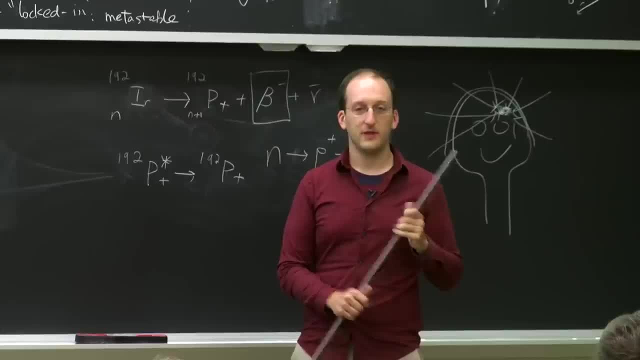 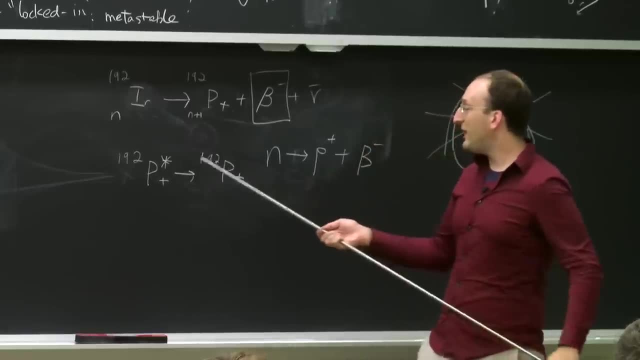 because that's the way to conserve mass. MICHAEL SHORTENBERG- Exactly So. the question with this is: what do we have to conserve Mass momentum energy charge? We have platinum-192 going to platinum-192.. 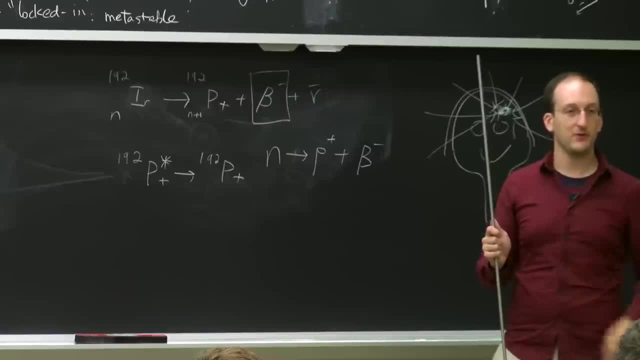 The mass is pre-conserved. MICHAEL SHORTENBERG- Yeah, Pretty much the same. Yep Question, Luke: What does it mean for platinum to be excited? MICHAEL SHORTENBERG- It means it's at a higher energy nuclear state. 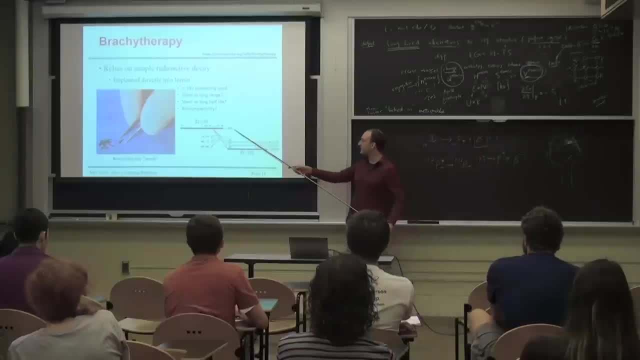 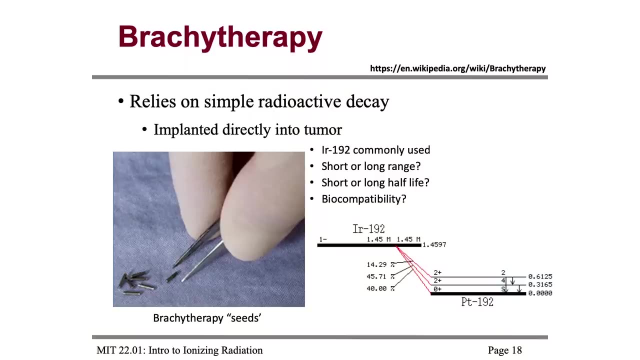 It means that there is excess energy in this nucleus. So the difference between ground state- or whatever- of iridium-192 and the ground state of platinum-192 is 1.4597 MeV. Notice, I'm not rounding, Don't round. 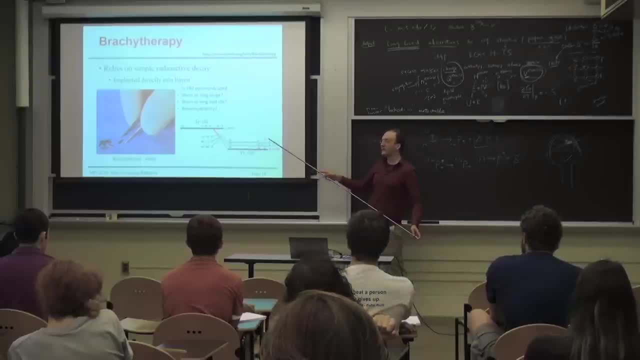 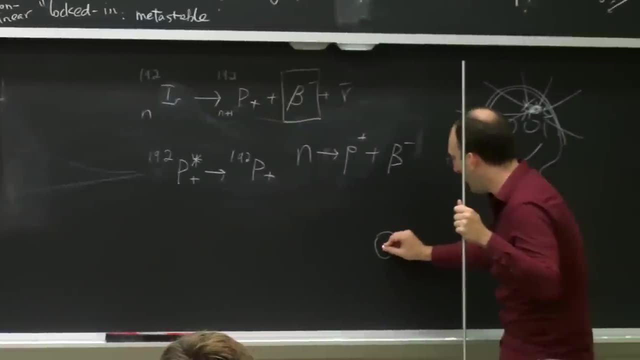 And we can end up with a beta particle that doesn't quite release all that energy, leaving some in the nucleus in what's called an excited state. It's analogous to if you have, let's say, an atom of A, whatever that happens to be. 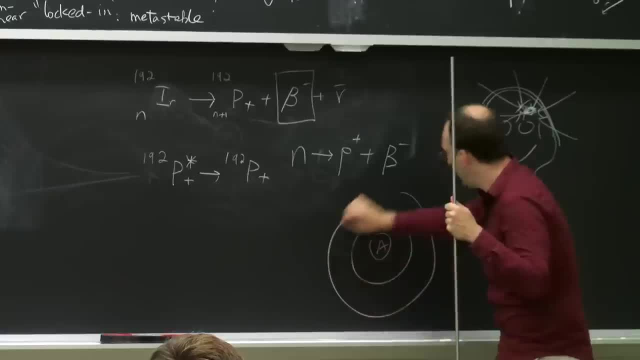 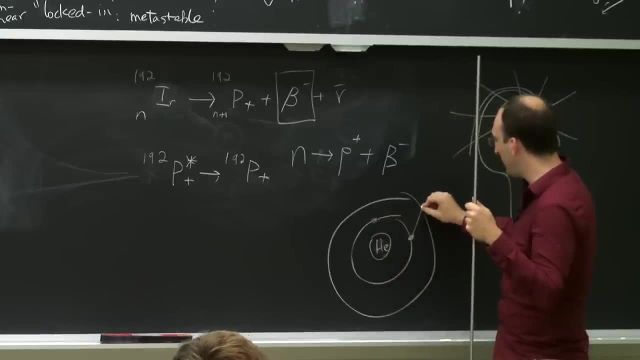 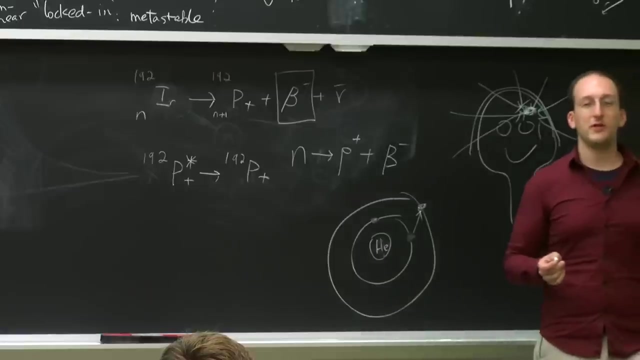 And since you started talking about different electron energy levels, maybe this atom is helium and it only has two electrons And one of them gains some energy becoming excited up to the next energy level. Same thing, but on the nuclear level. these excitations are not in the E-V range. 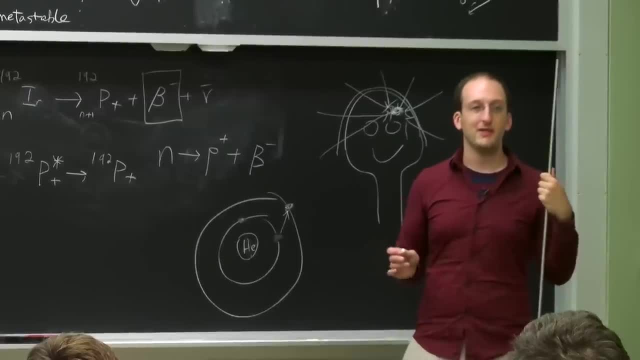 They're in the MeV range- MICHAEL SHORTENBERG- But you can think, if you're excited, you're excited. You can think of it as a precisely analogous process. for the time being, There are excited nuclear energy levels. 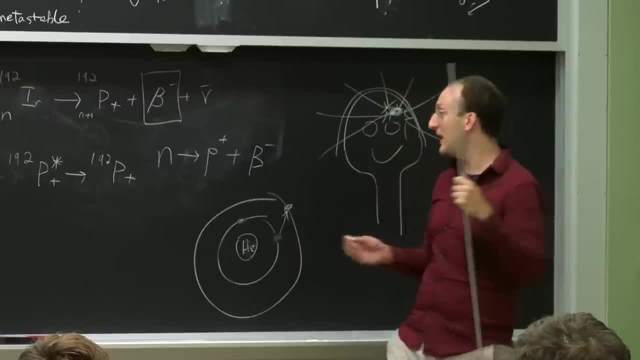 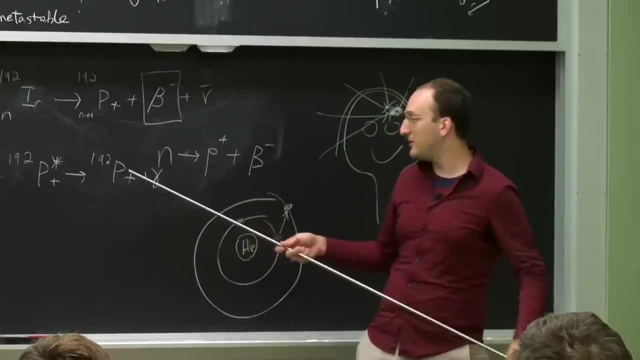 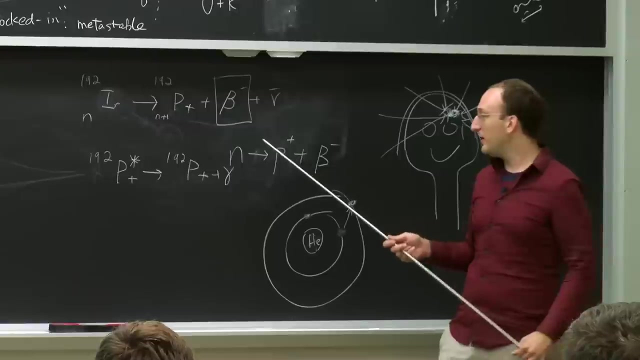 and they can also decay by photon emission, in this case gamma emission, because the masses are basically the same. Remember that the rest mass energies might be slightly different, but the charge is the same. There's no real change in momentum because this is a nucleus that started at rest. 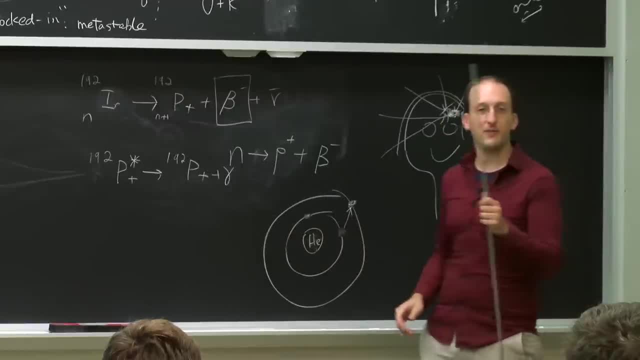 And this way the energy can be conserved. Yeah, Sean, In different cases. if there's very excited, can they just go through another decay process? MICHAEL SHORTENBERG- Absolutely. So there are multiple isomeric transitions or gamma rays. 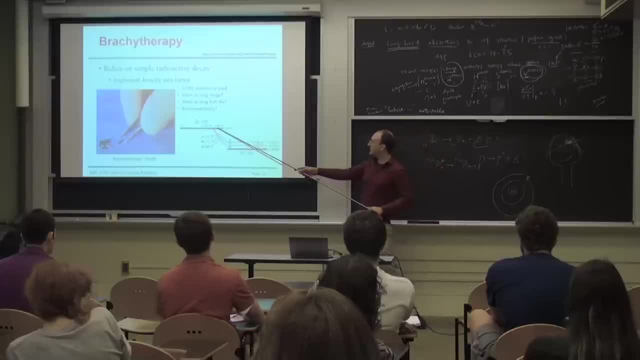 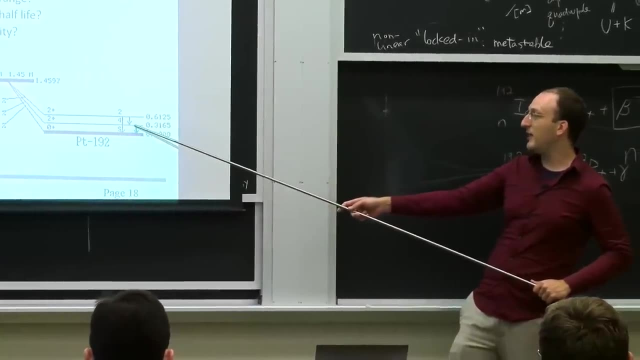 So let's chart one of the paths through here. There's a 14% chance that iridium decays to this excited state and it can then decay by a gamma ray to another excited state and then decay to ground. So there are lots of different possible pathways. 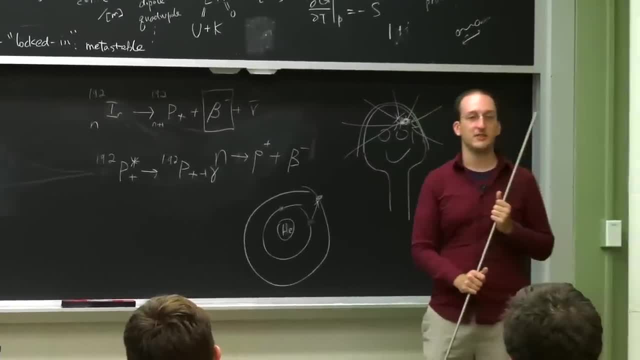 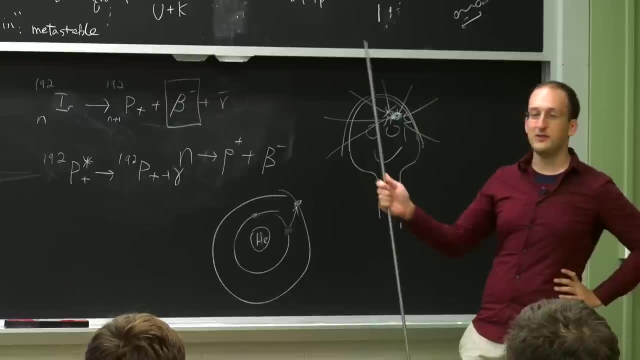 I've chosen a particularly simple isotope because it fits on the slide. In your homework you're going to get to look at the decaying diagram and you're going to see that there are not enough pixels in this projector for plutonium-239.. 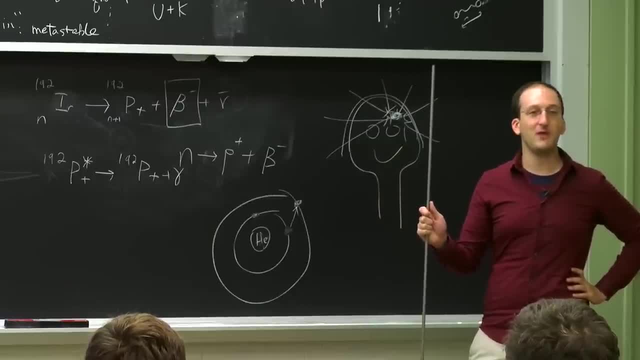 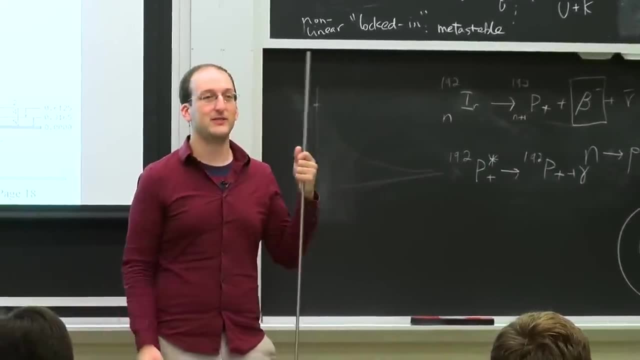 There are not enough pixels in this projector to show the full complexity of that, So you'll have to zoom in a little bit. but I'm not going to ask you to do anything with it, except for look at the three most likely transitions out of dozens, maybe scores. 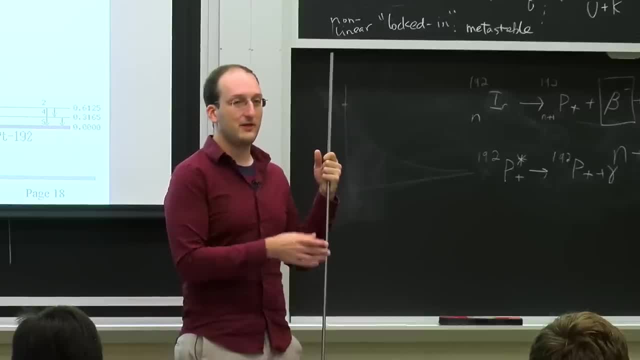 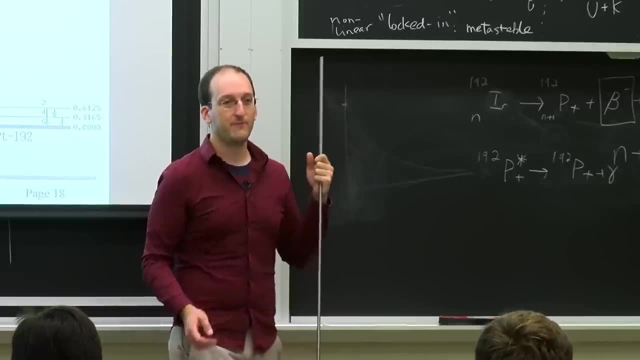 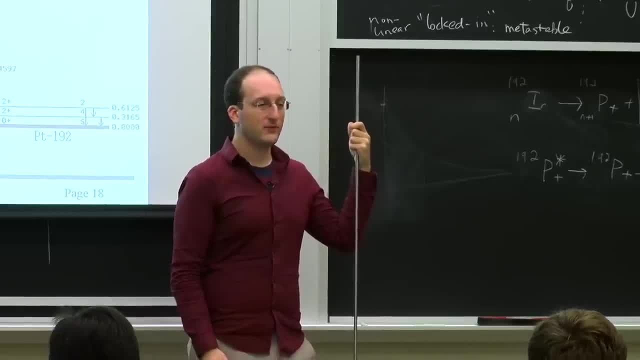 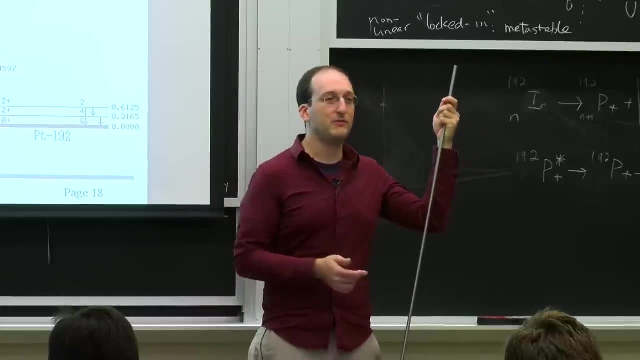 that there's still some left since the universe began. There's still a fair bit left, But you guys are going to actually calculate as part of your homework later in the course, how much uranium-235 was there when the Earth was born and how much has just disappeared, because 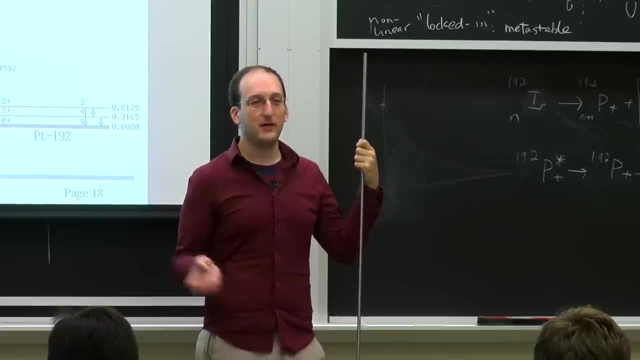 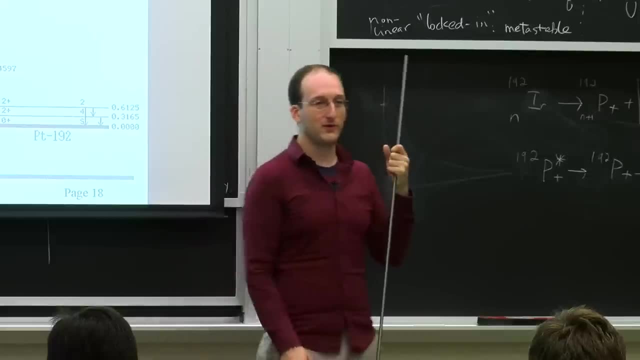 of the passage of time. So right now it's typically about 0.7% U-235 by isotopic composition. It was not the case when the Earth was born, But you guys will be able to figure that out. Yeah, so good question. 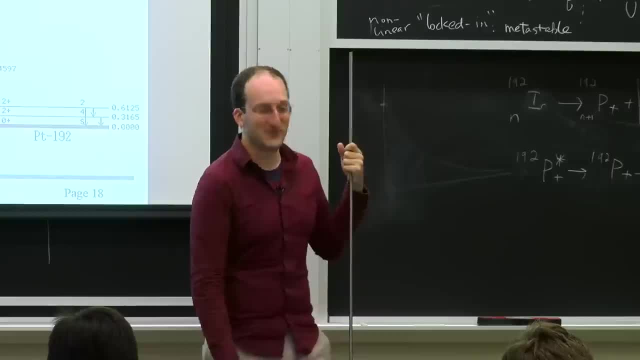 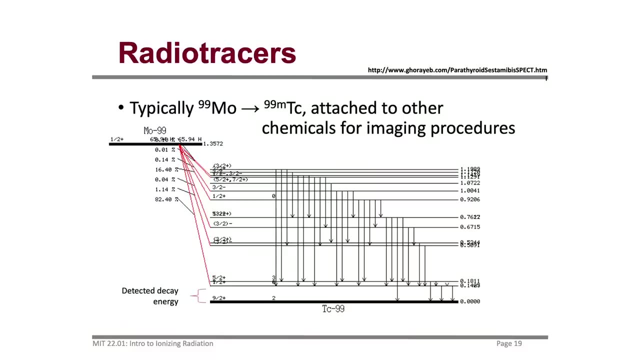 And have a rant from me, I guess, Just in response. I'll try and keep my answers a little shorter. Oh, here's a crazy one, Not particularly crazy, though. So this is molybdenum-99 decaying. 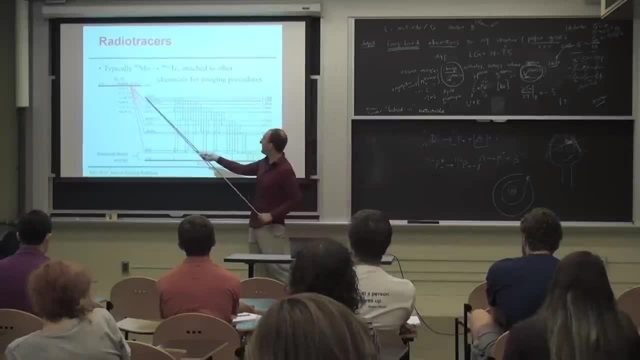 to technetium-99 metastable. There's lots of possible decays, but the most likely one is right here. the state above the ground state at about 140 keV, a fairly low energy and therefore more easy to detect photon. 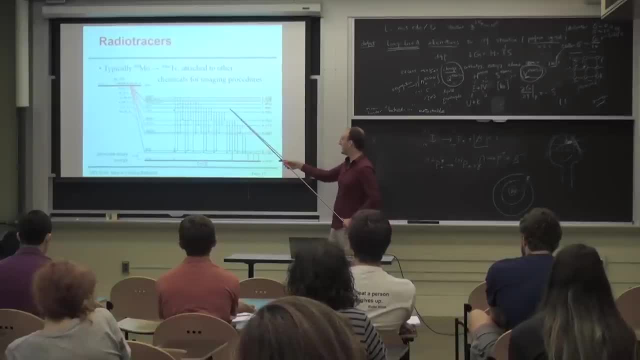 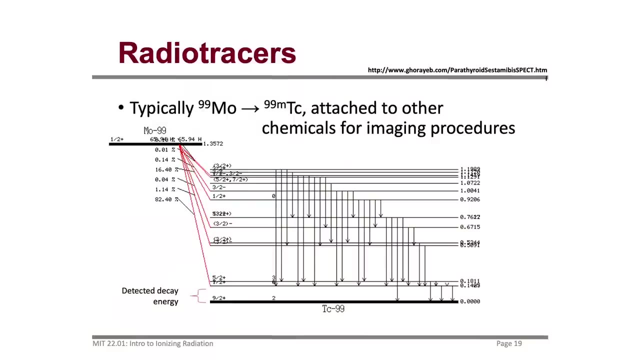 And so, if you notice all of this, almost all the other excited states, with a couple exceptions, decay down to this 0.14 MeV excited state, at which point you get decays to the ground state. Those also have a rather long half-life. It's a few days, So you can make molybdenum-99 in a reactor, transport it to a hospital, feed it to someone and use these 140 keV gamma rays- because they come from the nucleus- to image whatever the technetium will bond to. 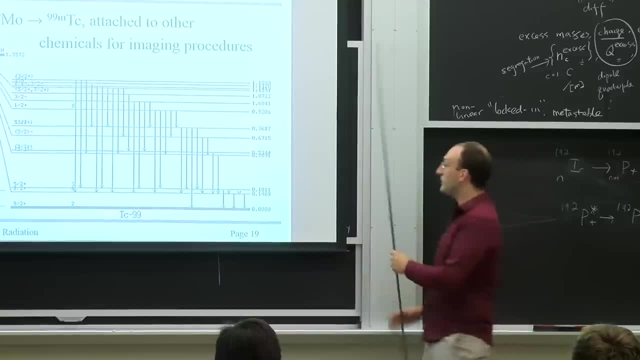 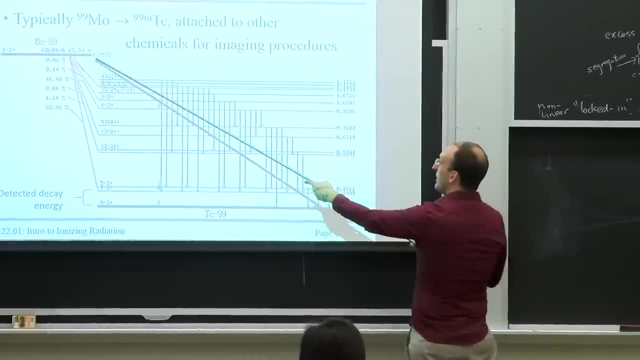 Yep Question. The M takes the 99. The M stands for metastable. Now, where do you see it, This one Yep? because the direct decay. you never go from molybdenum-99 to technetium-99. 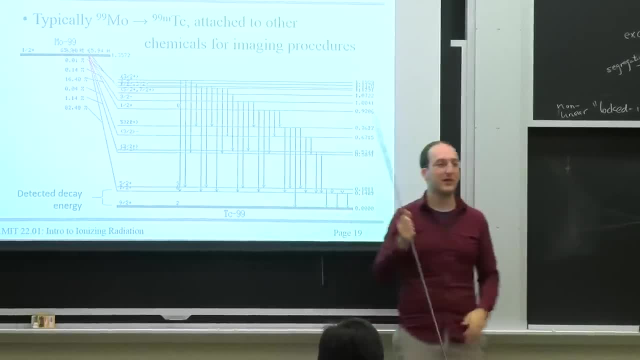 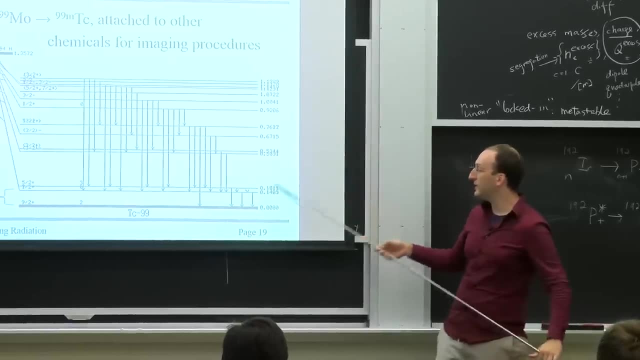 at the ground state. The M stands for metastable, so it's an excited state And metastable tells you that it's got a pretty long half-life. All of these other states are excited states. Metastable means it's kind of sort of stable. 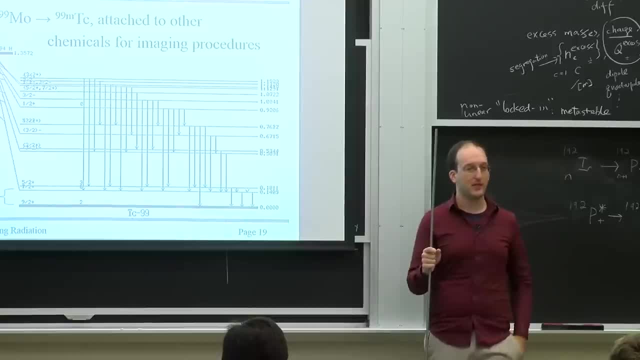 on like a human time scale of things. It's not technically stable, Because stable would mean infinite, half-life, close enough, But metastable means long enough to be detected or used, or significantly longer than the others. Any other questions before I move on? 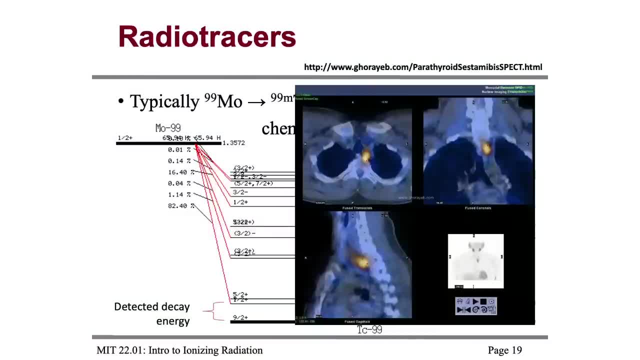 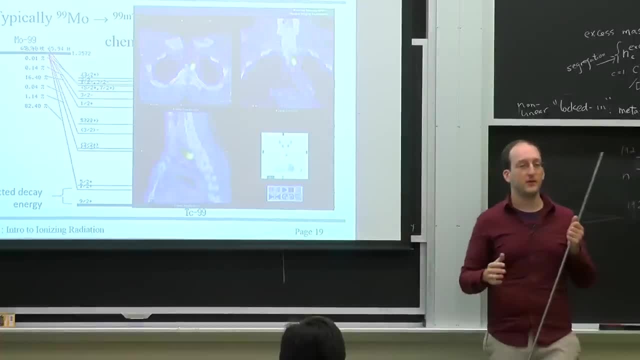 Cool, So you can use these to image where something is in the body. For example, you can use this to highlight certain organs, highlight anything that will absorb technetium, Or if you attach, let's say, the technetium to a type of sugar or something else that 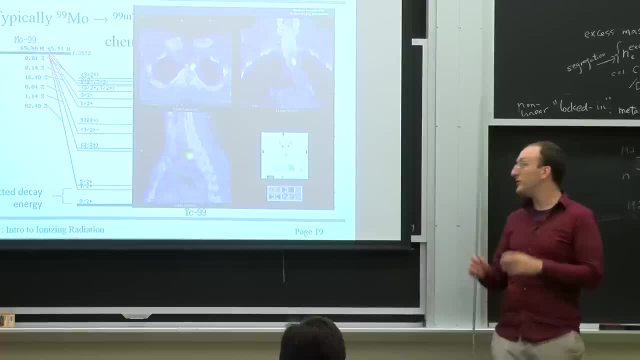 will be uptaken by the body, you can see where it goes And you can use gamma ray imagers to make kind of heat maps or radiation maps of where the technetium is going to find what could be causing the problem. The problem is well our main problem. 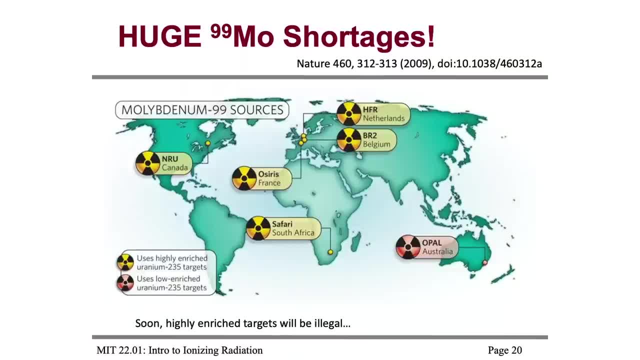 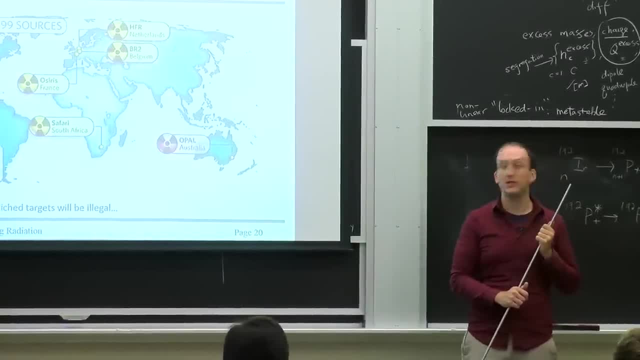 is there are huge moly-99 shortages Right now. the only economically viable way to make molybdenum-99 is in reactors, And there's only a few of these places in the world that actually make them, And I don't see any on the US. 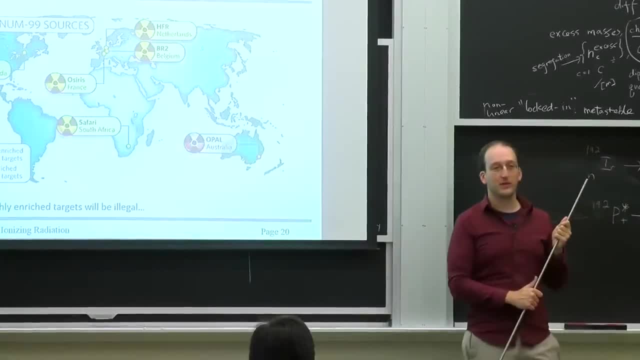 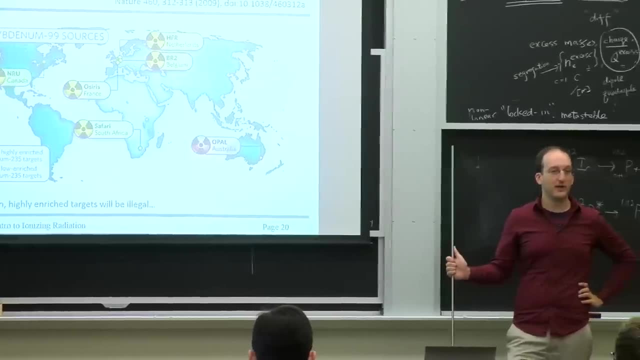 We get ours from Canada, And these are slowly getting closed down as we go. So the question is: with millions of these diagnostic procedures per year, where's the moly-99 going to come from? That might be where some of you guys come in. 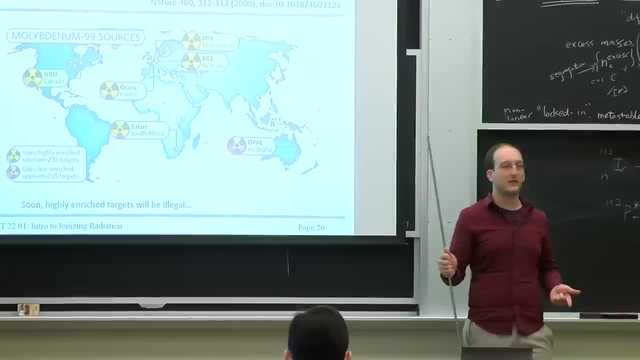 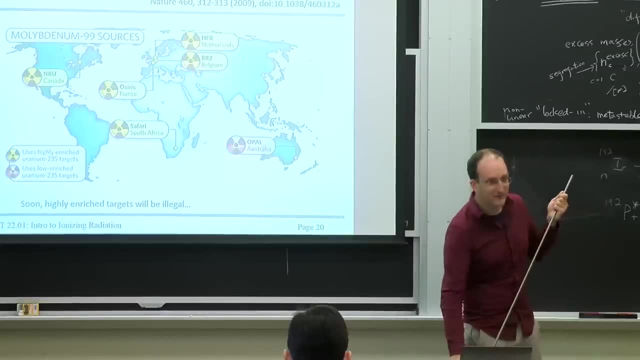 You can use the knowledge from this course to figure out an energetically and economically feasible way to make more moly-99.. You're rich. That's life goal achieved Space applications If we ever want to get off this Earth for a significant amount of time. 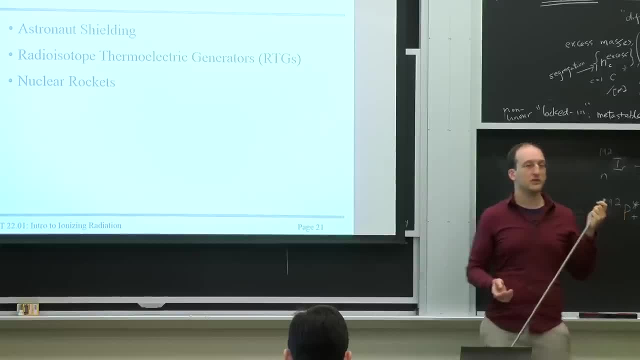 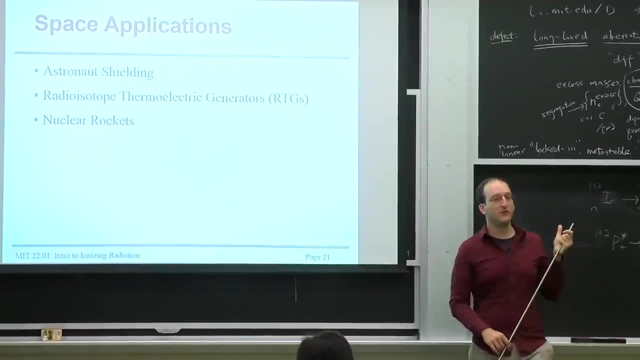 we have to deal with the fact that there's no atmosphere in space to shield us from the high-energy protons and other cosmic rays that would otherwise well destroy life. So there's a lot of interesting ideas and a lot of problems with astronaut shielding. 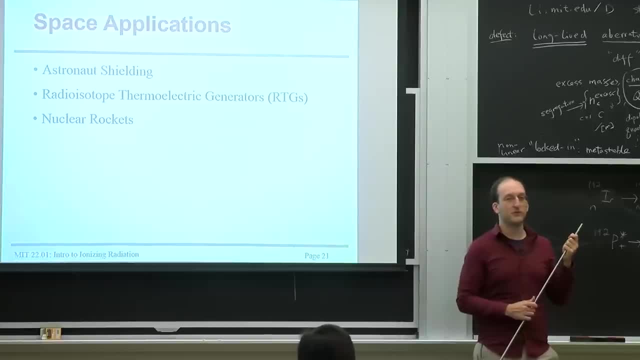 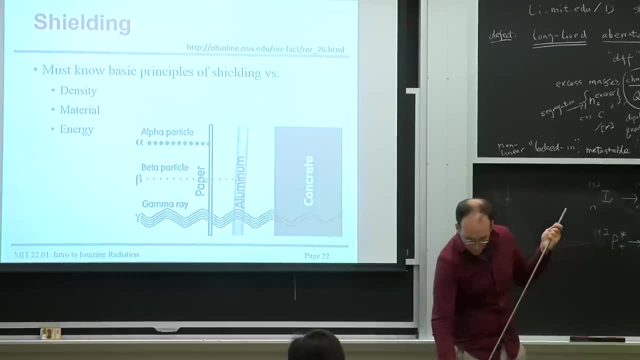 One of them is that the protons are so heavy. I'm sorry. the protons are so energetic that they're difficult to shield just by mass attenuation. And the trick here is well, different radiation has different penetrating power. It depends on its energy, but it also 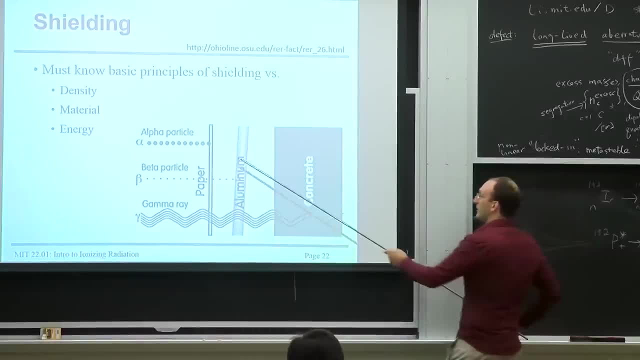 depends a lot on its charge. For example, alpha particles can be stopped by a sheet of paper. These would be MEV-level helium nuclei. Like if you hold an alpha particle source in your hand, the dead skin on your hand stops the alphas from getting in. 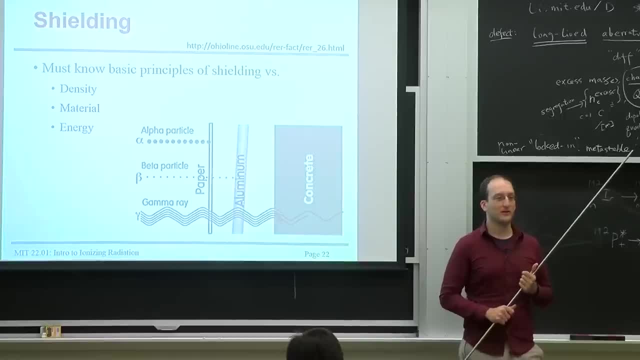 Remember that, because I'm going to be asking you a question later on to see who your friends are and who they aren't. I don't know if anyone knows what I'm talking about, But if you do, don't give it away. 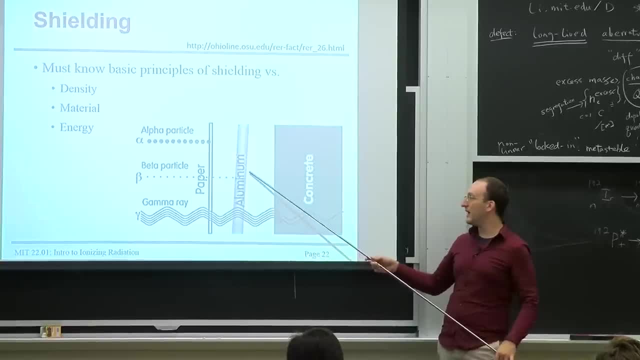 Beta particles, or electrons, have low mass and half the charge of an alpha particle. They can be able to get through paper, even through a little bit of plastic, but a small bit of metal can stop them. Gamma rays go right through. 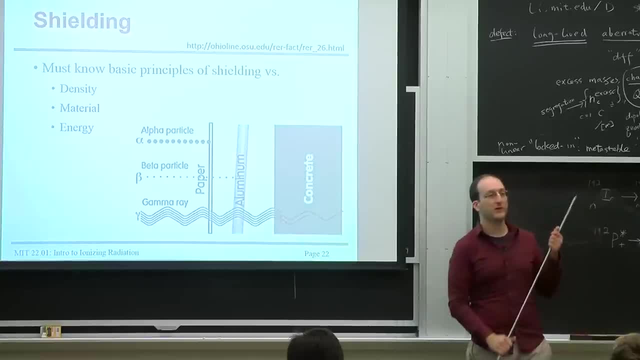 And notice that they've been drawn, not quite being stopped by the concrete, which is a great shielding material Because, like I said before, you can exponentially attenuate gamma rays, You can't with all certainty stop every single one. So then, how do you stop these high energy charged particles? 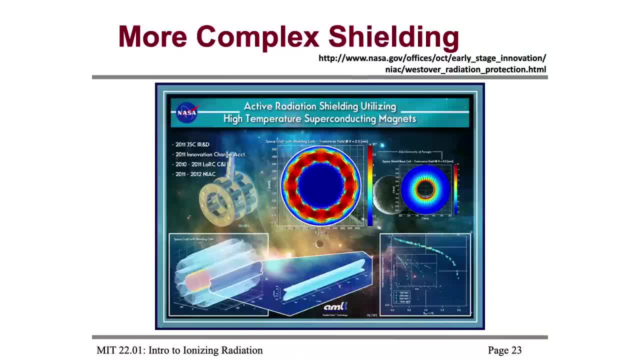 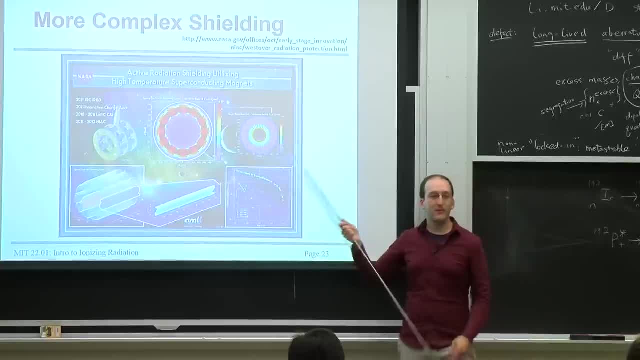 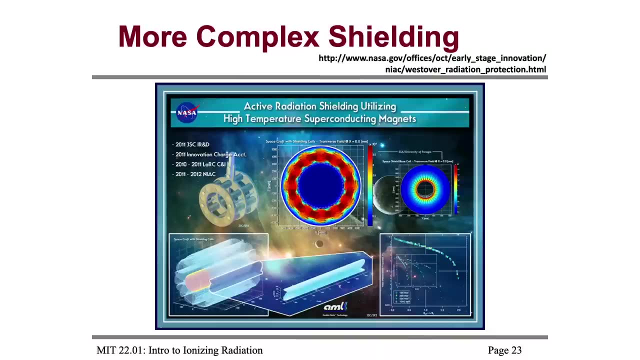 if the more energetic they are, the more range they are Boost your electromagnetic field. So it's actually been proposed to have spaceships with enormous magnetic fields or electromagnetic fields around them to deflect the protons away or around the ship. Because if you can't stop it by putting matter in the way, 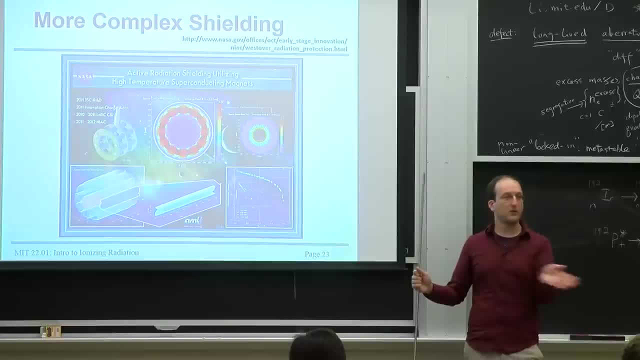 rely on the fact that they're charged particles and will curve around whatever's got a high electric field around it. So this is one way of, let's say, shielding deep space missions. You can't put more stuff in there, because stuff is heavy. 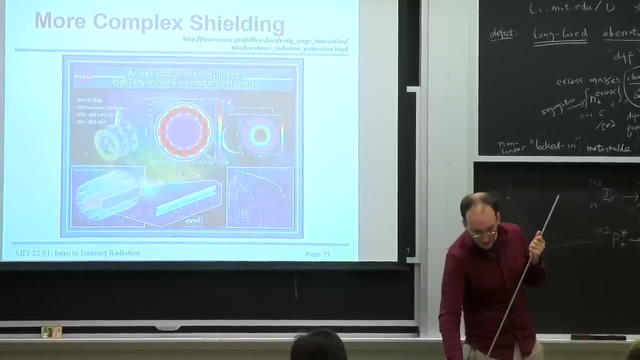 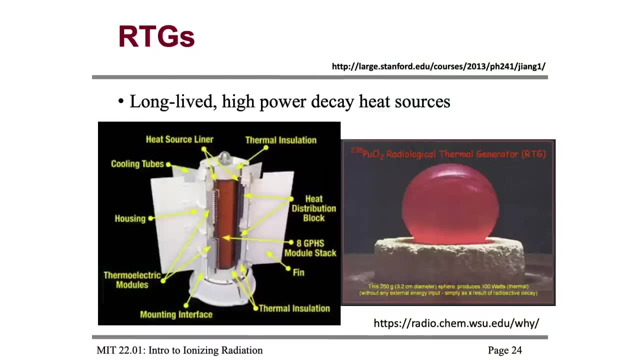 and launching stuff into space is expensive, Rely on electromagnetism And there are also RTGs or radiothermal generators or radioisotope thermoelectric generators, which are little balls of things like plutonium or strontium that give off so many alpha particles. 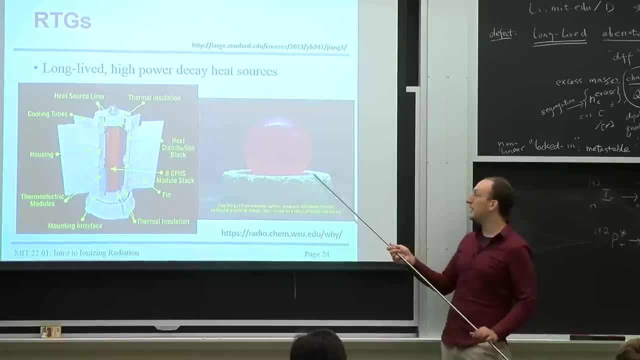 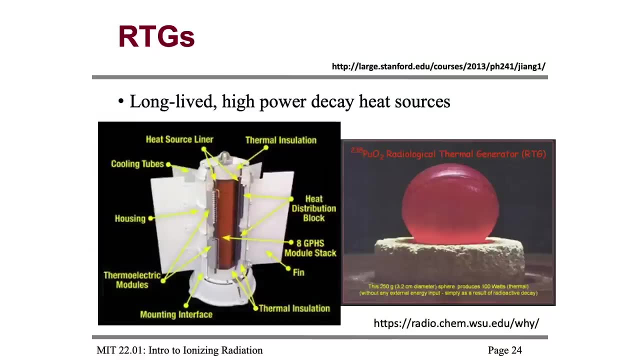 And the alpha particles have very low range. They deposit their kinetic energy as heat in the material and cause them to glow on their own. If you produce enough heat, if something's glowing red, you can use thermoelectric generators to capture that heat and turn it directly into electricity. This is how things like Voyager and, let's see, all the other space probes with interesting names are powered. Once you're too far from the sun for solar power to work, you need something that doesn't turn off, So you can use RTGs which have long enough half-lives. 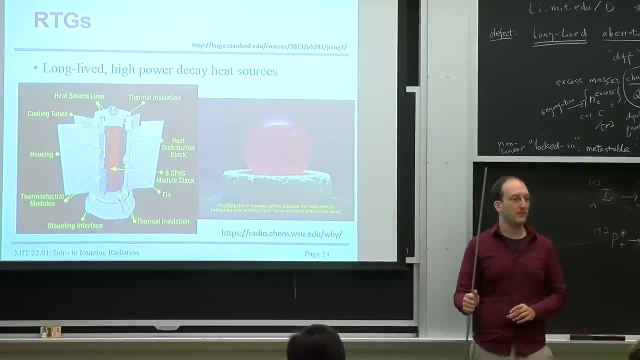 to produce significant amounts of power for a long time, but short enough- half-lives- so that their activity is pretty high and they release a lot of energy as radiation, And that radiation is heavy charged particles which you can capture as heat. So yeah, an actual little sphere of plutonium. 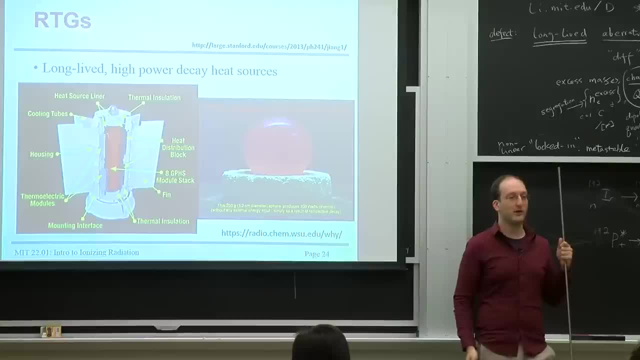 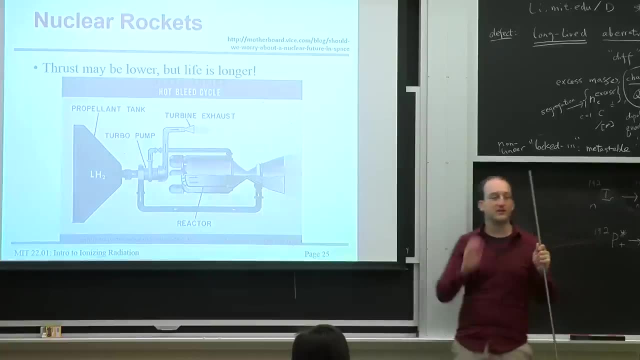 that produces 100 watts, just sitting there. There is no way to turn it off. That's the end of the sentence. It's plutonium And finally there's nuclear rockets, If you think about using a reactor for thrust instead of electrical energy. the design of the reactor, 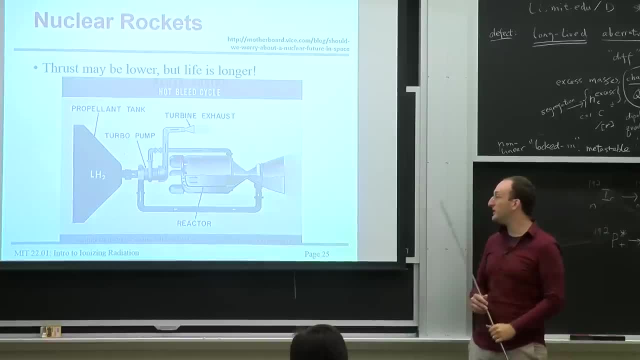 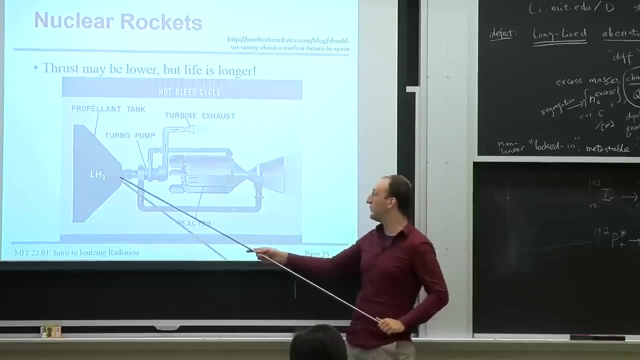 gets very different. For example, you can start to let things get a whole lot hotter when there's no oxygen in space to oxidize things And your propellant maybe would be liquid hydrogen that doesn't burn but goes to the reactor, gets accelerated. 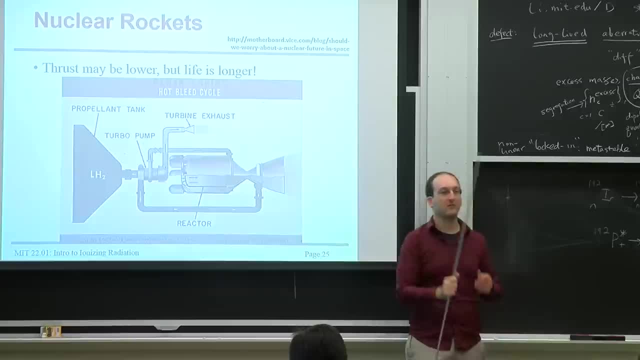 turned into a gas with a high kinetic energy to fire out the back of the rocket nozzle and provide the thrust that you need. And so it's nuclear rockets. that would really be the only feasible way without bending spacetime, which I don't think we've really done yet. 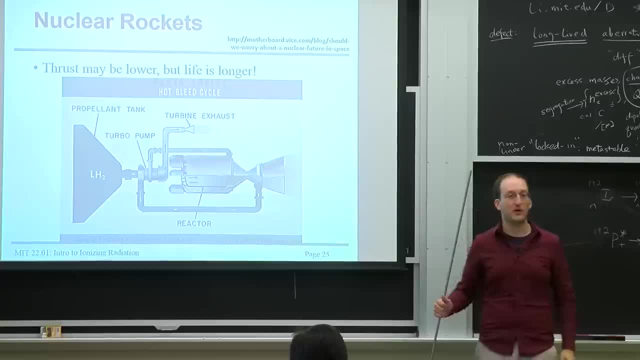 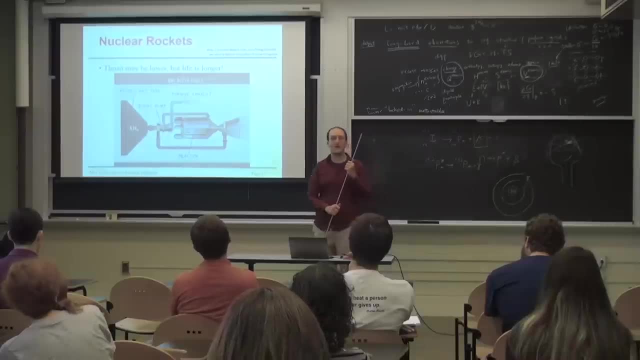 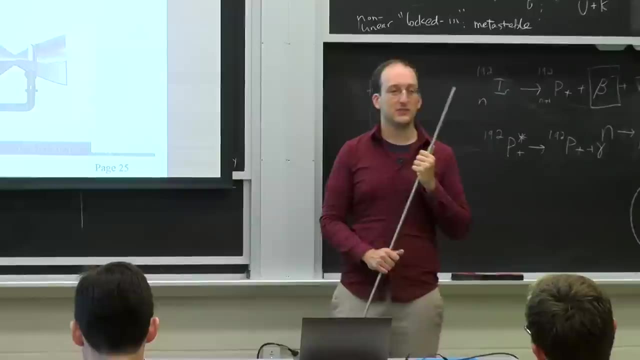 in order to get to very distant stars, like that planet they just found orbiting Proxima Centauri, Four light years away. pretty close, right? No, not really. If you think about how a nuclear rocket mission would work, well, it doesn't have to have nearly as much thrust. especially if you start from orbit. Maybe use a chemical rocket to launch yourself into orbit, then spend half your journey accelerating very, very slowly and then turn the rocket around, spend the other half of this journey decelerating very, very slowly. 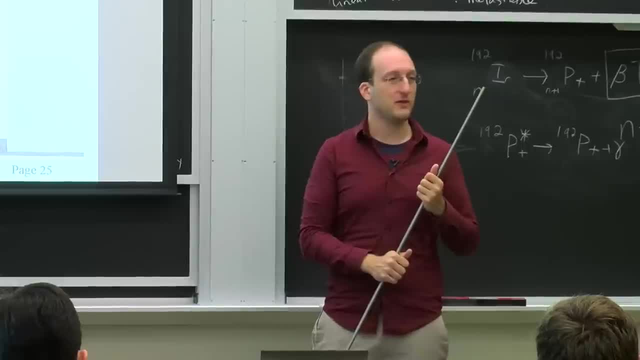 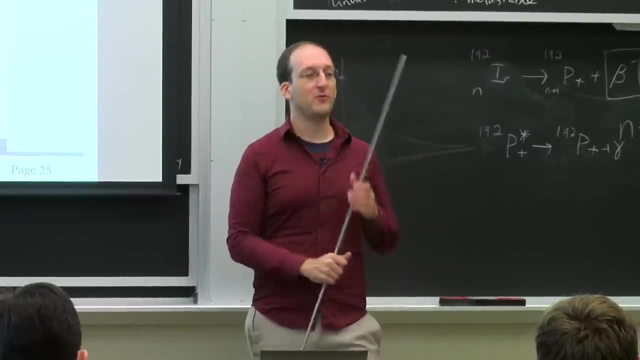 So you need a long, constant but low-level thrust for these long-lived nuclear missions. I'm going to stop here because it's five minutes before the hour. We only have a few more of these things to go through, But what I will ask is: you guys hang tight. 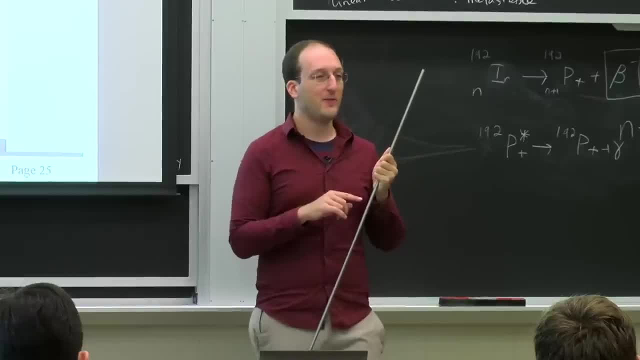 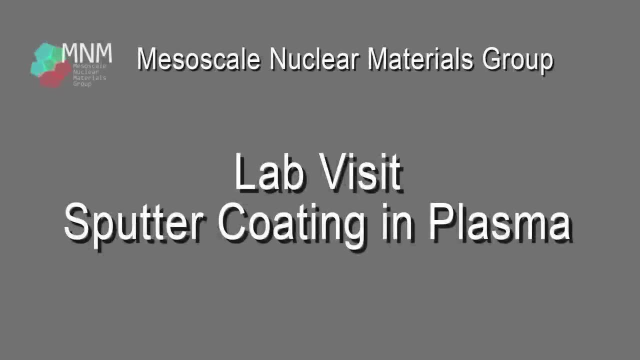 for the next few minutes, while these guys take the cameras apart, We're going to go to my lab and see an application of nuclear which, like I said, is plasma sputter coating. All right, everyone. So welcome to my laboratory. 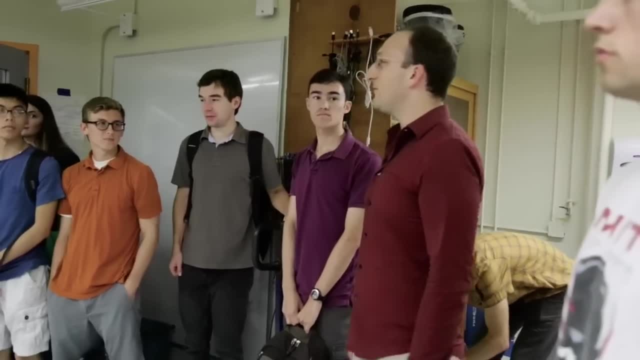 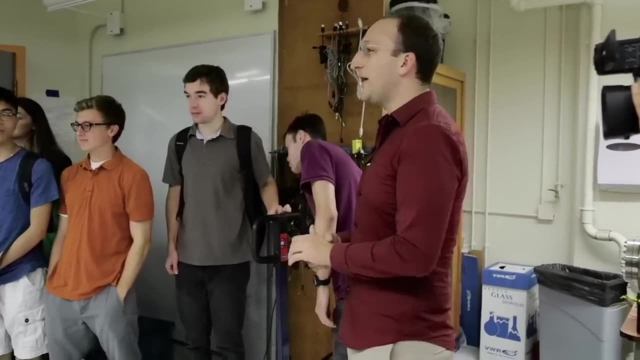 This is the Mesoscale Nuclear Materials Group, where we make and break materials for nuclear technology, Usually not in that order, but whatever, We get it done somehow. And this is Reid Tanaka, one of my graduate students who's actually repaired. 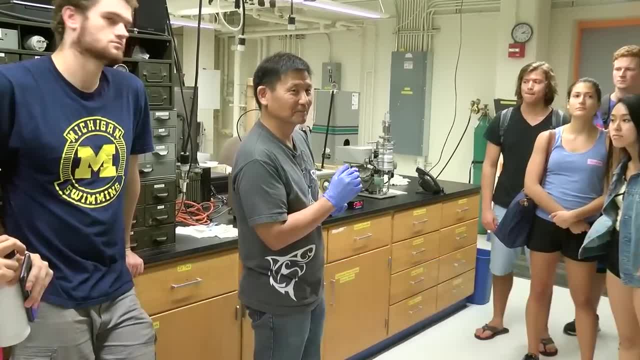 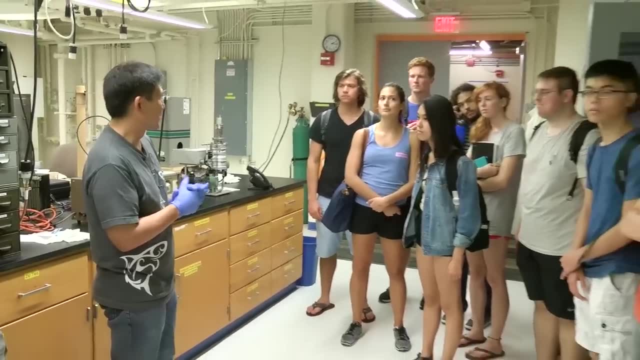 I'm going to show you the physical principles and operation of a sputter coater, which is nothing more than a controlled radiation damage machine, And he'll be making some interesting door prizes for you guys. Well, as Professor Mike Schwartz said, 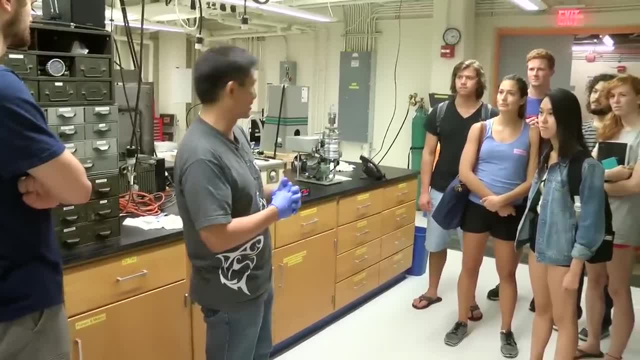 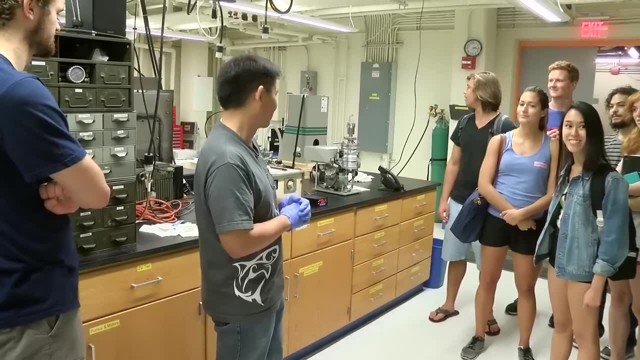 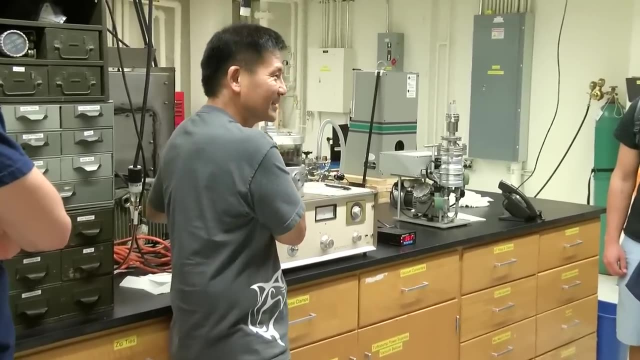 this is Professor Mike Schwartz, who calls it something else. I call it the home, the rehabilitation home for old orphaned equipment and old graduate students, And so this is actually this piece of gear here. I did a little research on it And I think it was built about the same time. 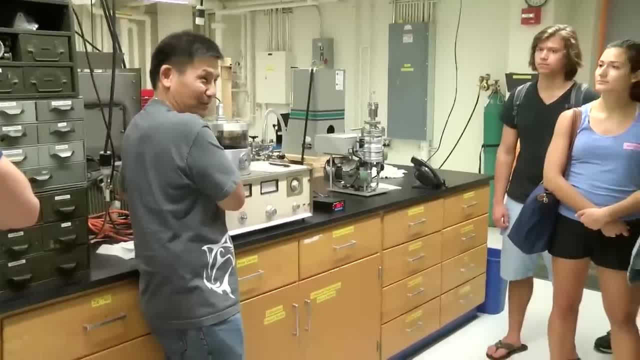 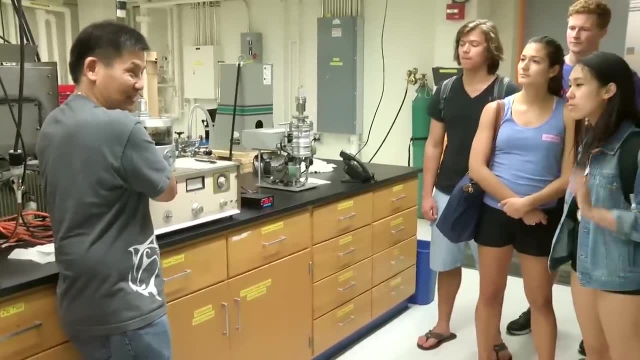 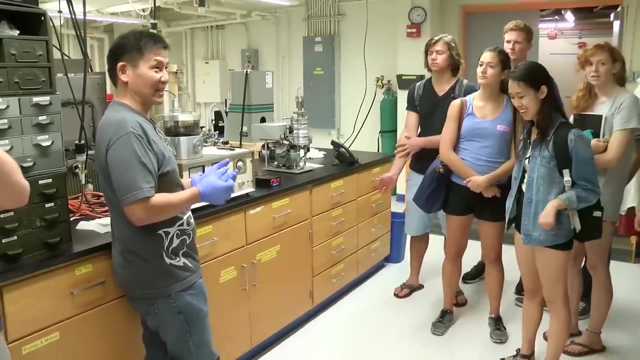 as I was entering college 35 years ago, So about 1978, maybe 1980.. That's how old this thing is. And then so Professor Schwartz goes around and asks all of us that we scrounge and we scavenge and we put stuff together. 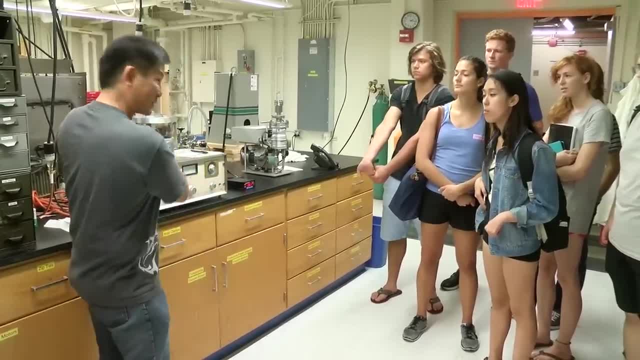 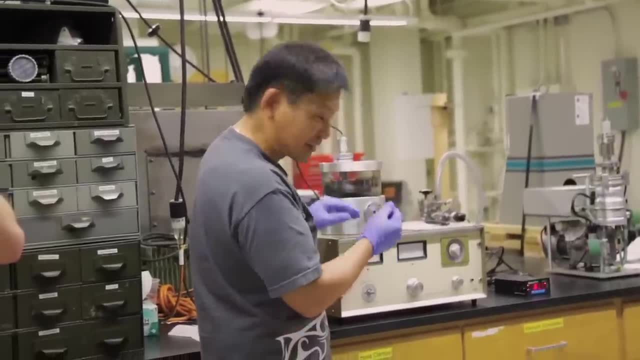 And you'll see that really, indeed, we use that a lot. So this part we put together out of a bunch of pieces of parts, If you look at it, and I'll talk to it a little bit, but there's a procedure that we've gotten rich out of. 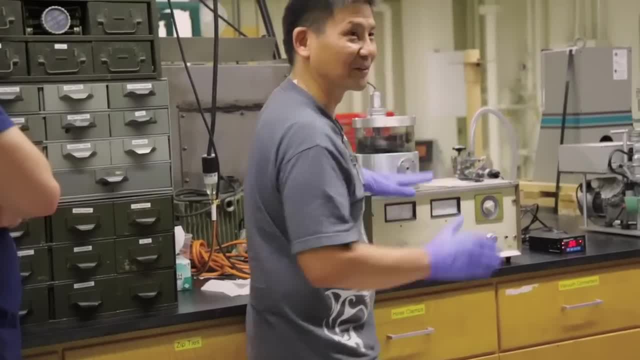 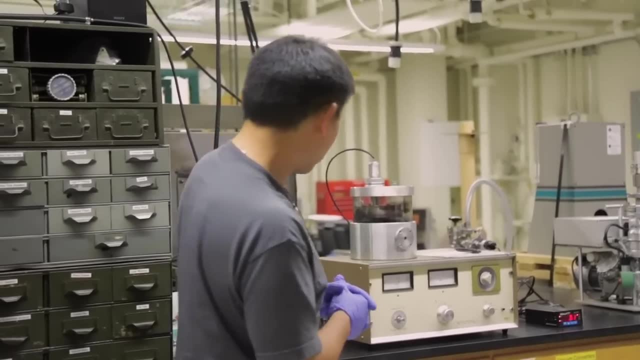 But we don't know what these knobs exactly do, So we just sort of throw them together. So what you're going to see is a little demonstration of what a sputter cutter is. You're going to see a little plow. It's under vacuum right now. vacuum pressure. 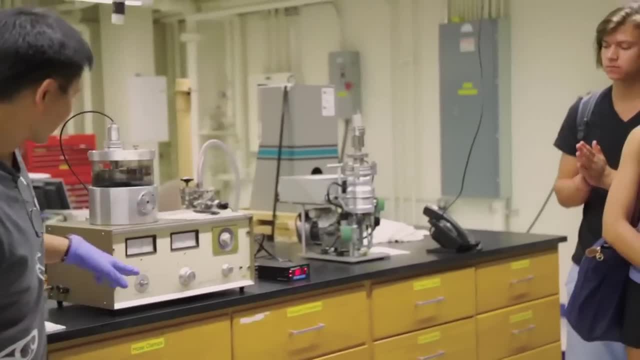 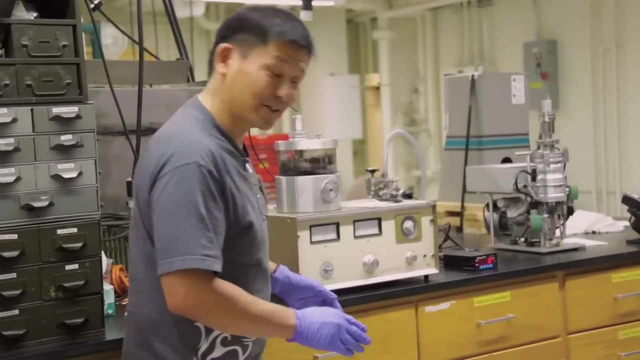 There's our vacuum pump. Let me just come right here so you can see Again. there's another pressure indication, But we don't actually trust that one too much. Without further ado, I'm going to just power it on. We're going to put this under a high voltage. 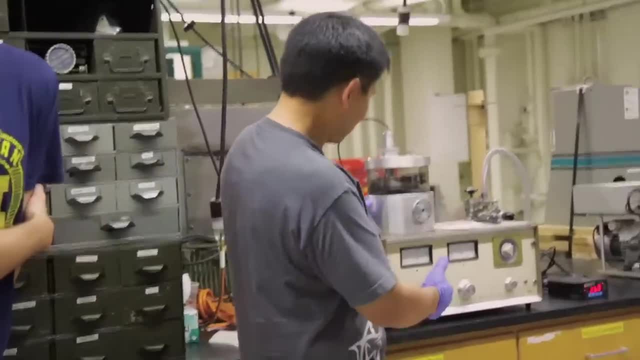 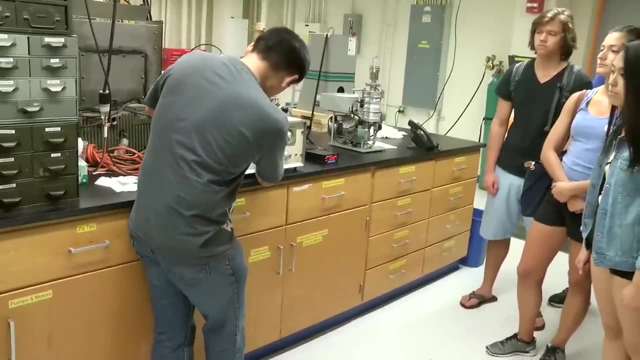 There's argon in here. We've got argon supplies in that bottle over there And we'll just take it. Got it? Just turn on the high voltage power supply. Turn it up. Should we get the lights? read Voltage. 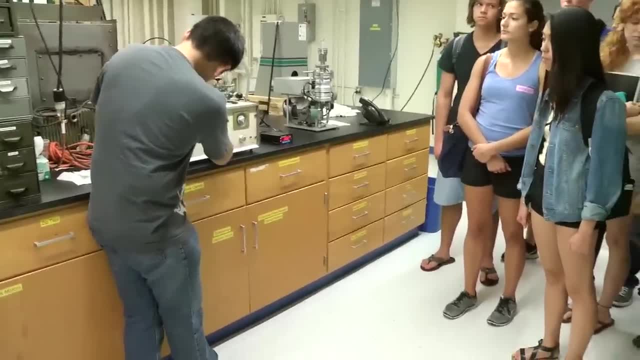 Yeah, We can go to the lights. I'll go get them. I'll just get them right over where you are And if you see through this glass jar, it's going to be a little bit of a glow, Some of them. you might be able to see it already. 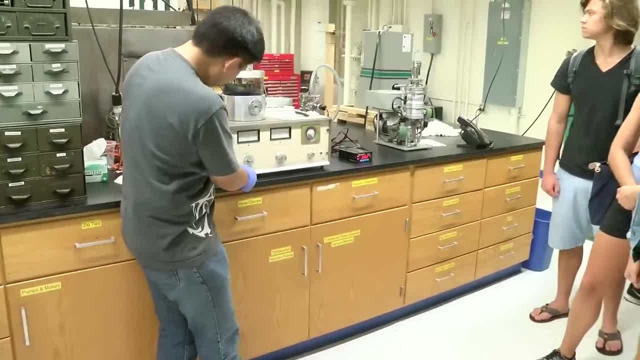 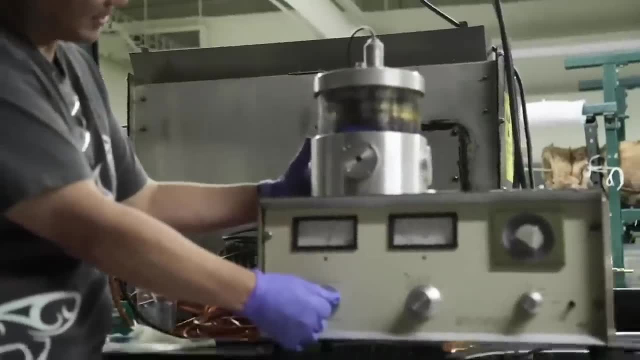 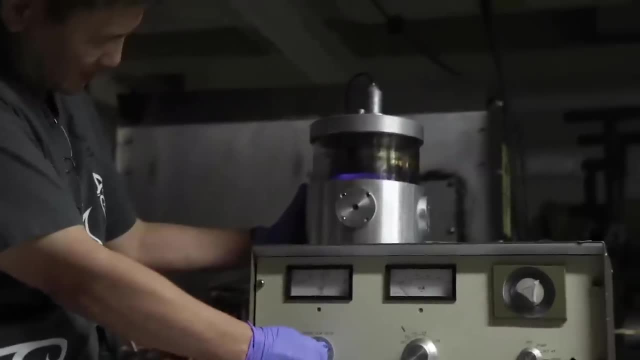 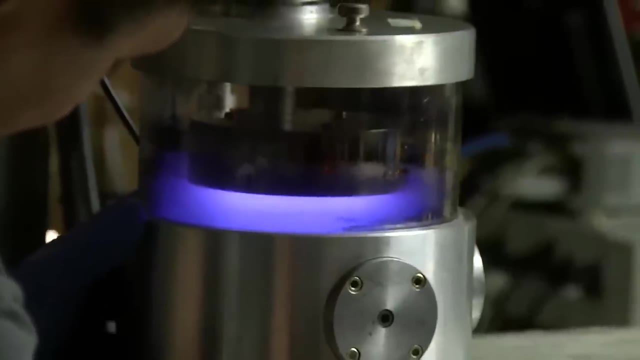 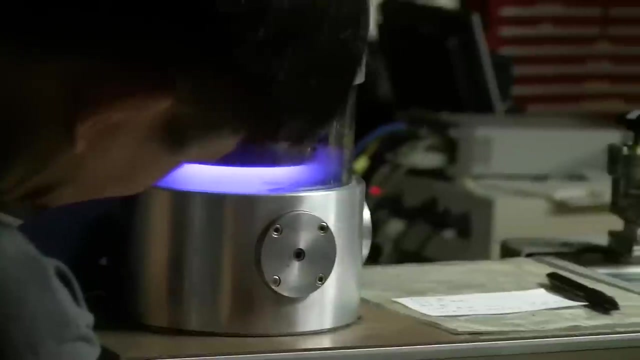 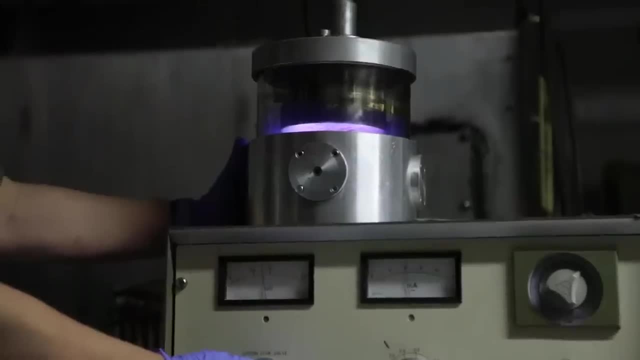 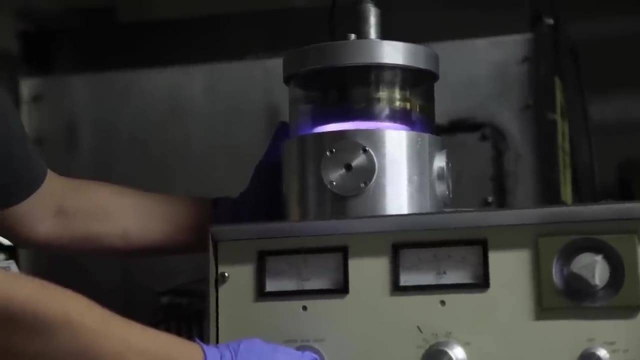 that you'll see in a second. But this is a controlled application of ionization and radiation damage using a couple of kilovolt argon ion. I don't know if you'd call it a beam, but at least an argon ion plasma. 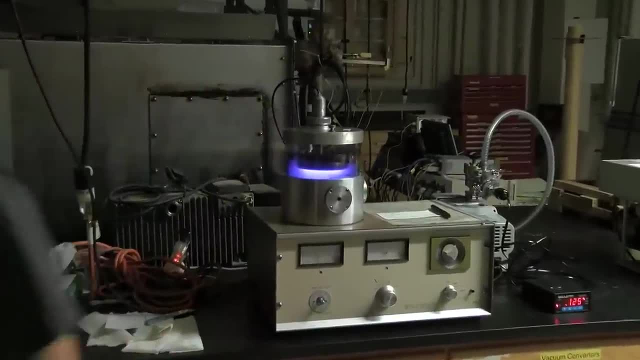 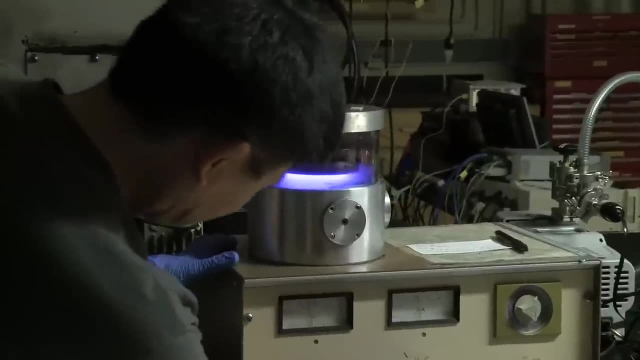 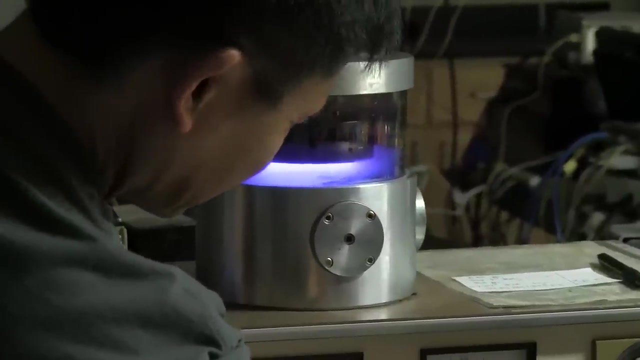 so there's a few other things to know. remember how we talked about charged particles having a certain range in matter. well, charged particles, and let's say low energy particles in the kv range, do not have a very high range, even in gases, which is why reed has this vacuum pump connected. 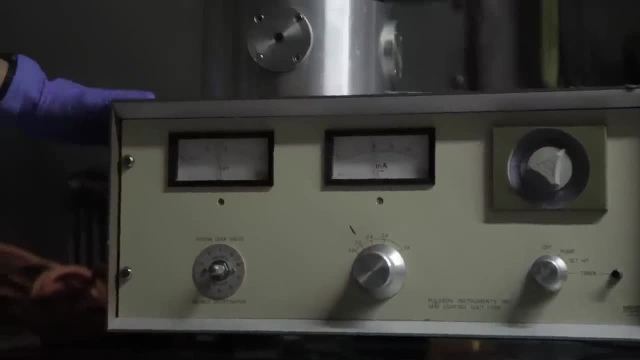 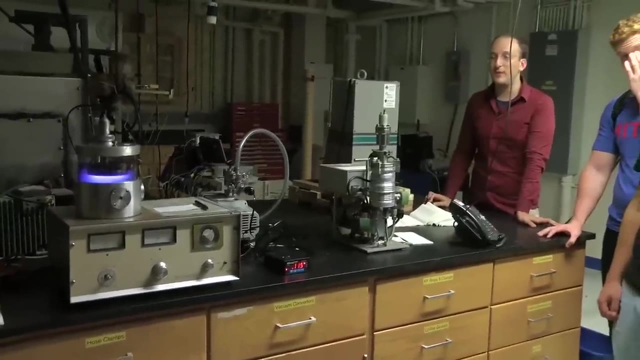 otherwise the argon wouldn't make it to where it has to do the damage. so when there's too much gas in there, shuts off. when there's not enough argon in there, there's no argon to do the damage. so we're actually exciting about two kv ions and their range is higher than the distance they have. 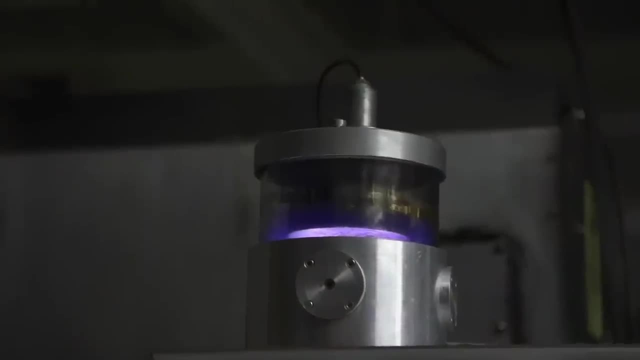 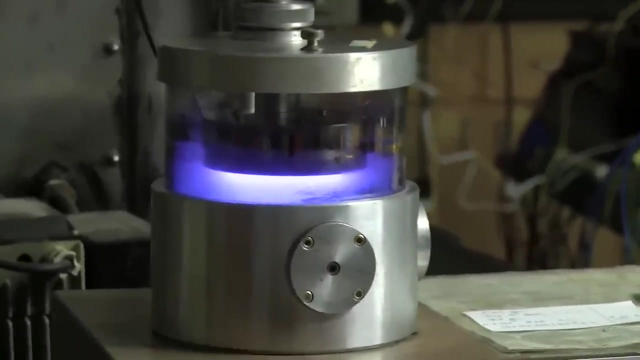 to travel, so they actually make it where they're supposed to go, and this is a kind of direct application of nse, along with a fair bit of high voltage electronics, and that's pretty much all there is to it. you have about two minutes if you want to take a closer look at this. yeah, 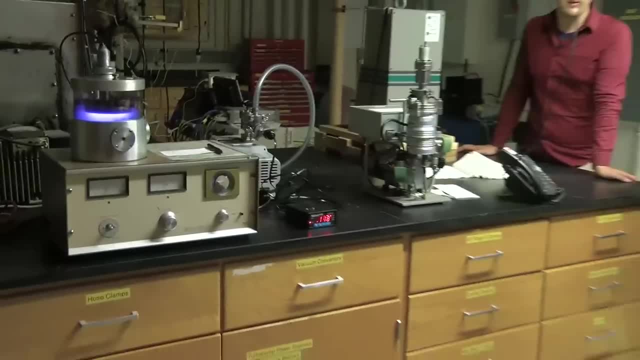 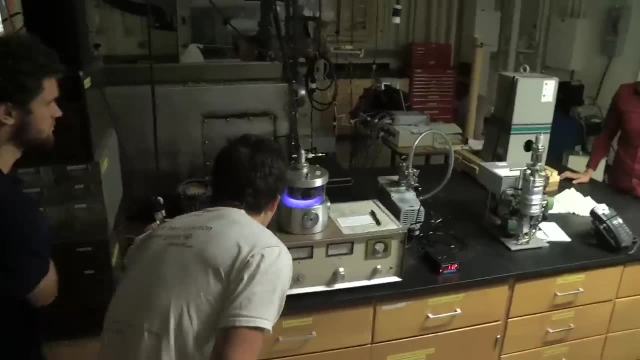 it's not going to hurt you. they'll get right in there. you, if you want to say, if you look underneath, you'll actually see that a blue glowing ring that's actually a ring of gold that's being hit by the plasma and that's causing gold ions to fire onto. 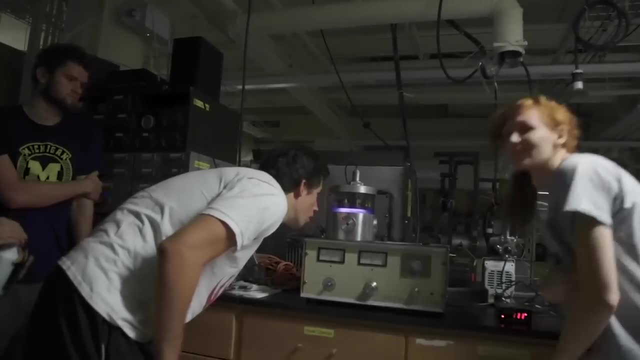 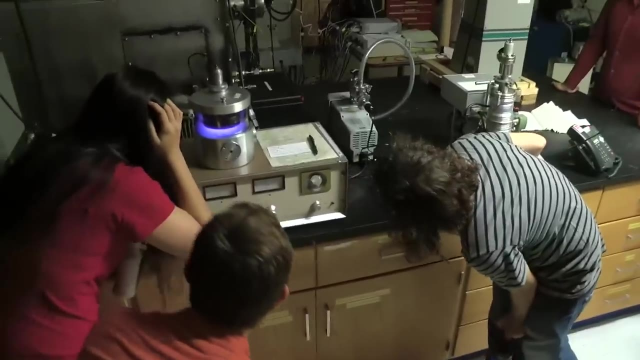 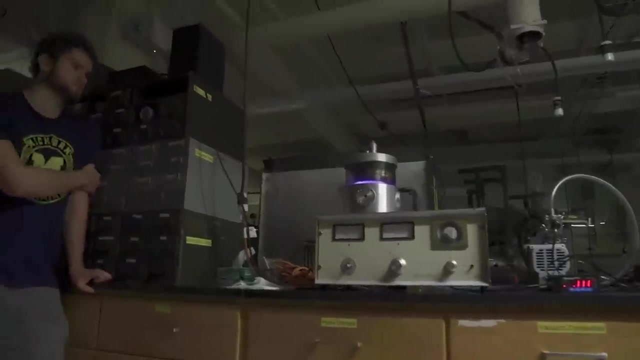 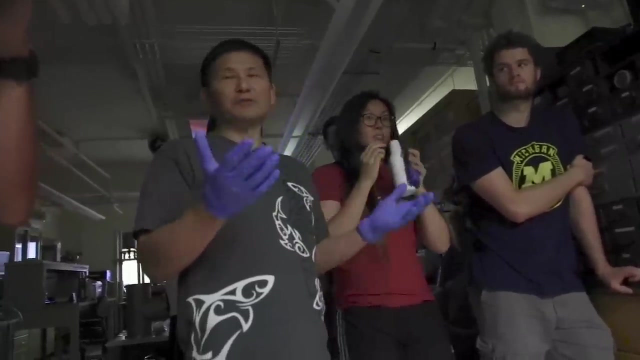 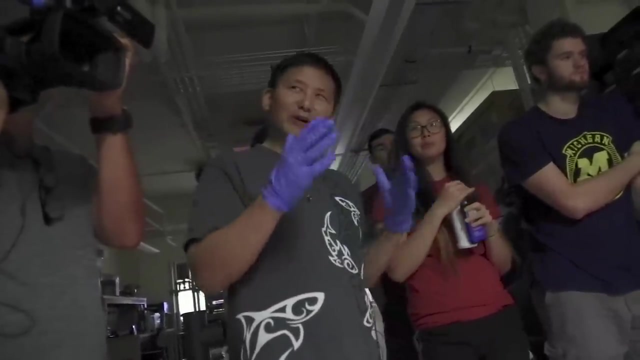 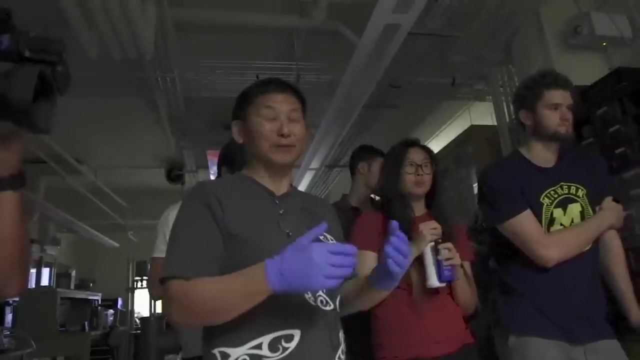 the target. you guys all know about chemistry at some point. right, they tell you that you know, one of the great mysteries in the world that we've always tried to solve is when you take something and turn it into gold. well, you should know that only the nukes can do that. right, really, all you got, you got to get away from all the electrons and all that other chemistry stuff, and only the nukes. so if you really want to turn something to gold, you got to join the nuker department. 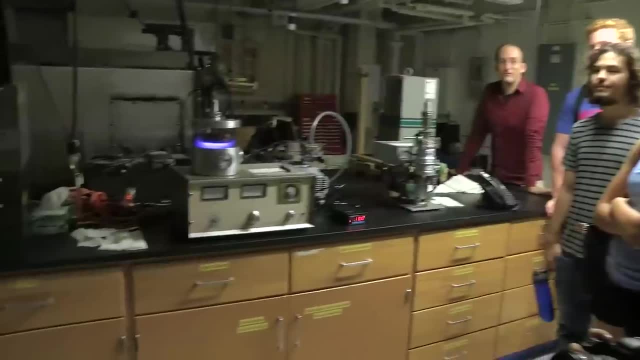 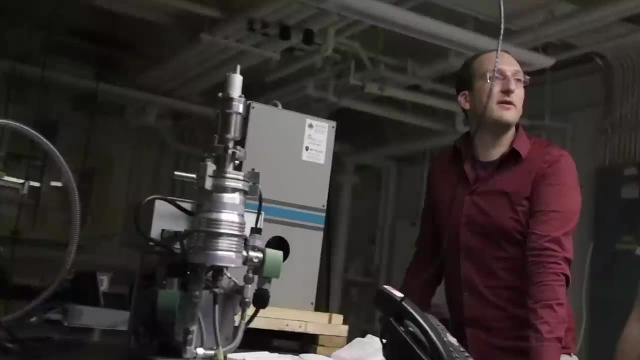 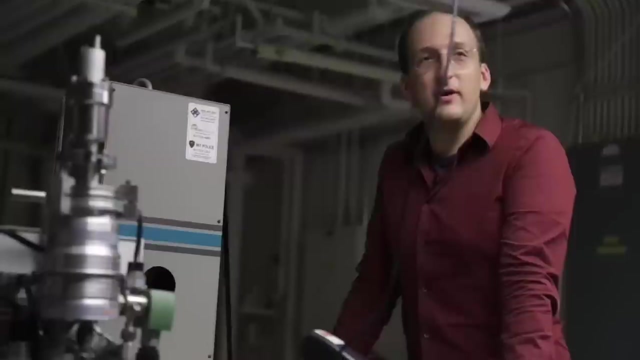 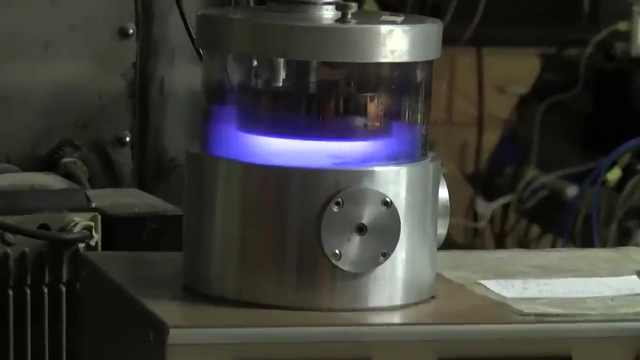 okay, let's just let you know that. keep that in mind. you everyone had a chance to get a close-up. look, okay, anyone have any questions about what you're seeing here getting like super hot there? it's good question. the temperature does not go up that much. 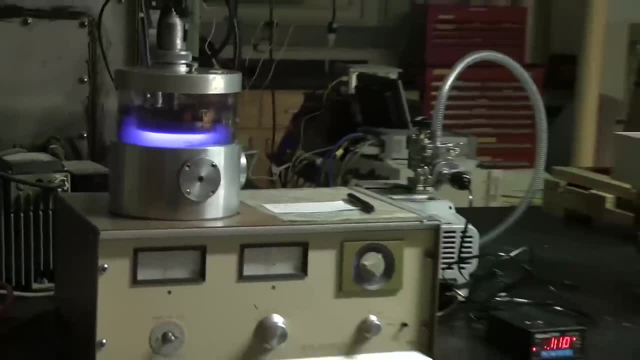 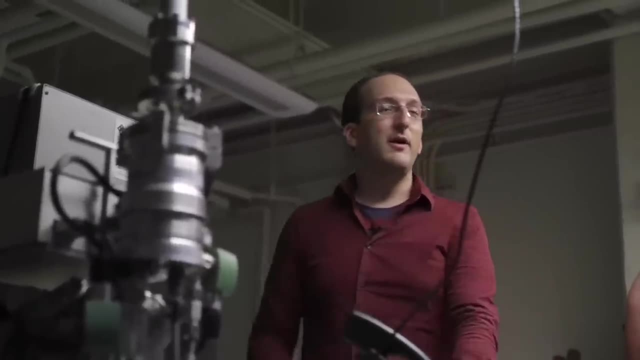 there's certainly kinetic energy turned into thermal energy, as the argon hits the gold and the gold hits whatever you're trying to coat, But the total amount of energy, the density of that gas, is extremely low. That's another reason why in fusion reactors, 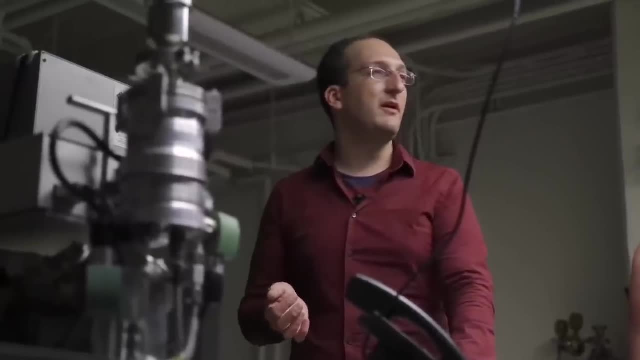 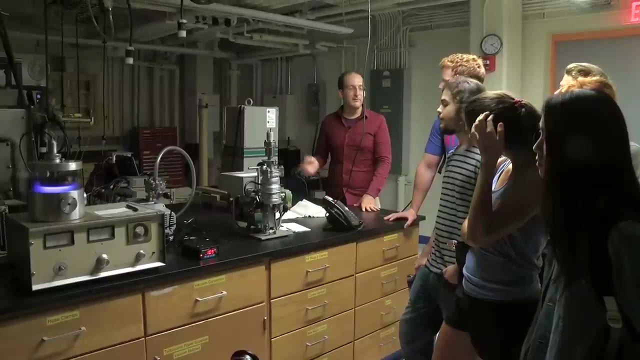 the plasma is up to millions or tens of millions of Kelvin. There's just not a lot of it. So if you look at the total amount of stored thermal energy in a fusion reactor, it's quite low, even though the temperature or the relation 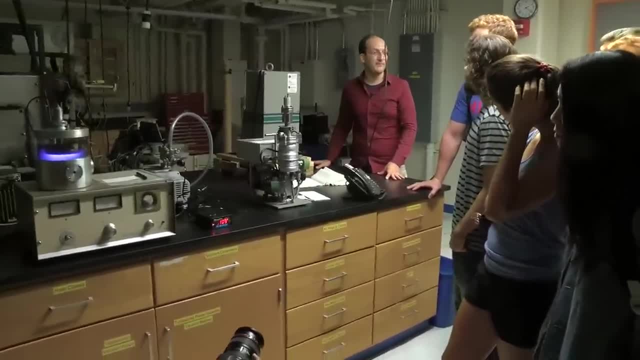 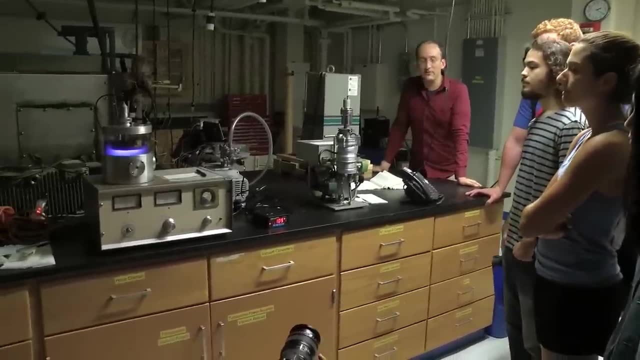 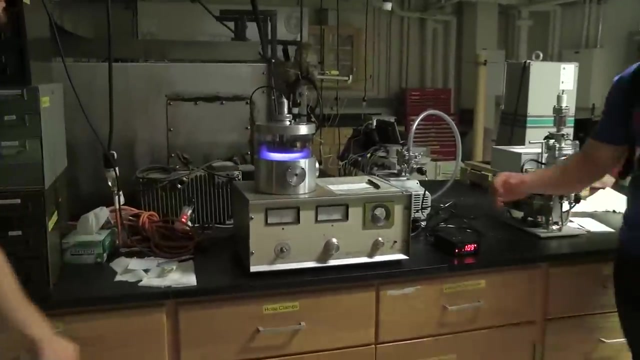 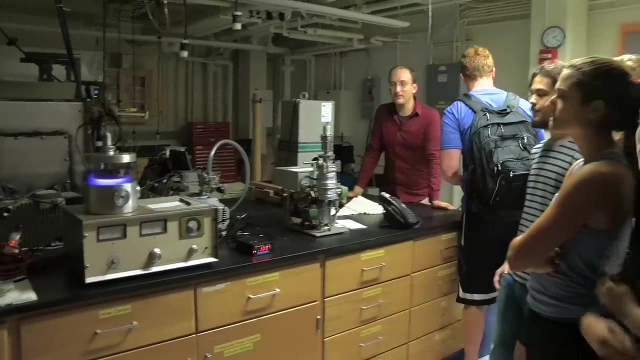 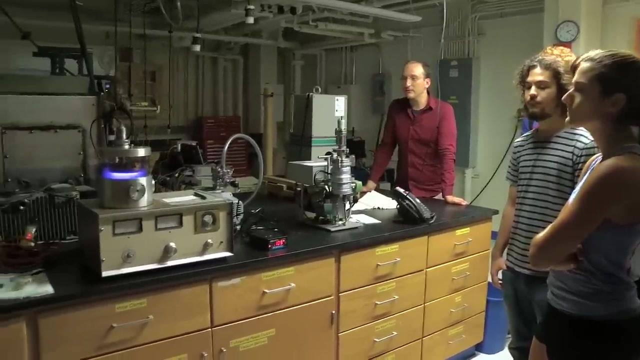 to the average kinetic energy of the molecules is extremely high. So, yeah, good question. If you want, put your hand up to the side of the chamber. Is it warm? Not at all. Yep, So the plasma is argon, and where? 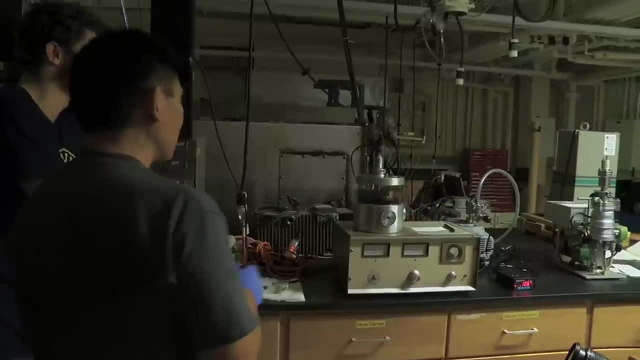 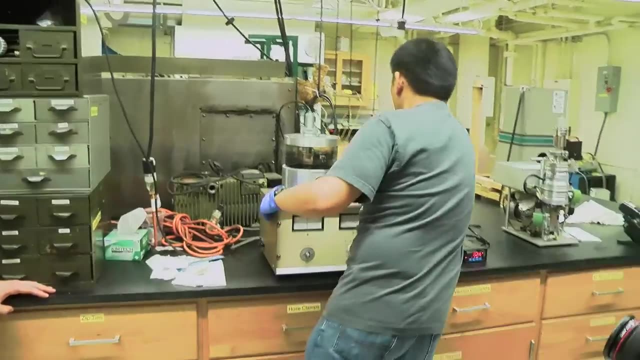 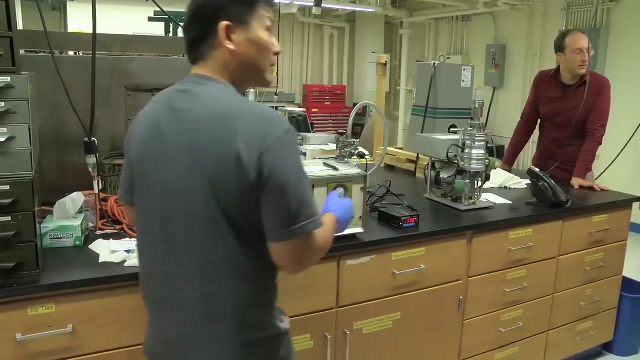 is the gold coming from From the reactor There we go. Yeah, we'll open it up and show you, So I'll get the lights on now. OK, Why is it that the pressure changed? Or was it the glowing? What's that? 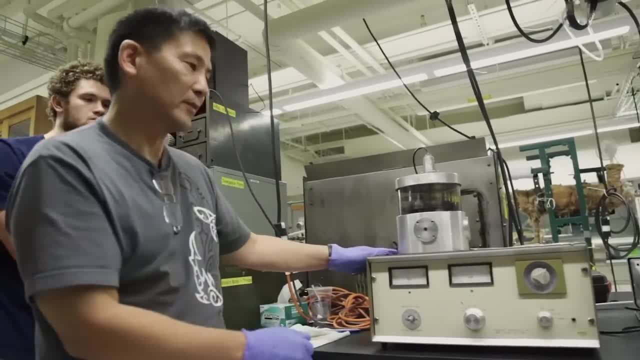 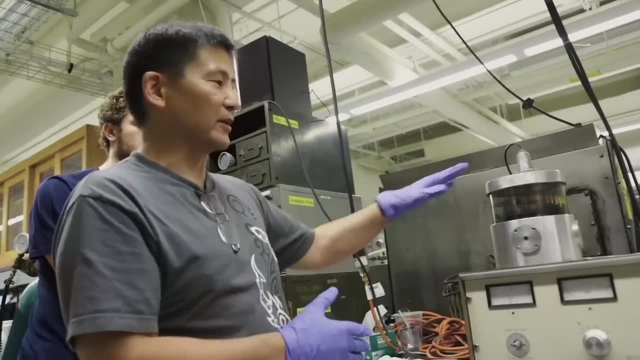 The pressure changed So it went from 0.09 to 0.06.. Yeah, From the point that when you walked in and saw that, Yeah, OK, The first thing, The first thing, OK. So this had a sort of a static amount of argon in it. 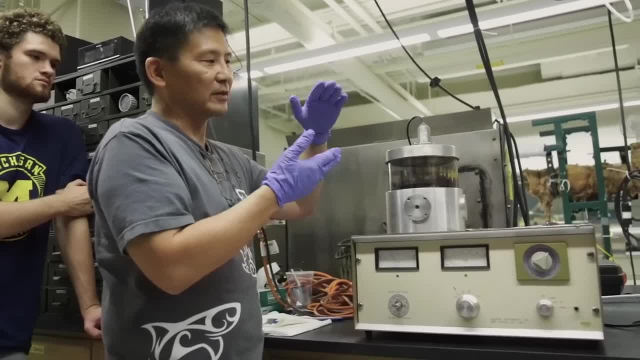 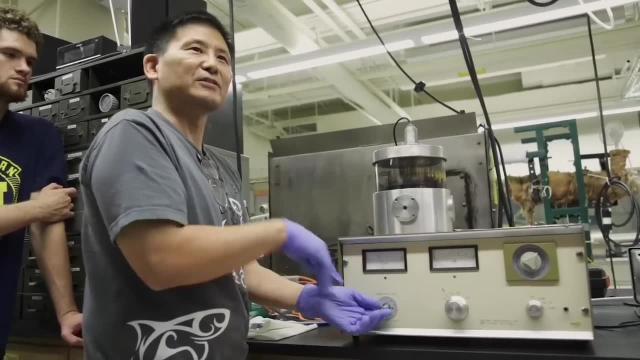 And when I turned on the voltage, the high voltage that's to create the plasma, But then it has to get fed, And so what I ended up doing with this little knob here I probably should explain, that is, I was feeding it argon. 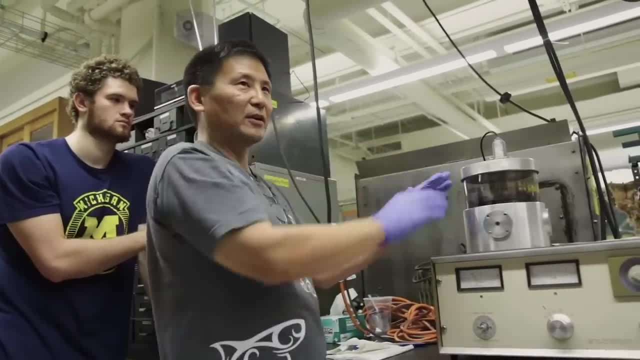 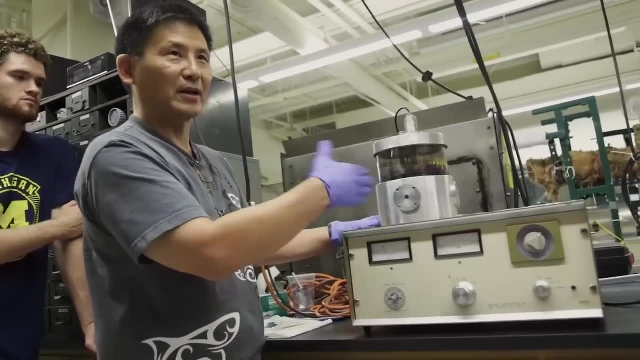 OK, So the argon bottle's moving here, It's going into this chamber. When you're feeding the argon in, then the pressure comes up, And if the pressure comes up too high on this particular instrument, then it has an automatic cutoff where the high voltage comes out. 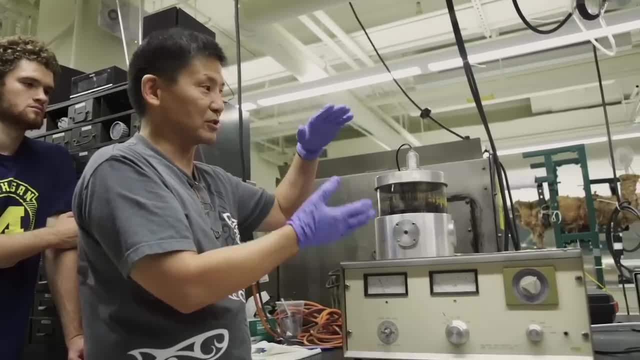 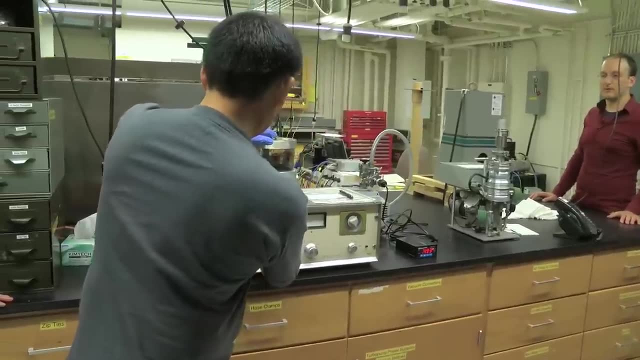 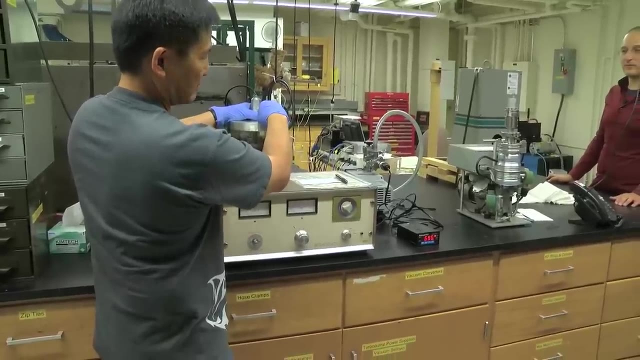 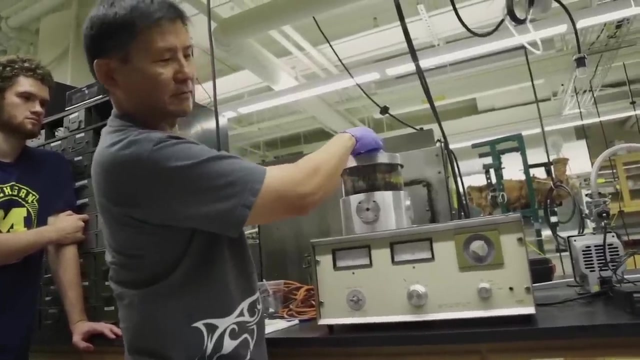 Because otherwise, you know, one of the reasons why it works is because we have so few atoms in there. Measure it like that. OK Yeah, Do you know what atmosphere pressure is in 4? 768?, 768.. 760.. 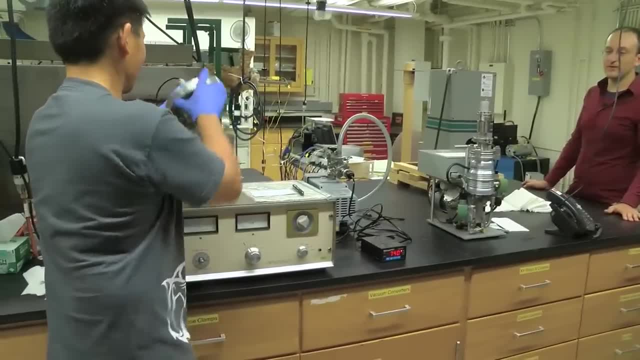 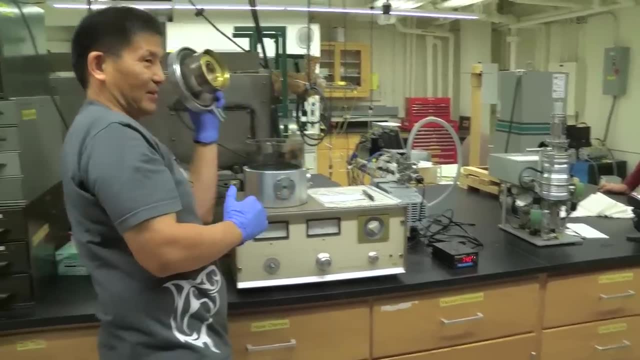 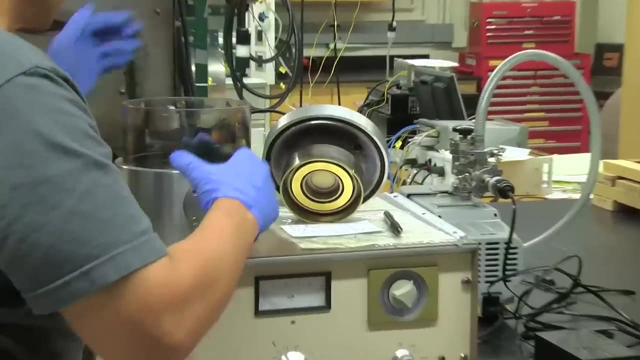 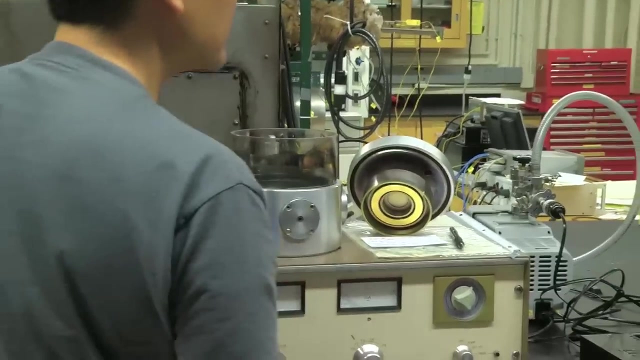 That's your line 760.. Maybe we actually have a little bit of a. So this is that. That's the gold ring, And in the chamber you can put the ring facing down for stability, if you want. I said you can just put the ring lying flat down. 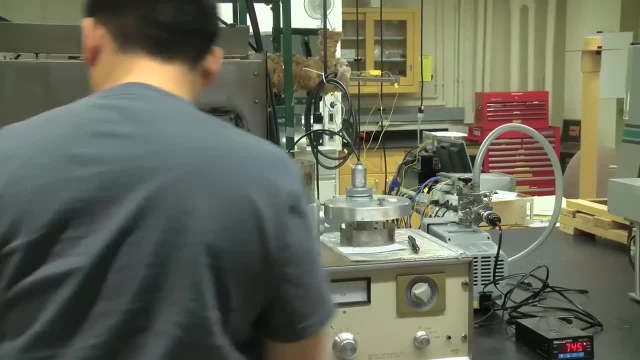 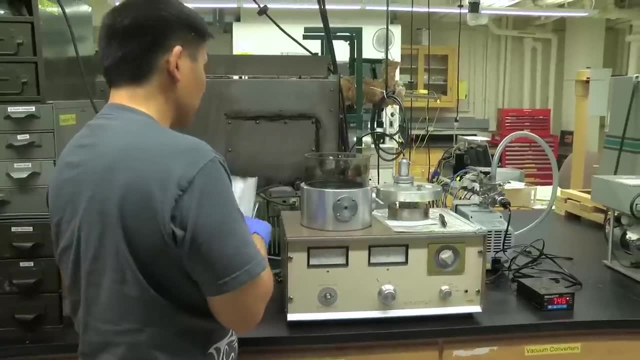 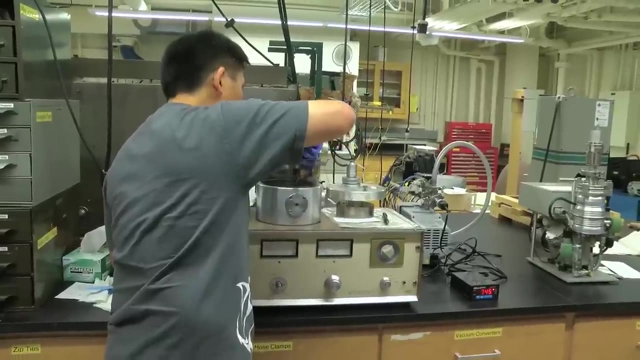 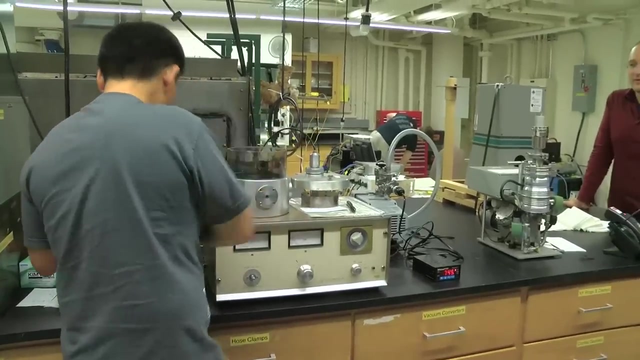 if you want for stability, Yeah. And in the chamber, the purpose of having this- actually this machine, the main reason we use this for- is if you have something that you want to put into a scanning electron microscope, and We're actually going to use one of those in the plot. 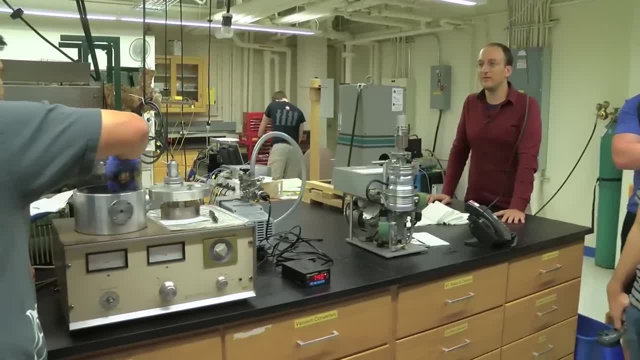 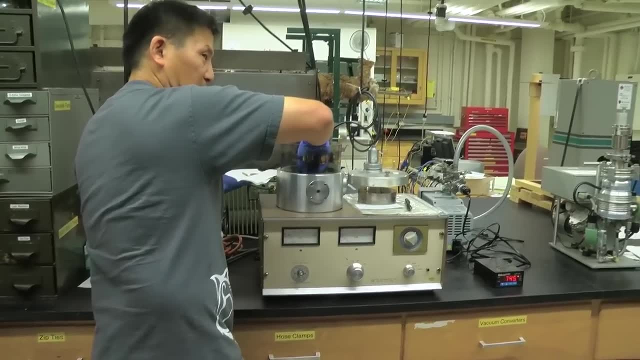 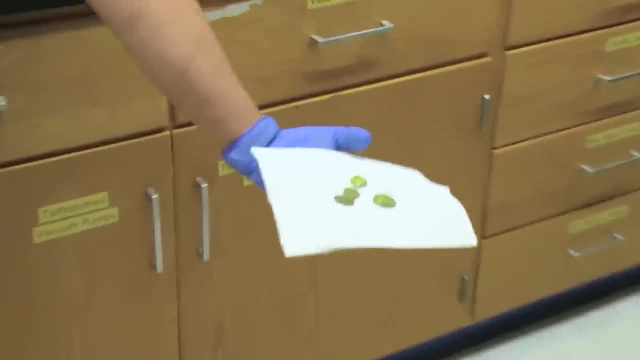 So you need to have some kind of conductive code, of conductive coating on it. So if you're looking at something like biologics, you actually coat it with something that's conductive. So there you see, that's the full coat of about. 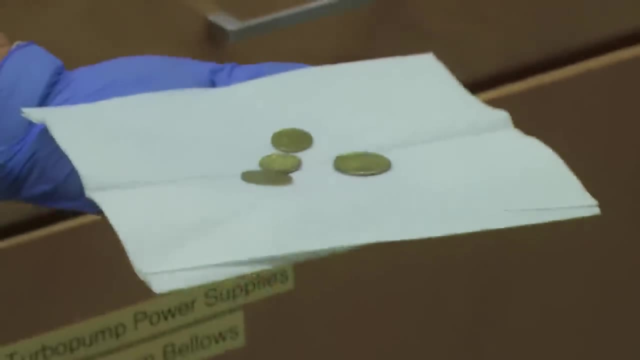 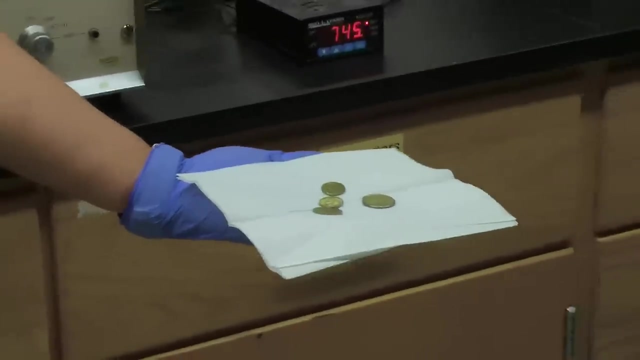 I would guess. I think for as long as we did it for something on the level of about 200 anglers. It's a pretty thin coat. That's all you need. though Remember, after quiz number one, we will be piloting, or two of you guys. 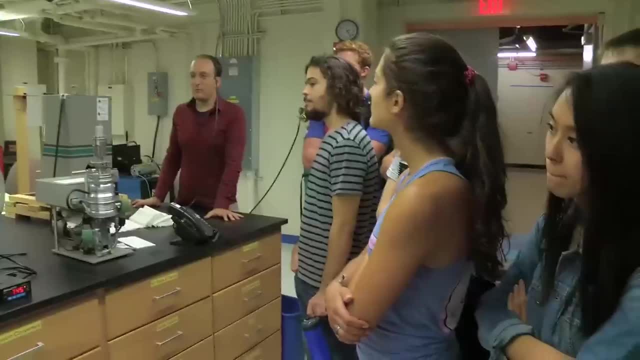 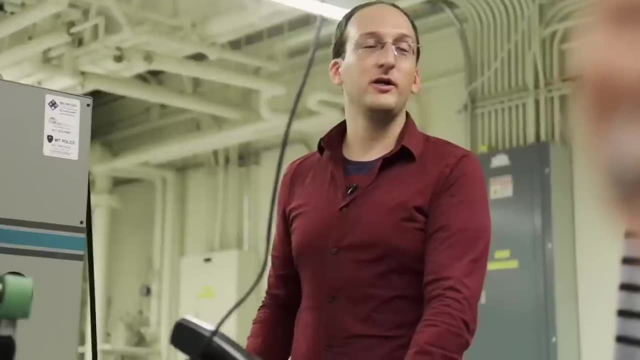 will be piloting a scanning electron microscope down in the basement And before we look at whatever samples you want to see- whether it's one of your eyelash, there's dust on the floor or a bug you found or something- we'll want to coat it in gold so that the electrons that we use 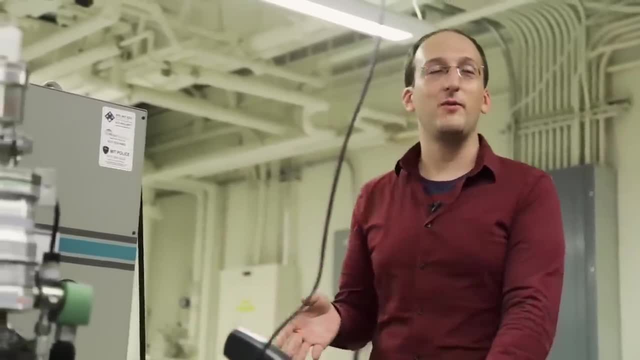 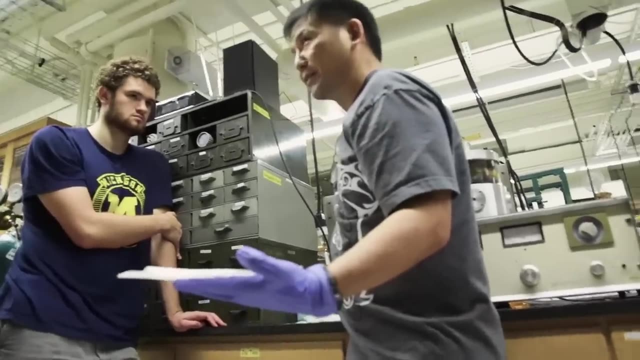 for imaging, will have a place to go, will have a conductive path and they won't charge up ruining the image. All right, I have a question. Yeah, Was anybody here born this millennium? Anyone 2000 or later? 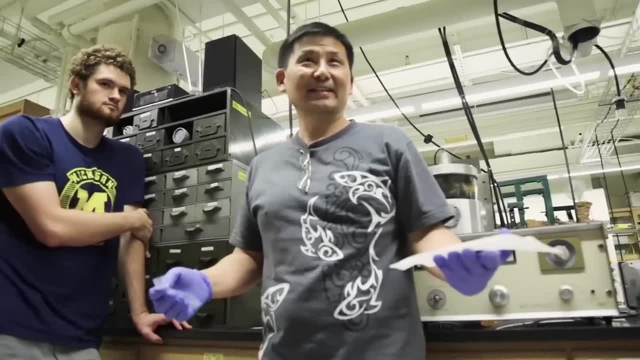 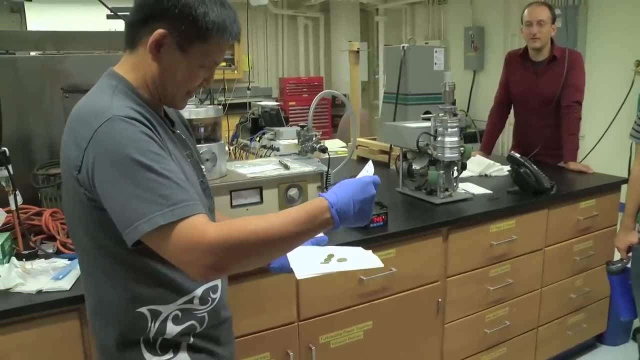 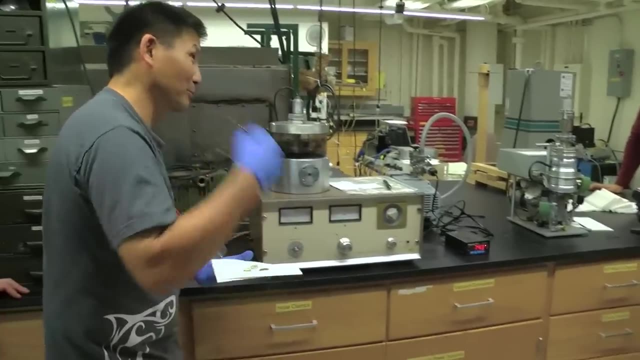 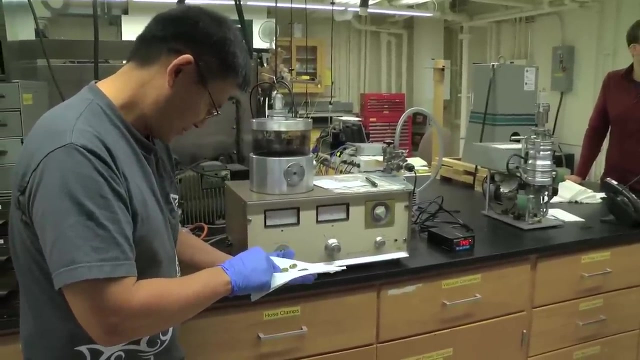 Nobody. Anyone 1999?? Nobody in 1999?? How about 98?? Anyone born in 98?? There we go. All right, That would be. I've got a 1998 dime here. It's now gold coated. 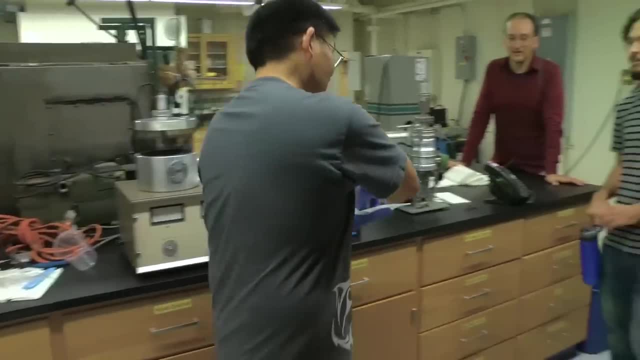 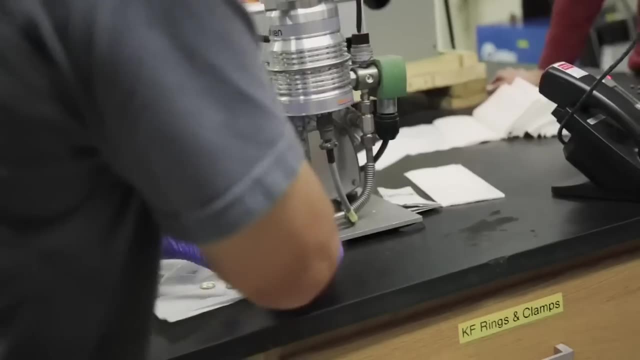 You can have it. That's right here. You bet, If somebody was born in 1999, you'd get it on the floor. You would lie and say: I guess you're the youngest one. Yeah, All right, So you win this. 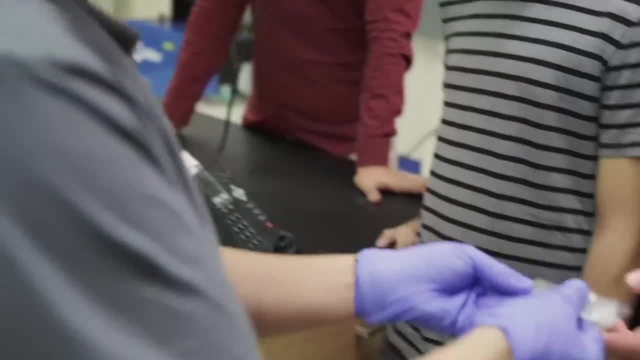 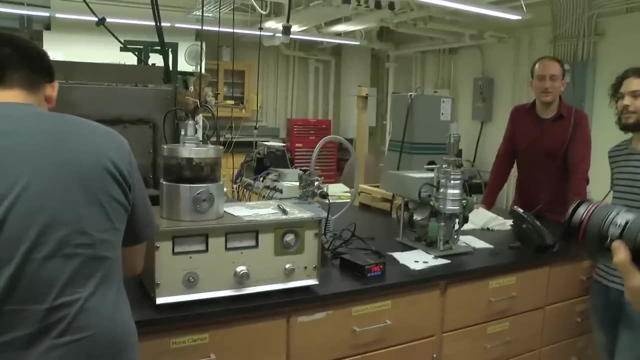 Yup, It'll rub off, OK. So thank you very much. That's why you keep it in a plastic bag, And I guess the other ones go to people that Oh no 97.. Oh no, 97.. Oh no 97.. 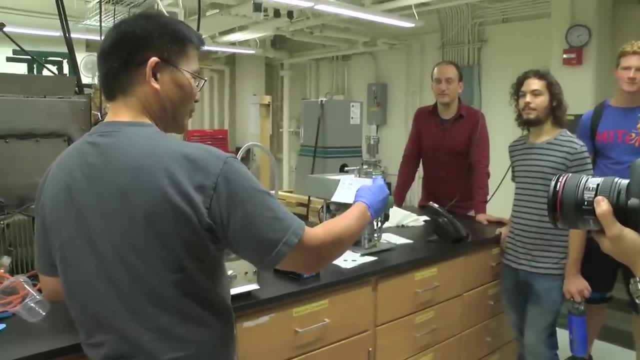 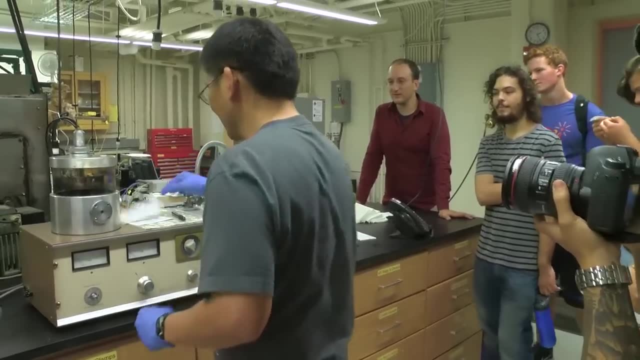 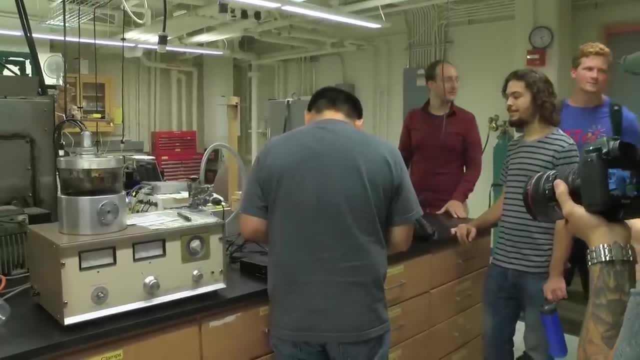 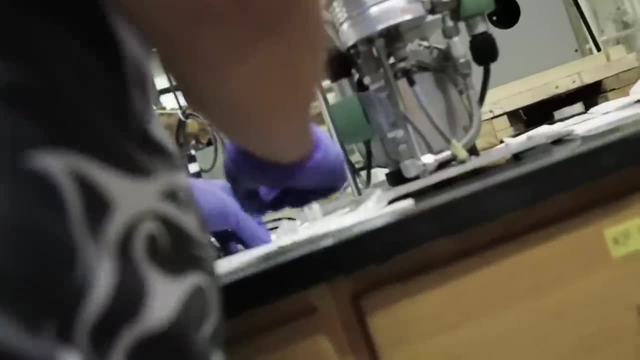 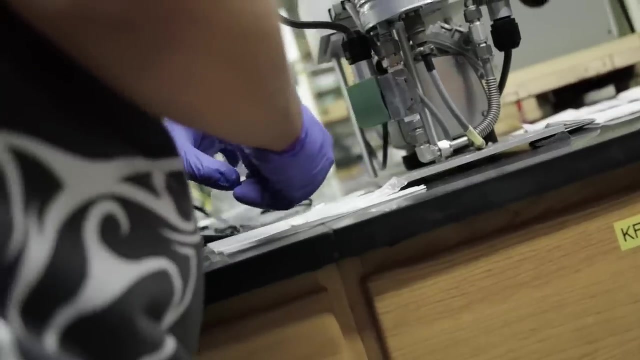 Oh, there's 3.96s. OK, You guys get this Right. Who wants the nipple? that's a 96?. You know what? There you are. There you go, Right in front of you, Reid. Well, there's three of them. OK, OK. And who have the other two knives? You're going to have to arm wrestle: One gets a cork and one gets a Arm melter. Yep, That's the only fair way of doing it. That's not a nuclear thing, but it's fun. 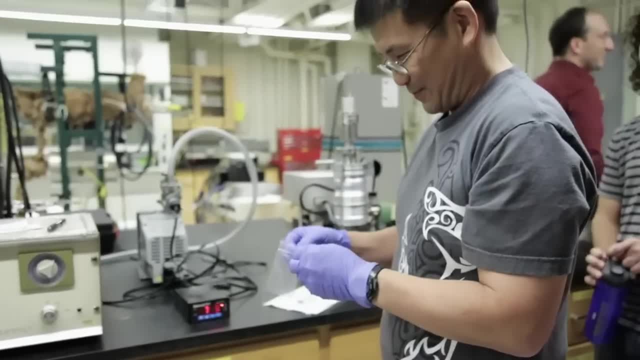 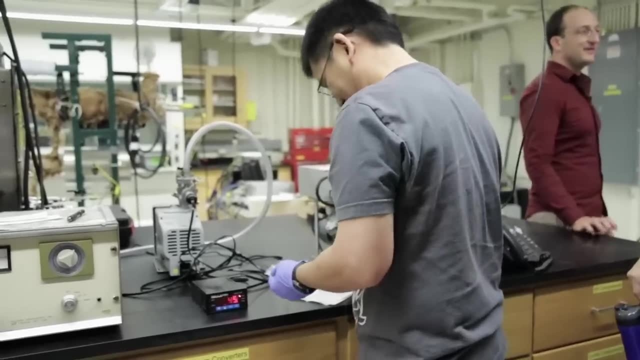 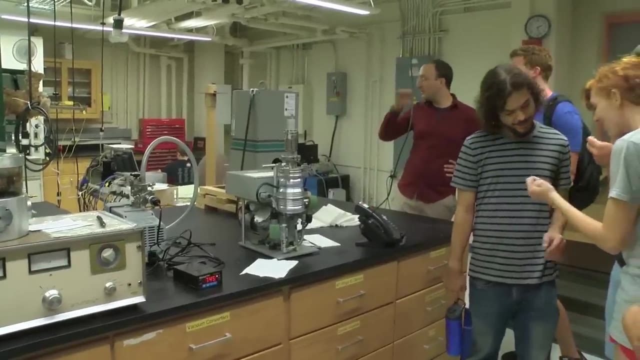 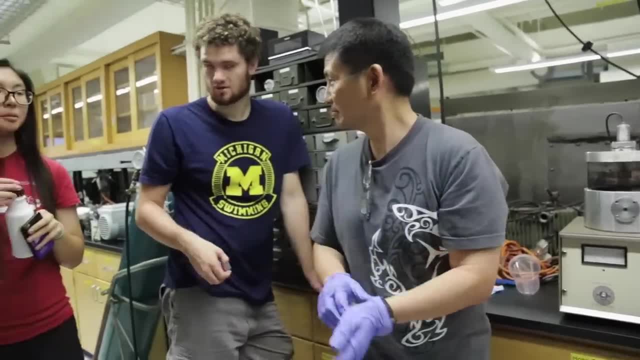 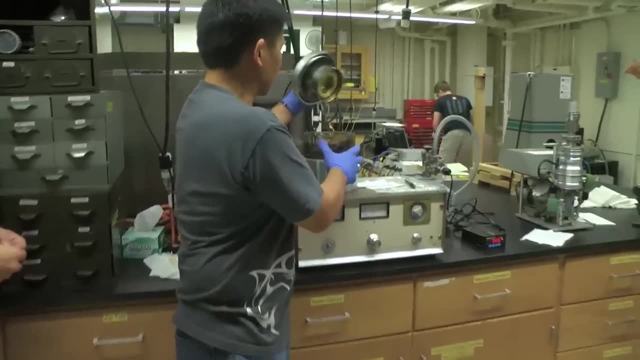 That's actually brand new insulation. It's just OK. Yeah, So is the gold deposited anywhere else in that chamber? Yeah, If you look, actually if you look in the chamber, I mean this is all from it being spluttered. 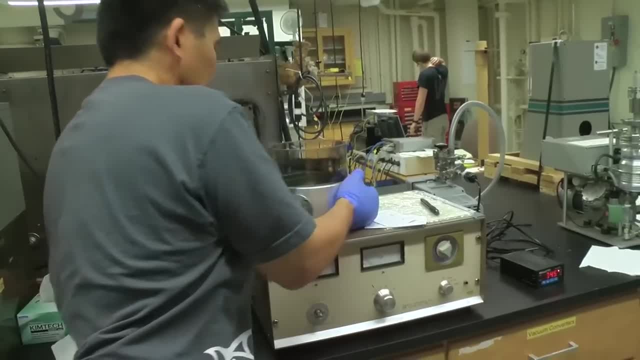 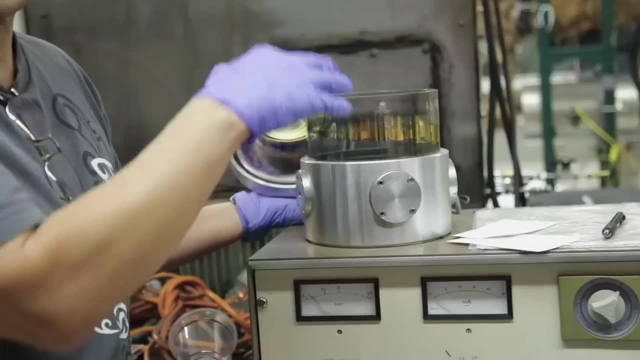 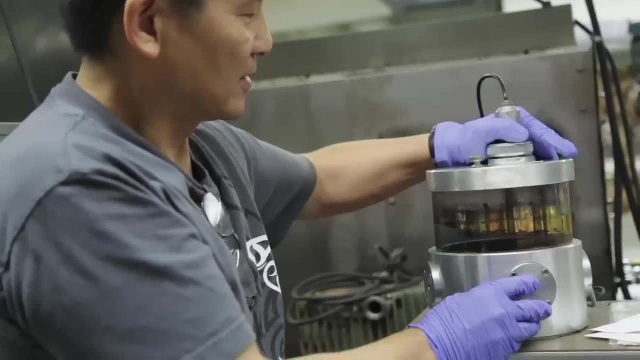 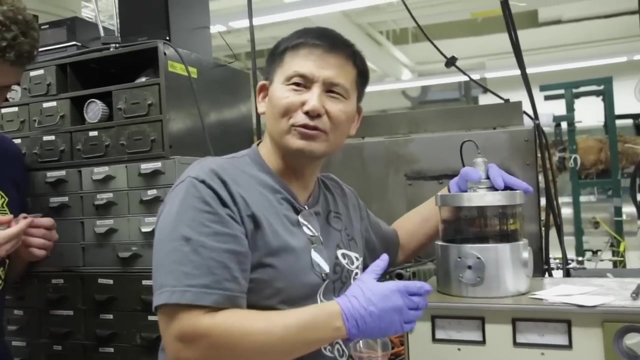 And if you look around, I can turn this and look. Look at the glass. It's a glass too Right, So it actually gets everywhere, but it's mostly directed to that area that you saw that I have another offer. are you guys all nukes? are you guys all going to be in the nuclear? 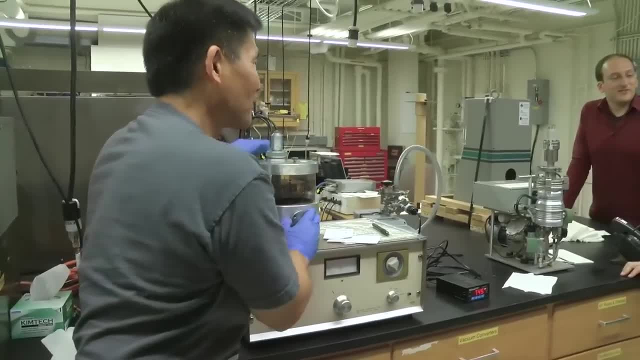 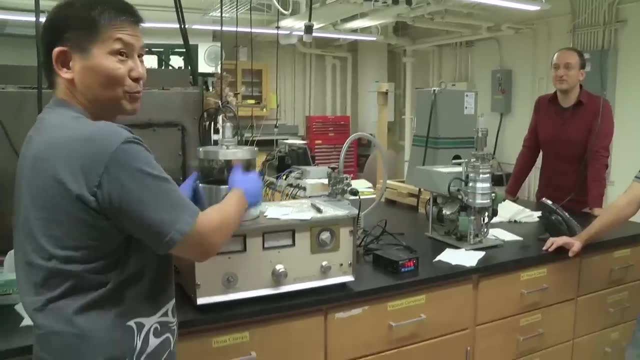 All but one, Huh. But we have a nuke enthusiast so otherwise we wouldn't be in this class, and anyone scared of nuclear is probably not in this class. So obviously it's pretty easy for us to do. we have this machine here if you're going. 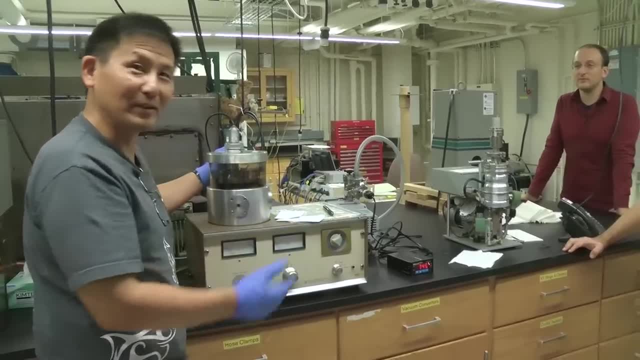 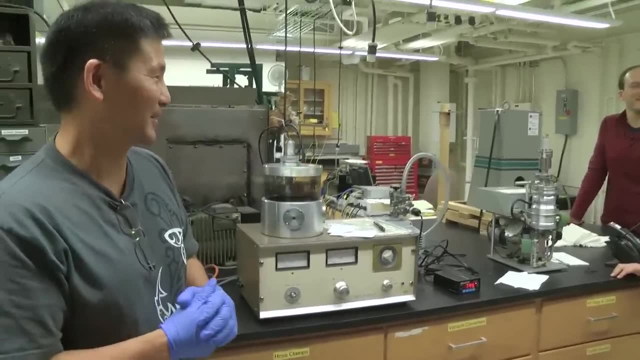 to be part of our department. if you wanted to come in, we can make you a quarter, okay. I mean I can even supply them. I feel rich enough I can do this stuff because all this graduate school money I'm getting. 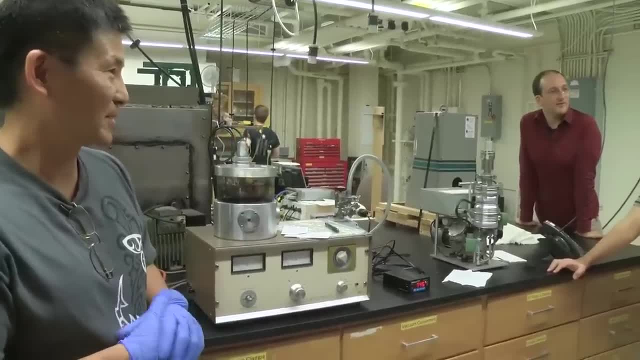 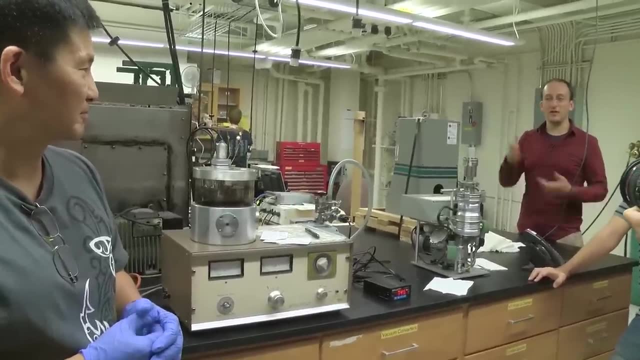 But anything else, Any questions for Reid? What you just saw, The goal is to sort of give you a real life. you know, learn 2201, you'll understand how these things work and how you can modify them, Create new stuff. that's a general idea. 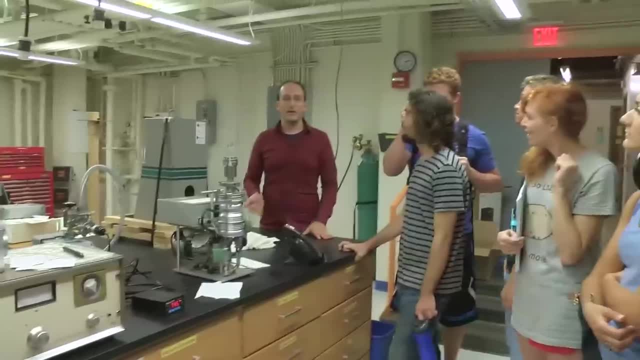 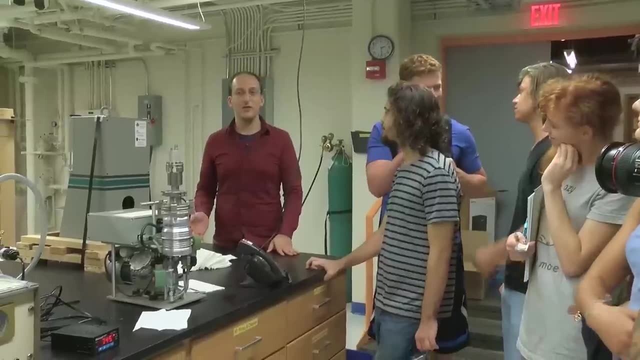 Same thing behind looking at the electron microscope, the focused ion beam, EDX, elemental analysis. I want to bring what we're teaching you to life as often as we can. Since we only got one recitation a week, we'll be doing it about that much. 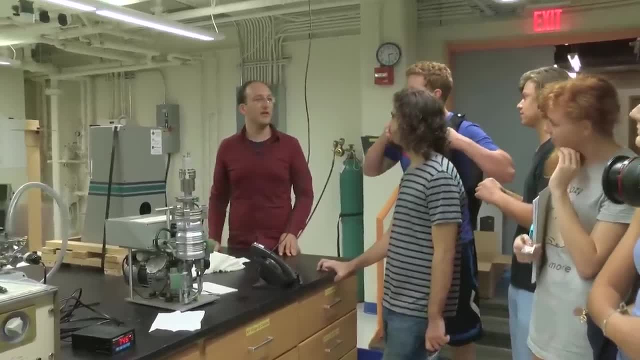 Once in a while I may schedule some extra stuff as long as folks are available, but we're going to try all we can to have days like this where you get to see what you're learning in real life. It was called a sputter. 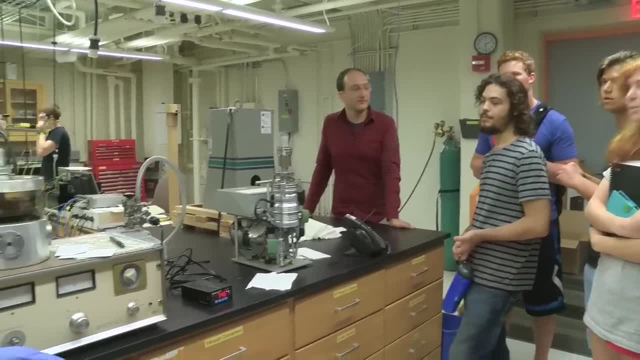 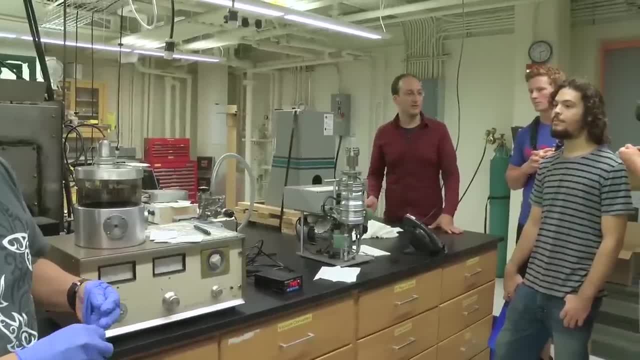 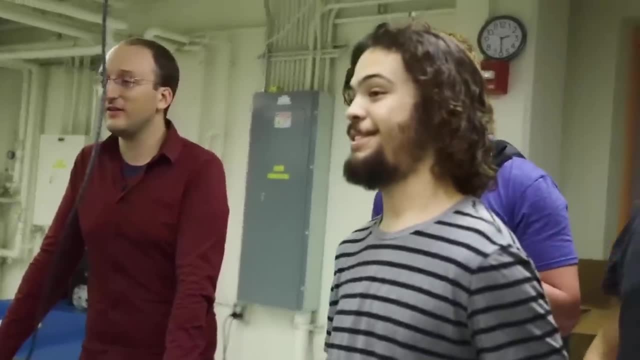 which is the blasting off of surface atoms by energetic particles. It's a controlled form of radiation damage. What's a swagalock? Swagelock, Swagelock, Swagelock, Yup. So what's a swagelock? 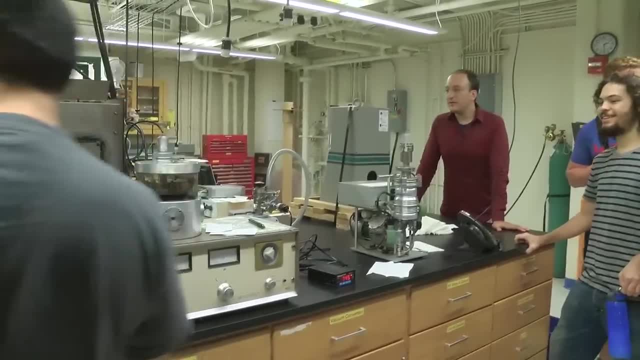 Well, Do we have any pieces here? Let's see, We have lots. actually, If you go back around Like, do you see all the tubing that you see back in there? They're connected, They don't fit, They don't fit. 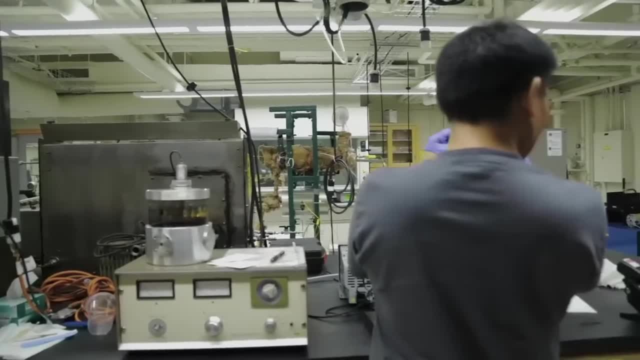 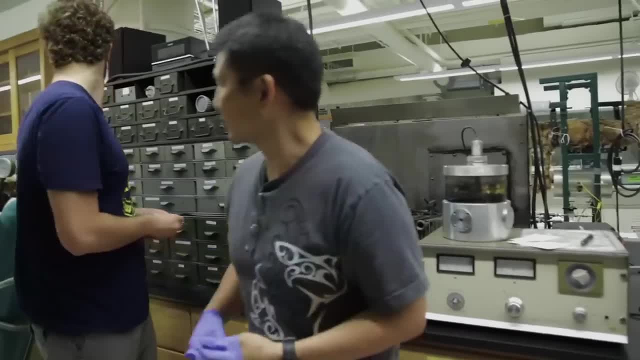 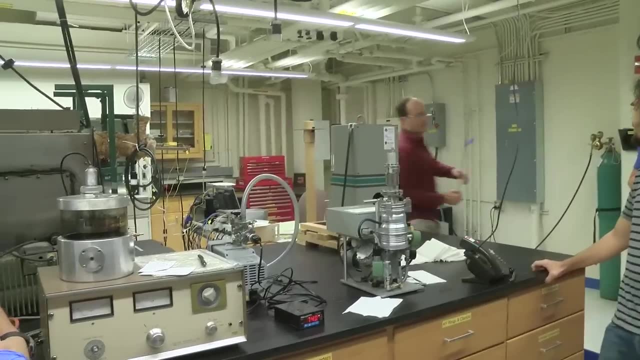 Oh, here we go. Yeah, So I don't know if Mike's going to take you around that as well. Hey, Hey look, This is swagelock tubing. It's got a two-piece ferrule which makes a metal-to-metal seal for moving liquid or 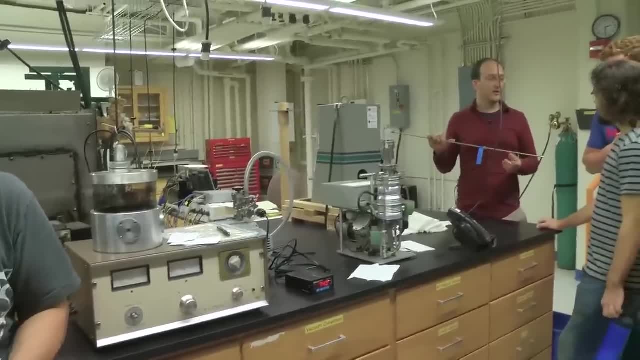 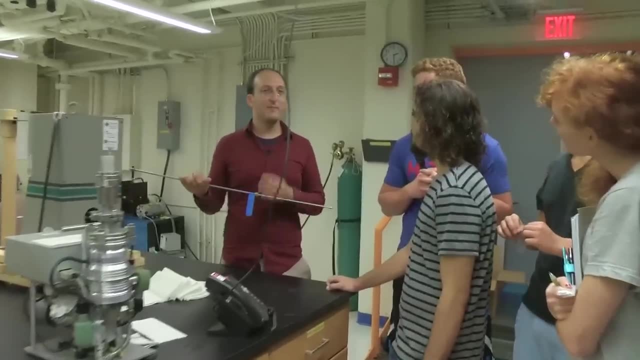 gas and it takes an insanely high pressure. So actually over in the next room we can look on our way out. We've built a reactor simulator like an experimental reactor that replicates all the conditions except for the radiation. We had to make it entirely out of swagelock tubing because this stuff can hold the pressure. 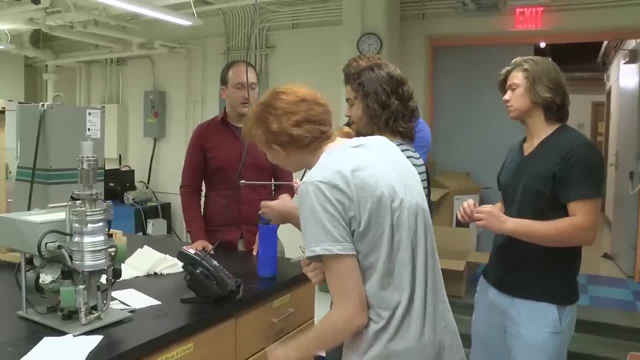 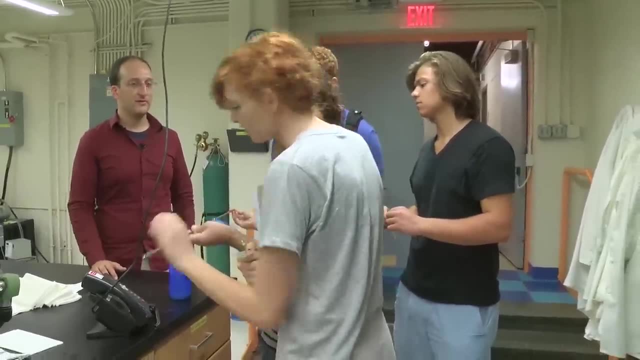 and the temperature without deforming too much. So when you want to make an absolutely airtight seal, you use swagelock or things like it. This is stainless steel. Yup, They make it out of titanium or other things too, but stainless steel works for us.